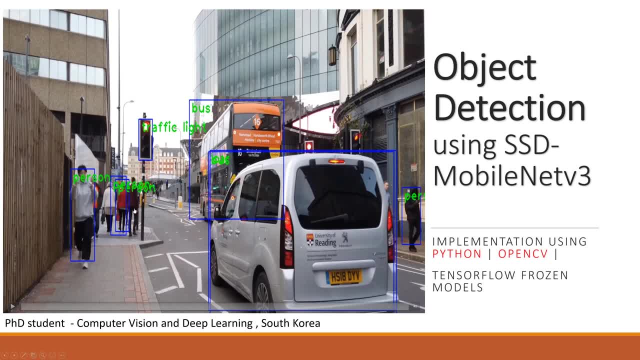 and for overlaying these rectangles and text data. we will be using opencv. Similarly, as we are targeting the beginners level students, so it's in this video. we will not train the object detection classifier. rather, we will be using pre-trained deep learning architecture based on tensorflow. 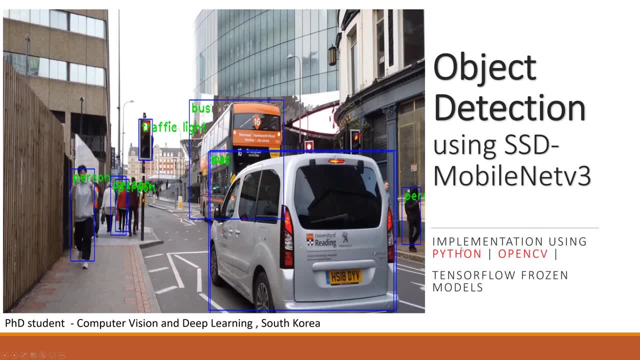 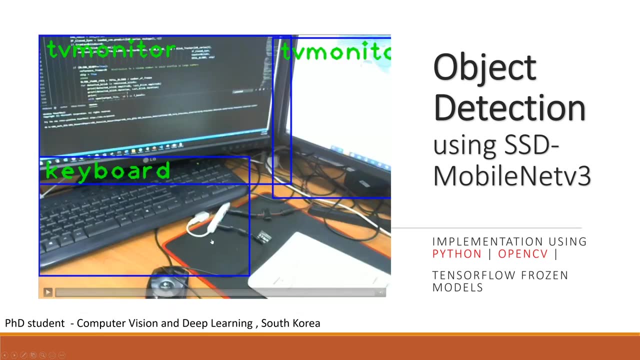 So, in this regard, we will be using opencv to load already pre-trained tensorflow frozen models. Let's get started. My name is Shanullah, I am a PhD student at Inha University, South Korea, and my major is computer vision and deep learning. At the end of this video, you will also deploy 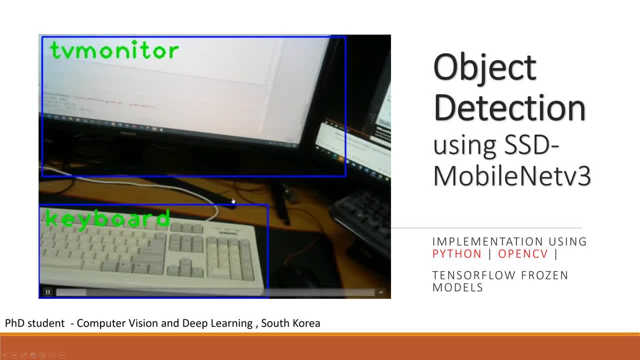 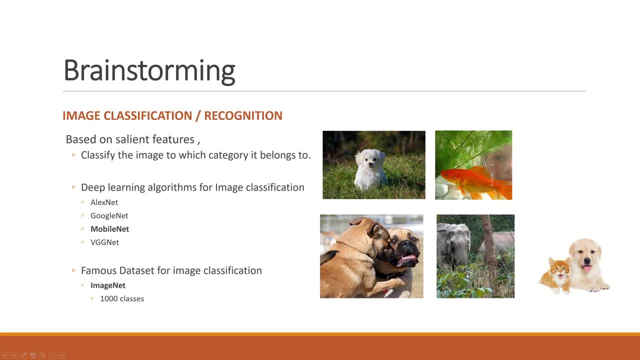 our object detection algorithm for live webcam demo. So okay, before diving into the implementation, let's have some brainstorming. As you can see over here that this: in this image we can see that there is a dog. there is a grass and background as well. But if you 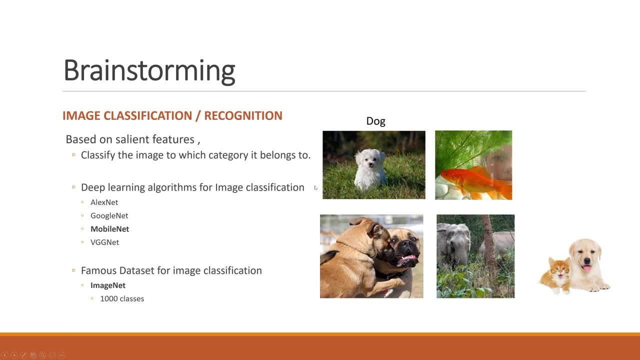 give this image to any deep learning classifier, such as AlexNet, GoogleNet, MobileNet, this will be classified as a dog Why? Because dog is the most salient feature of this image. Even a human will definitely classify this as a dog. So let's get started. 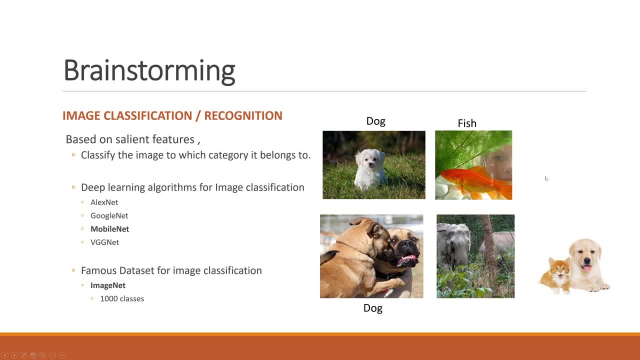 So in this image, we will classify this image as a dog. Similarly, for this image, we will classify it as a fish. right, because in this image, the most salient feature is fish. Similarly, in this regard, dog is the most salient feature and elephant is the the one which is most salient. But what about? 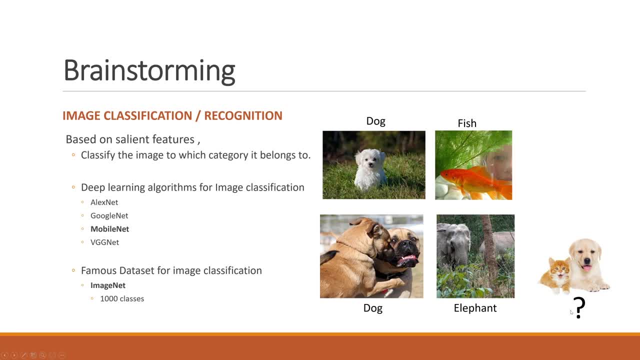 this image. it will be unfair if we classify this image as a dog or a cat, because both of them are the most salient features. so this is the problem of this video, right? so the solution to this problem is object detection, so that we can classify both of them and localize, so, for simple image. 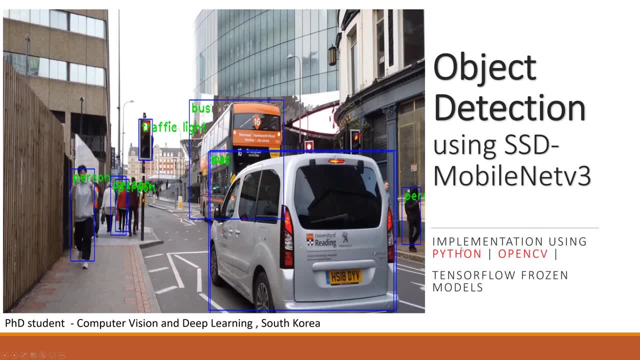 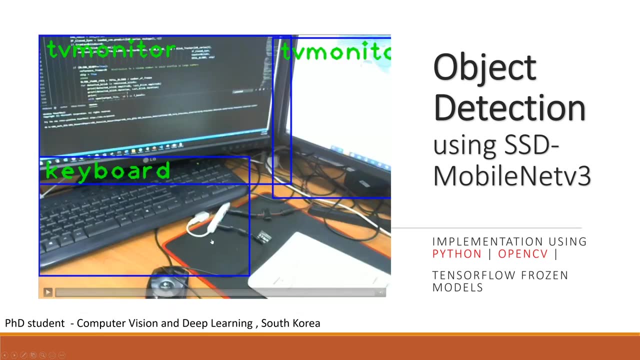 So, in this regard, we will be using opencv to load already pre-trained tensorflow frozen models. Let's get started. My name is Shanullah, I am a PhD student at Inha University, South Korea, and my major is computer vision and deep learning. At the end of this video, you will also deploy 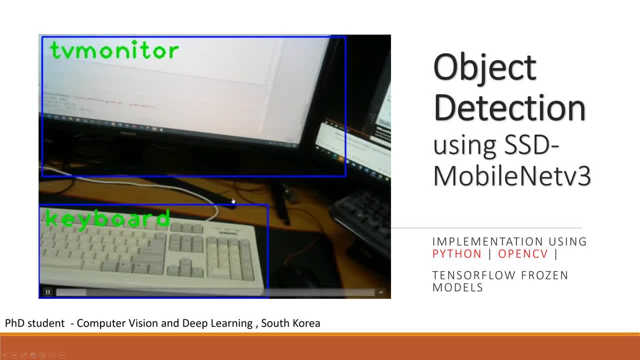 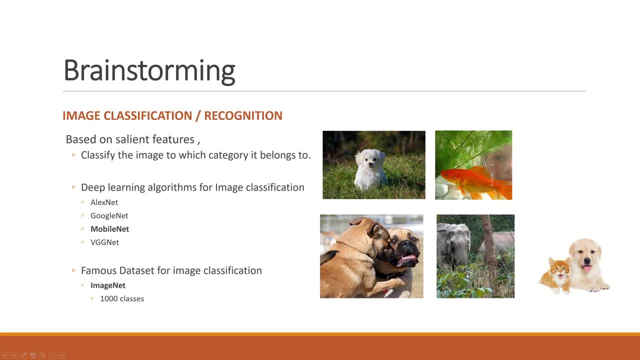 our object detection algorithm for live webcam demo. So okay, before diving into the implementation, let's have some brainstorming. As you can see over here that this: in this image we can see that there is a dog. there is a grass and background as well. But if you 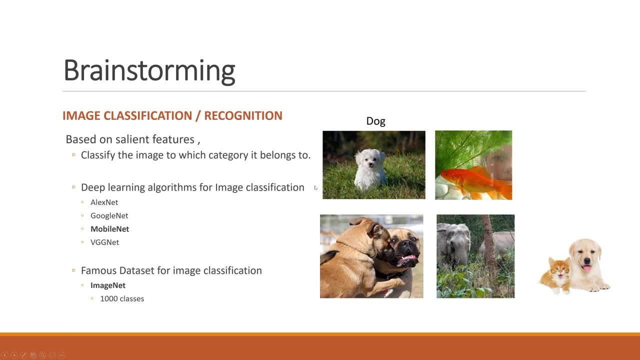 give this image to any deep learning classifier, such as AlexNet, GoogleNet, MobileNet, this will be classified as a dog Why? Because dog is the most salient feature of this image. Even a human will definitely classify this as a dog. So let's get started. 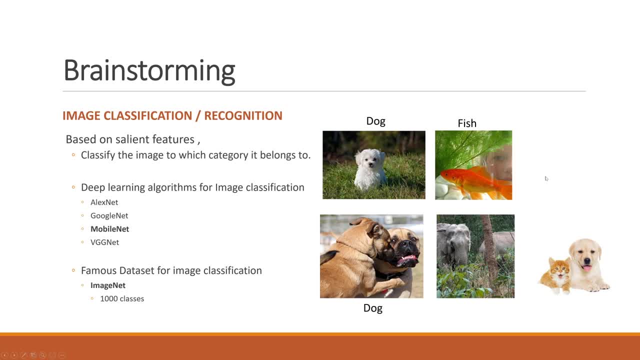 If you tap here, you will be todascaped. You just have to tap option option button To classify this image as a dog. you will specify as a dog which you can see here, as in case of animal, you will do click here and tap animal which can be classified called animal and. 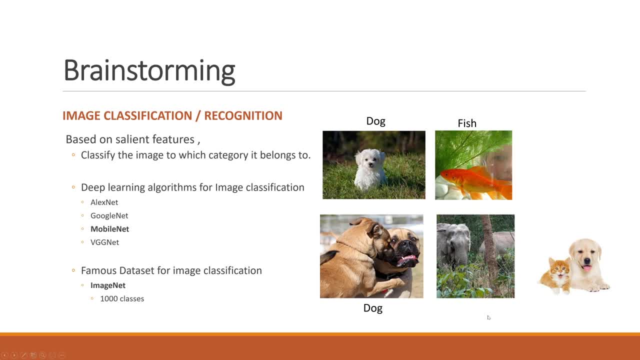 you will see the patient who is being classified had been classified as a full- близdewed dog. If you tap them, Tony will tell you that the formula is clear, where you can find your dog, is saying that this length is reached, but your dogon's length has been threshold to 234 thousand. 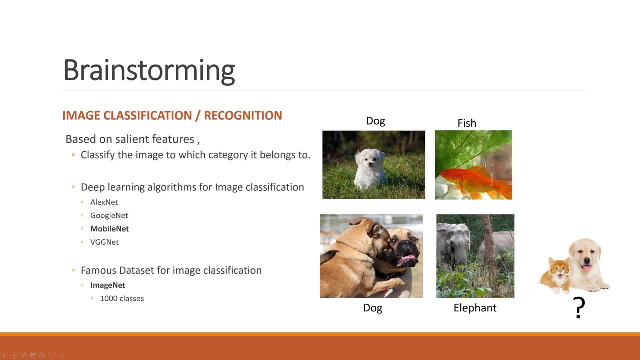 fev. Technology requires large amount of information. that's why you cannot classify things surgically- not for your cat, because both of them are the most salient features. so this is the problem of this video, right? so the solution to this problem is object detection so that we can classify both of them. 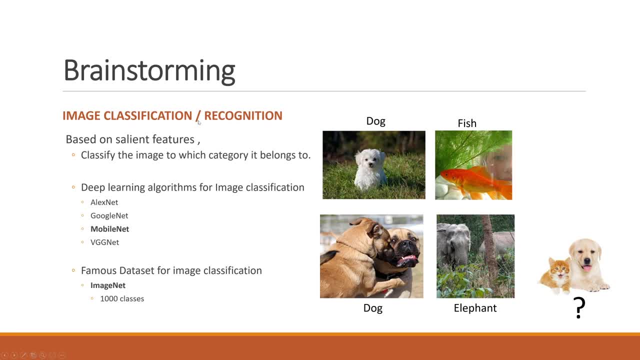 and localize, so for simple image classification and recognition. most of the classifieds are lx net, google net and all, and mobile net and vgg net, right and many others as well. so in 2012, lx net was the pioneer of the image classification challenge, which beat the human capacity by 150. 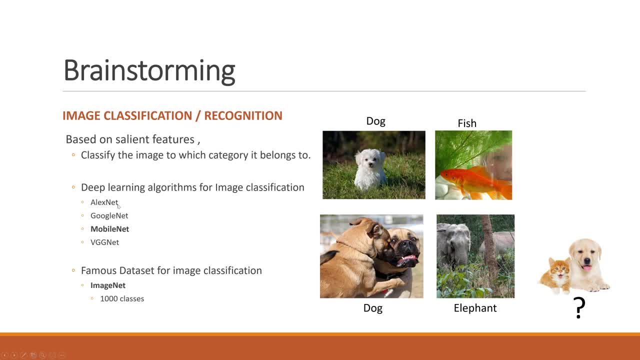 classification and recognition. most of the classifieds are lx net, google net and all, and mobile net and vgg net, right and many others as well. so in 2012, lx net was the pioneer of the image classification challenge, which beat the human capacity by 150 percent, so it was a major 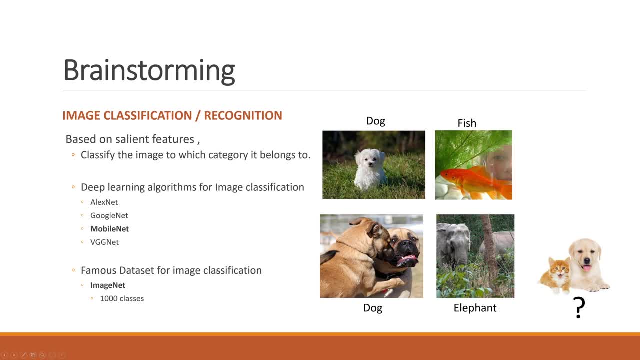 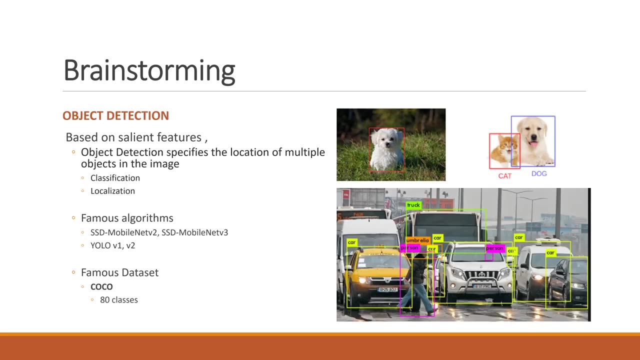 breakthrough in the deep learning. so after that many deep learning architectures are revolutionized day by day. the famous data set used for image classification is image net, which contains 1000 classes. so, however, for the object detection, the famous data set is coco having 80 classes. so, as you can, 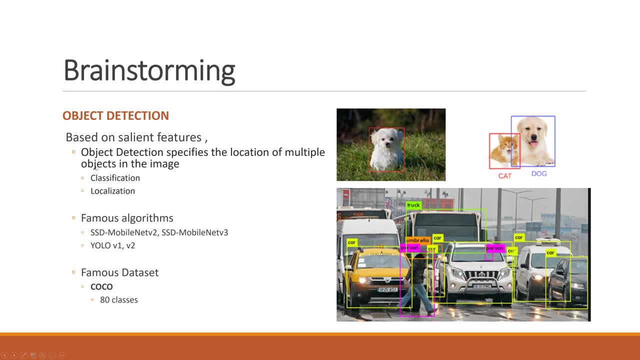 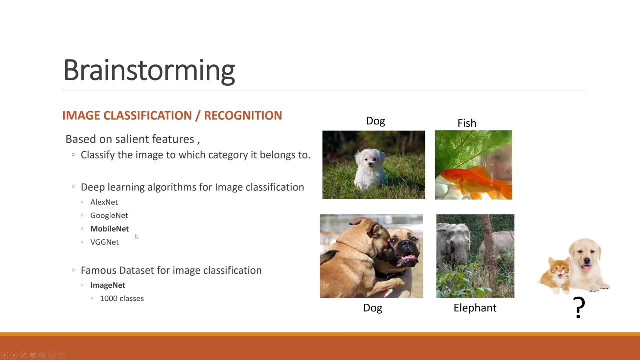 see the object detection is basically a combination of classification and localization. so, for example, in this regard we will use two the like, two algorithms, like. we will be using the combinations of two or more algorithms, right? so, for example, mobile net was the image classifier in previous we. we can see that in previous slide we 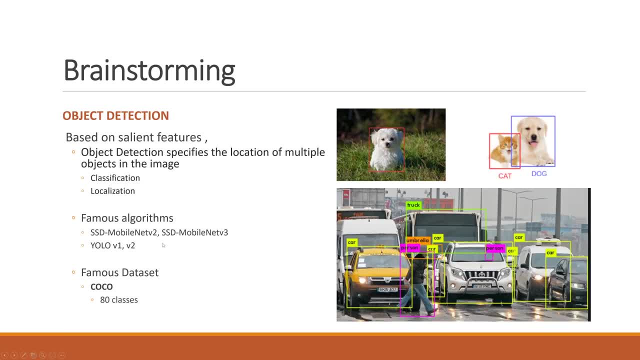 have shown that mobile net is the image classifier right. so we will use single shot multi-box detector, the combination of these two, for a better object detection. what happened in it, for example? there is image right. so what single shot multi-box detector do, right it it classify? for example, it, sorry, divides all the image into small patches and then 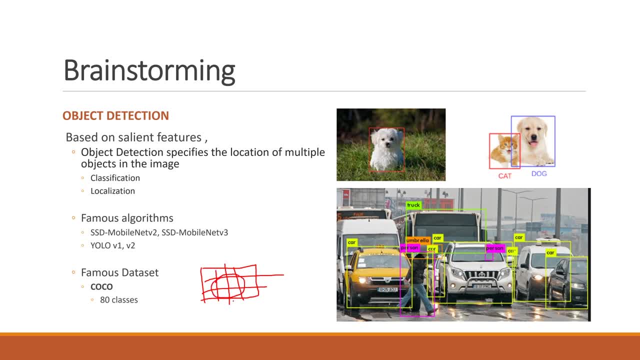 combination of the patches based on the most salient feature. it joins those patches and ask the classifier: okay, like mobile net and other, whatever is the combination. so it asks the classifier to classify this image, for example, in this case, if there is a cat and dog image. 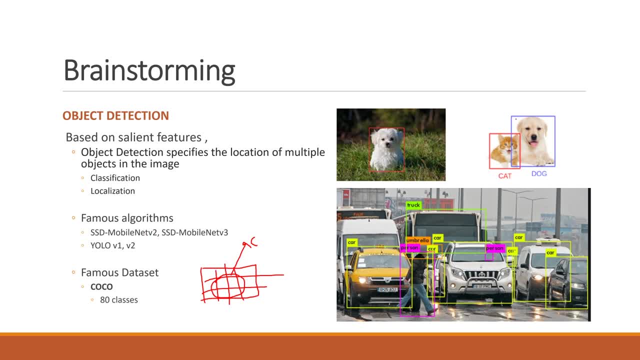 what ssd mobile net is going to do is it will ask the classifier to classify this image. and does that, it will divide into different patches and then combination of the patches it will make a most salient one, and then it will ask for from the classifier: right, so, right. so it will ask from: 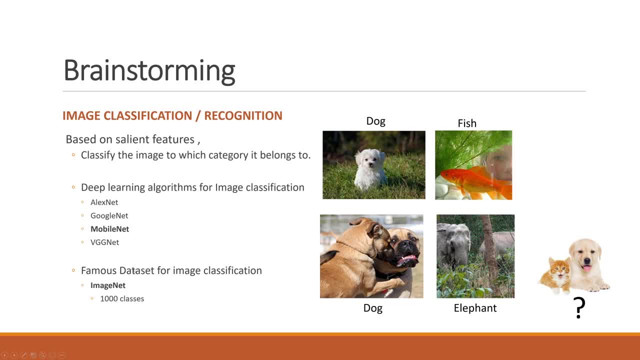 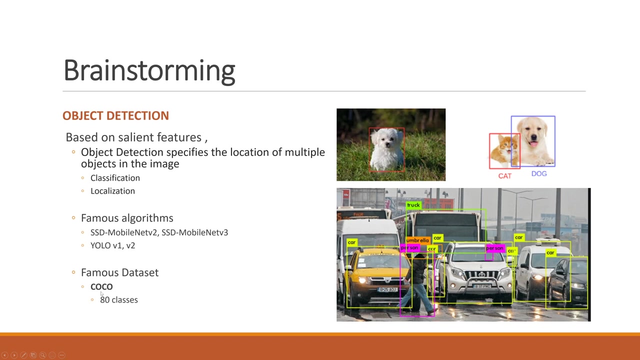 percent. so it was a major breakthrough in the deep learning. so after that, many deep learning architectures are revolutionized day by day. the famous data set used for image classification is image net, which contains 1000 classes. so, however, for the object detection, you the famous data set is coco having 80 classes. so, as you can see, the object detection is basically. 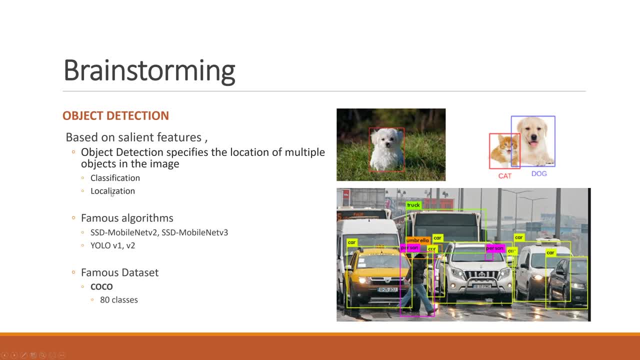 a combination of classification and localization. so, for example, in this regard, we will use two the like, two algorithms like. we will be using the combinations of two or more algorithms right. so, for example, mobile net was the image classifier in previous we. we can see that in previous slide we 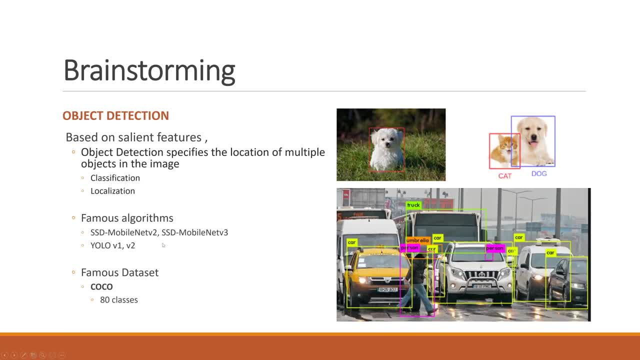 have shown that mobile net was the image classifier. in previous slide we have shown that mobile net is the image classifier right, so we will use single shot, multi-box detector, the combination of these two, for a better object detection. what happened in it, for example? there is image right, so 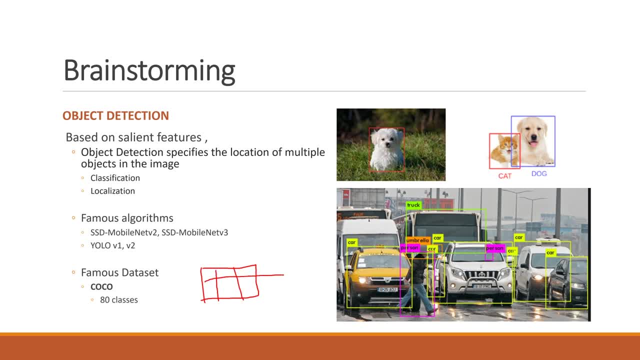 what single shot multi-box detector do? right it. it classify uh, for example. it, sorry, divides all the image into small patches and then combination of the patches based on the most salient feature- it means those uh patches- and ask the classifier: okay, like mobile net and other, whatever is the. 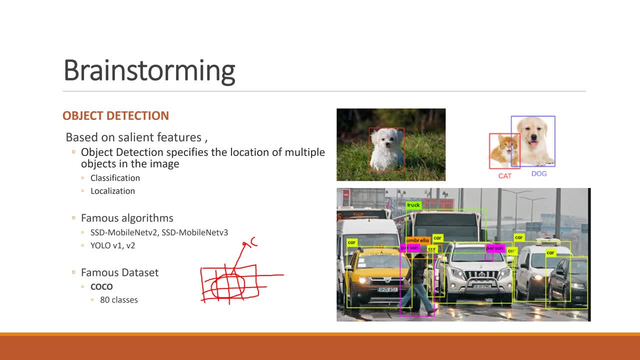 combination. so it asks the classifier to classify this image. for example, in this case, if there is a cat and dog image, what ssd mobile net does? that it will divide into different patches and then combination of the patches it will make a most salient one and then it will ask for from the 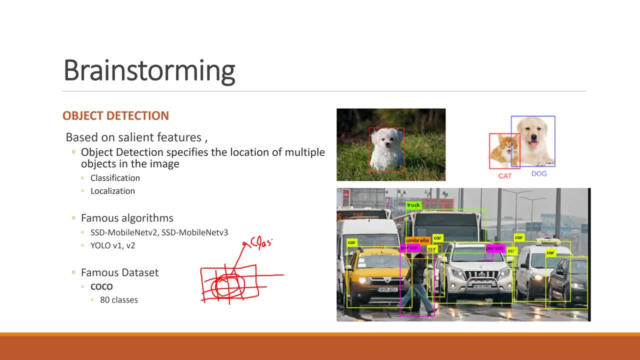 classifier. right, so right. so it will ask from the classified. so it is the combination of two algorithms. similarly, we do have other algorithms, like yolo- you look only once- which is also a very famous one, but the most lightweight and faster one is ssd mobile net and, in this regard, the most recent one is ssd mobile net. 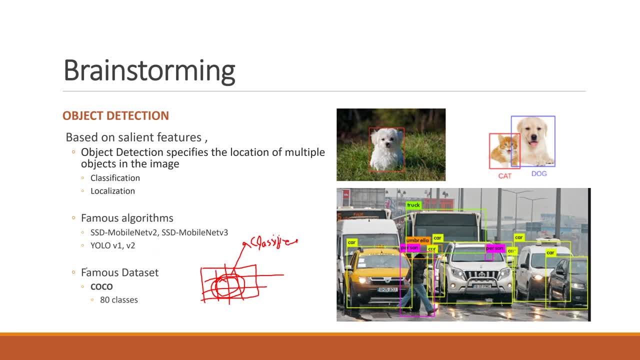 the classified. so it is the combination of two algorithms. similarly, we do have other algorithms, like yolo- you look only once- which is also a very famous one, but the most lightweight and faster one is ssd mobile net and, in this regard, the most recent one is ssd mobile net version three, which is among all like version. 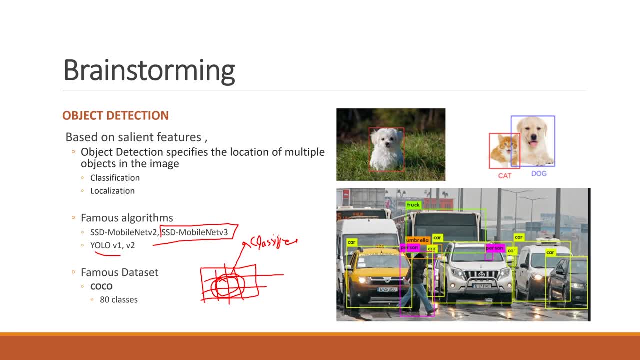 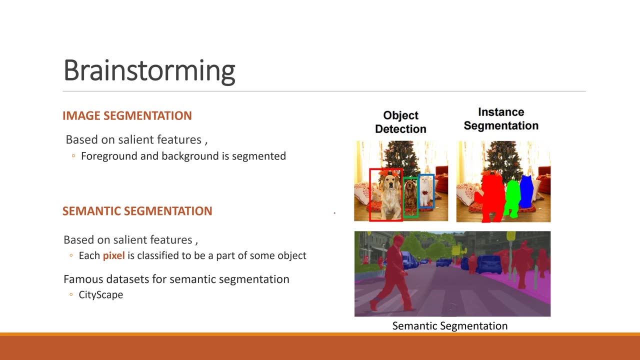 one, version two and version three is the best one right. so now we have defined the problem that what is object detection? now let's dive into implementation. but before diving into implementation, one another very important concept is image segmentation. so these are the three important concepts, like image classification, object detection and then image segmentation. 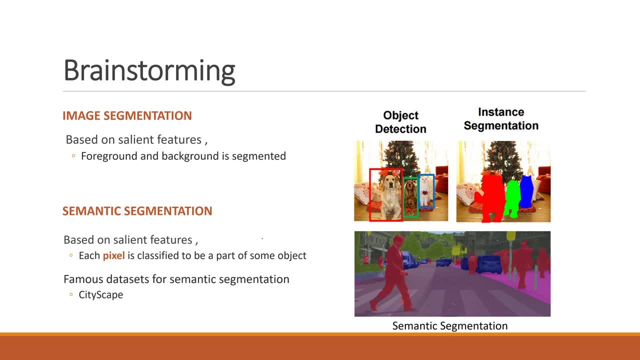 so what is image segmentation? so image segmentation is to classify, rather than classifying an object, it is to classify each pixel. over here you can see that, for example, this man, this is a person, right, so every pixel has been classified, right, it it shows like red. so all the. 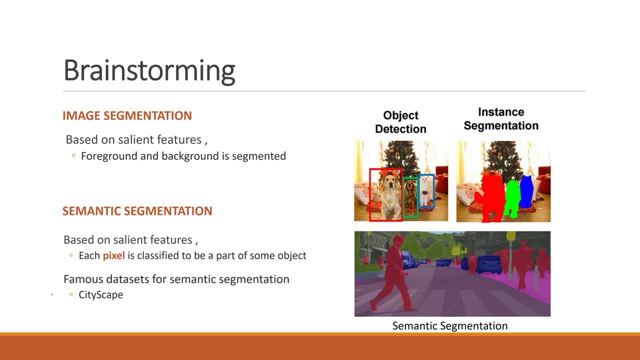 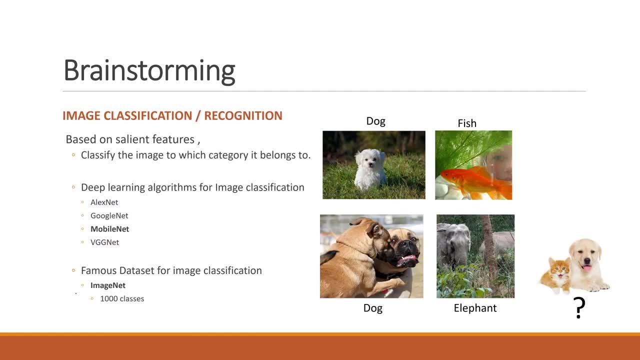 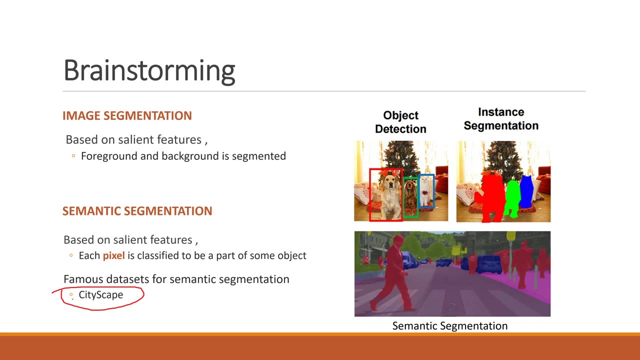 persons in this video is shown to be red. similarly, the data set is different, like cityscape. previously, for the object detection the famous data set is coco and for image classification it is image now. so definitely we need to care about the data set as well, but in this video we are. 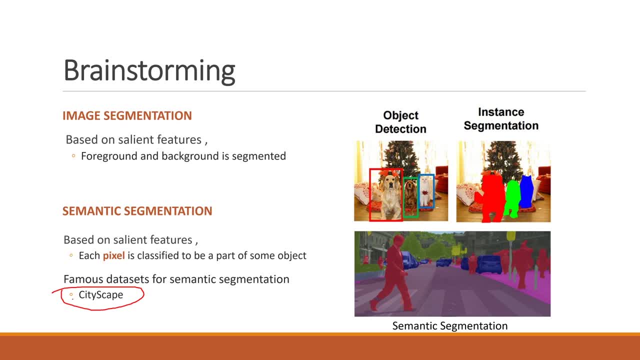 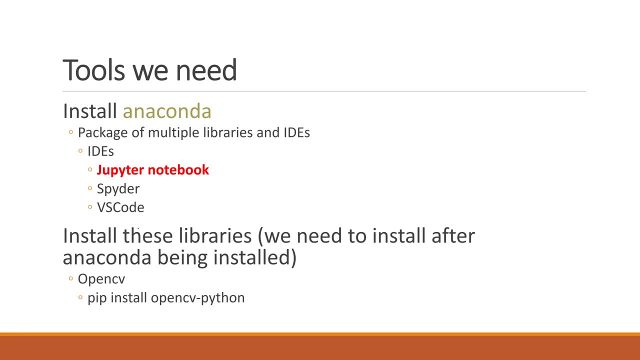 targeting only the concepts and just the implementation. so let's dive into the implementation. the ingredients we will be using in this video is, for example, anaconda, which is the package containing different ids. id is the one in which we program our code right, so we do have spider. we. 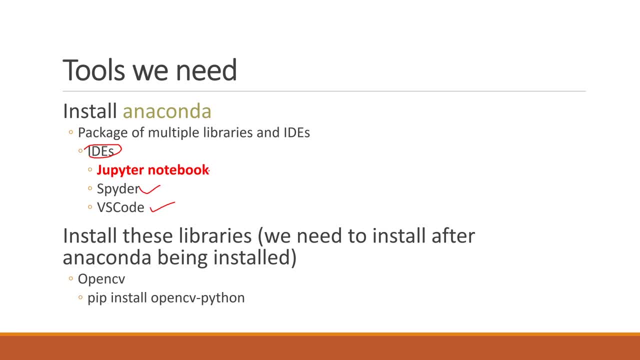 have vs code and jupyter notebook. but we found the jupyter notebook the best candidate for this tutorial. why? because we can make nodes and a lot of other features we do have in the jupyter notebook. you will see in this video, after installing anaconda and jupyter notebook at the end of this video- sorry, I mean after installing these two- we will 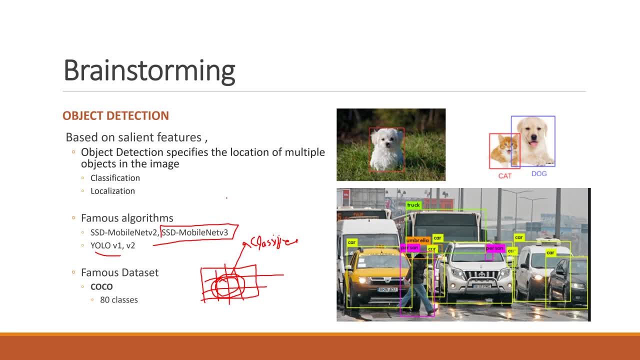 version 3, which is, uh, among all, like version 1, version 2 and version 3, is the best one, right. so now we have defined the problem, and we have defined the problem, and we have defined the problem, that what is object detection? now let's dive into implementation. but before diving into, 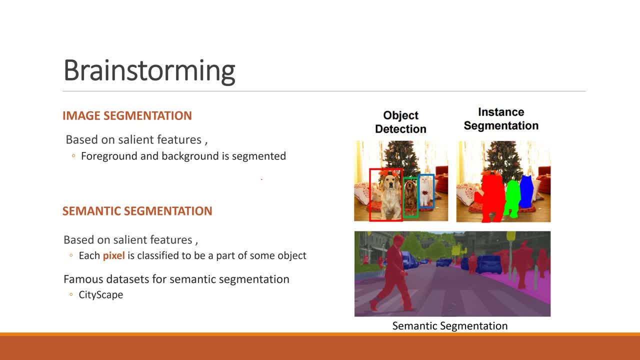 implementation. one another very important concept is image segmentation. so these are the three important concept, like image classification, object detection and then image segmentation. so what is image segmentation? so image segmentation is to classify, rather than classifying an object, it is to classify each pixel over here you can see that, for example, this man, this is a person, right. so 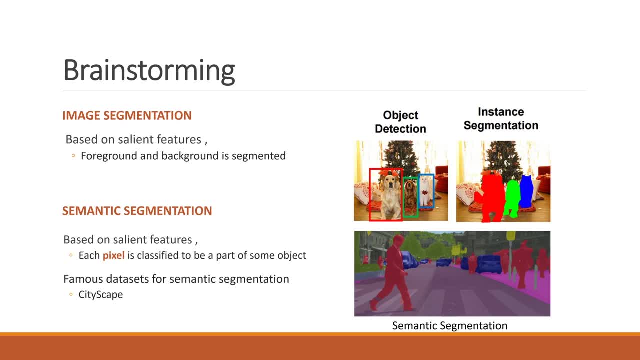 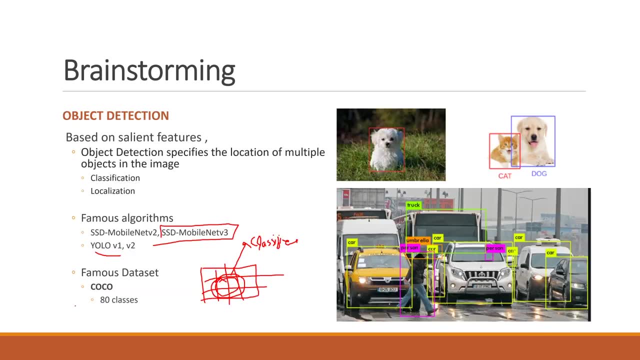 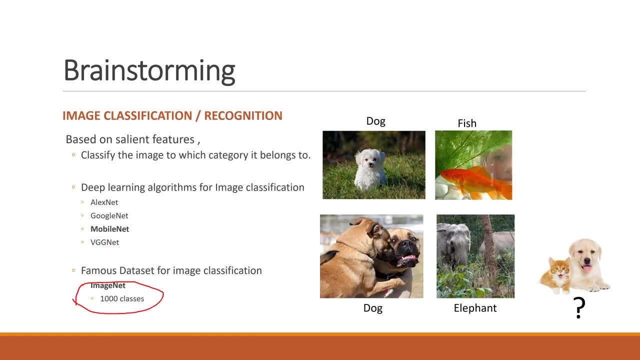 pixel has been classified right it it shows like red, so all the persons in this video is shown to be red. similarly, the data set is different, like cityscape previously. for the object detection the famous data set is coco and for image classification it is image net. so definitely. 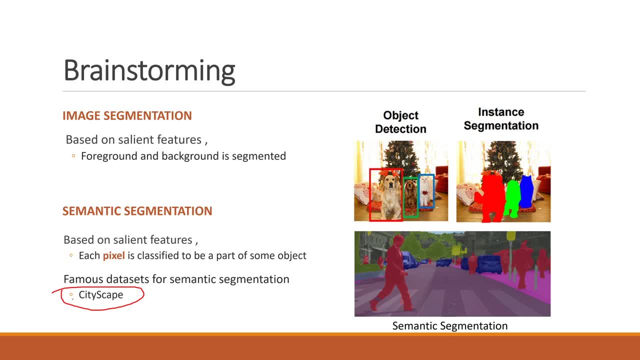 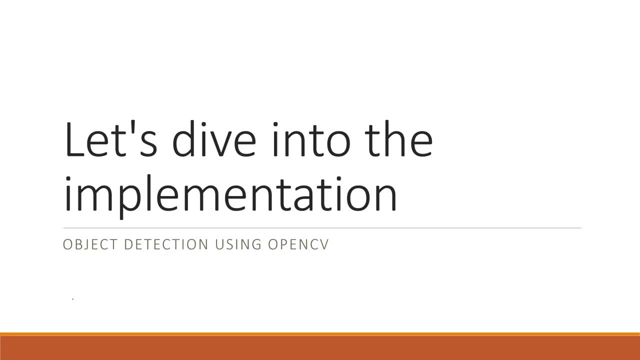 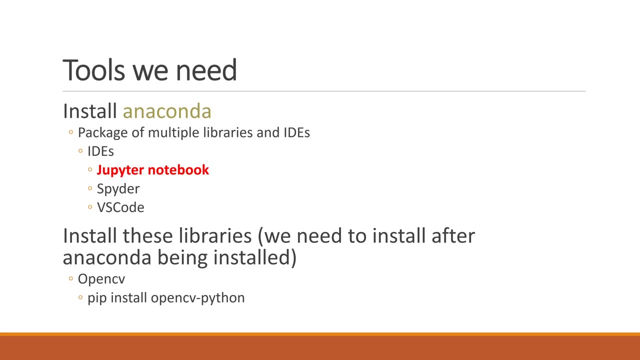 we need to care about the data set as well, but in this video, we are targeting only the concepts and just the implementation. so let's dive into the implementation. the ingredients we will be using in this video is, for example, anaconda, which is the package containing different IDs. ID is the one in which we program our code right, so we 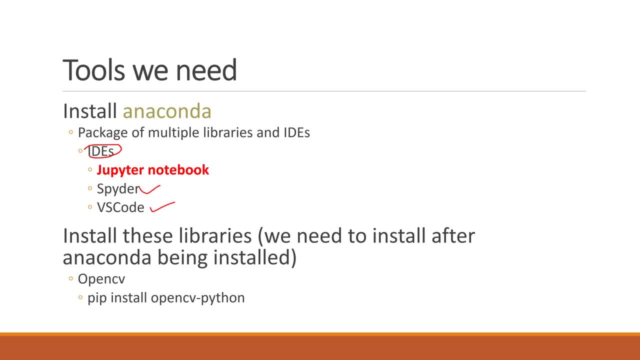 do have spider. we have vs code and Jupyter notebook, but we found the Jupyter notebook the best candidate for this tutorial. why? because we can make notes and a lot of other features we do have in the Jupyter notebook. you will see in this video after installing anaconda and 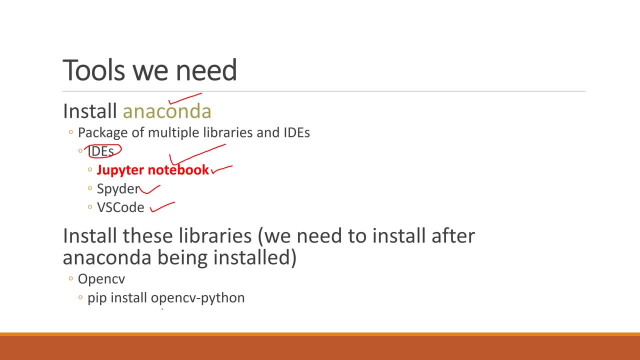 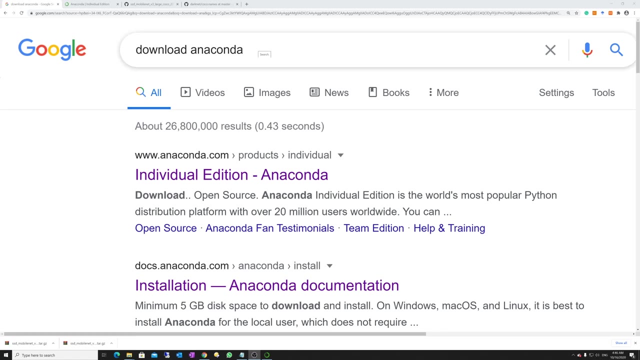 Jupyter notebook at the end of this video. sorry, I mean after installing these two, we will install OpenCV. let's get started for the implementation. in order to install anaconda, all you need is to just write in this Google search bar download anaconda and once you write it, you will find the first link, if you. 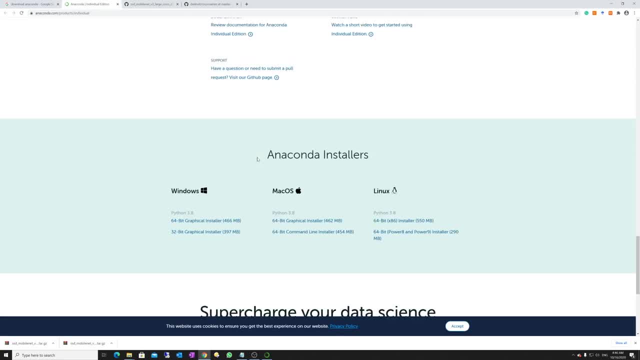 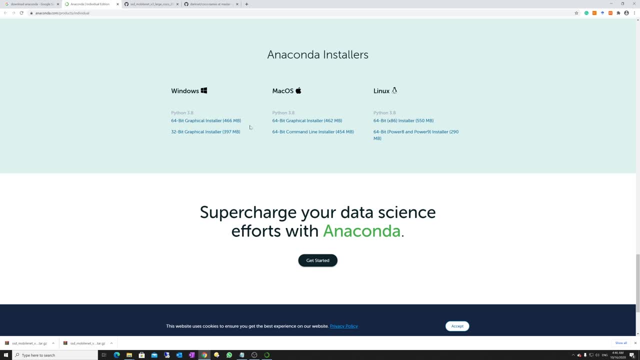 could click the first link. you will find at the downside of this link and many executables also based on your specifications. either you are using anaconda or Jupyter, you can just download the corresponding executable right. once you download, all you need is to just press next, next, next and it is. 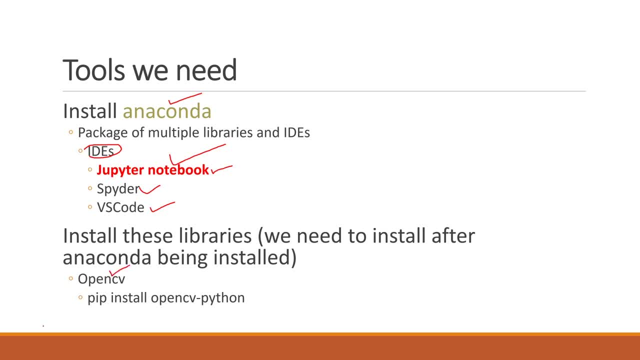 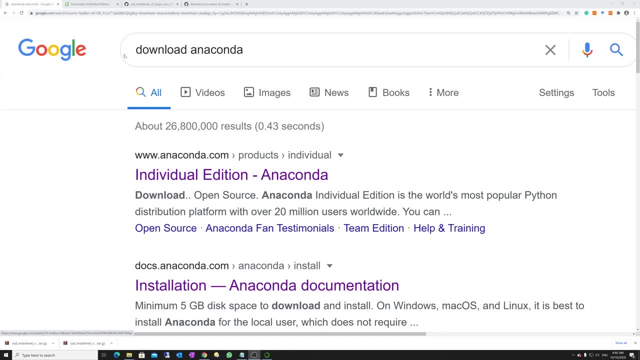 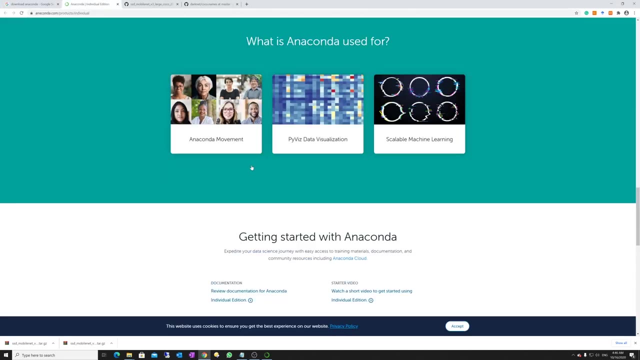 install opencv. let's get started for the implementation. in order to install anaconda, all you need is to just write in this Google search bar download anaconda, and once you write it, you will find the first link. if you click the first link, you will find and the downside of this link and many executables, so based on your specifications. 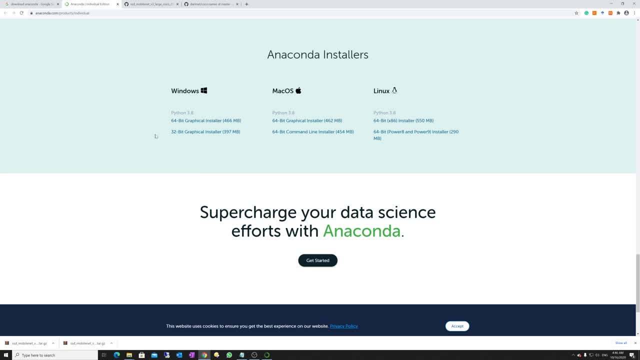 either you are using Windows, macOS and Linux, you can just download the corresponding executable right. once you download, all you need is to just press next, next, next, and it is super simple to install. now I assume that you have already installed the anaconda, so in the Windows search bar, if you. 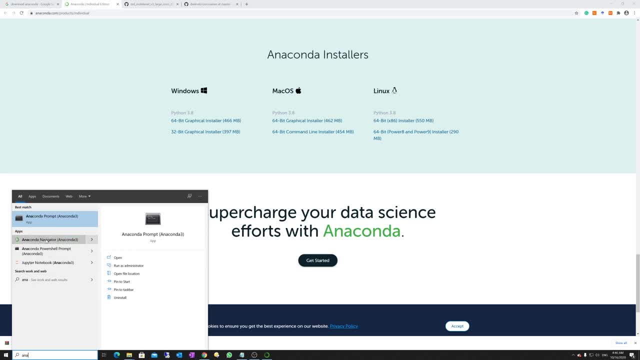 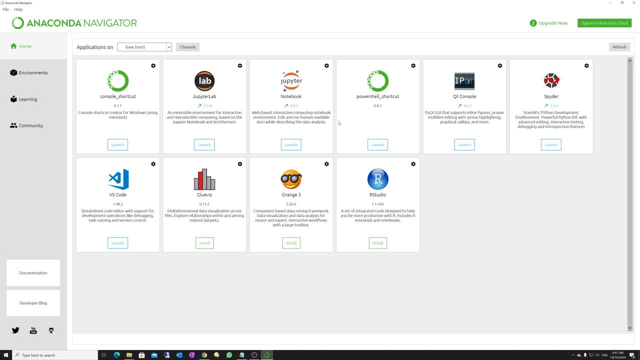 the anaconda like this, so you will reach here like anaconda navigator. if you press the anaconda navigator, you will reach to this page. over here you can observe that we have green buttons with install instruction and blue buttons to launch, right, so in your case, as you install the navigator, so all of them. 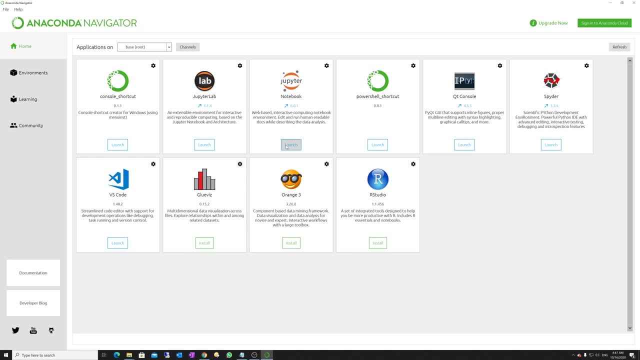 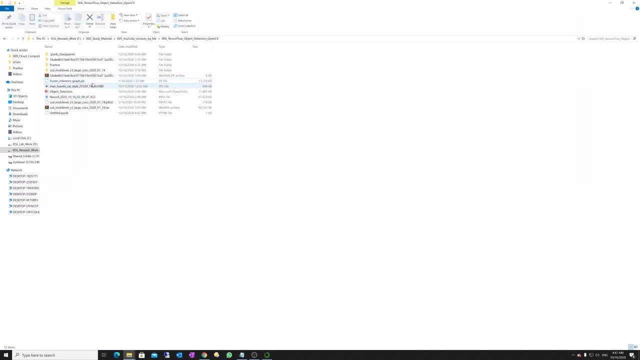 will be green and you can just click the install button of the jupyter notebook. now I assume that you have installed an anaconda navigator and jupyter notebook. once you install the both of them, it's better to create a new folder, right? so in my case it's full, but in your case the folder will be empty, right? so create. 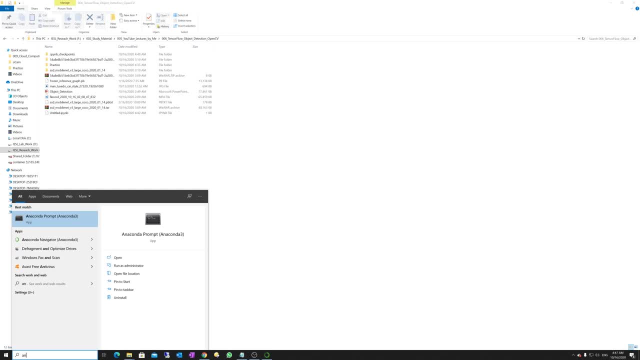 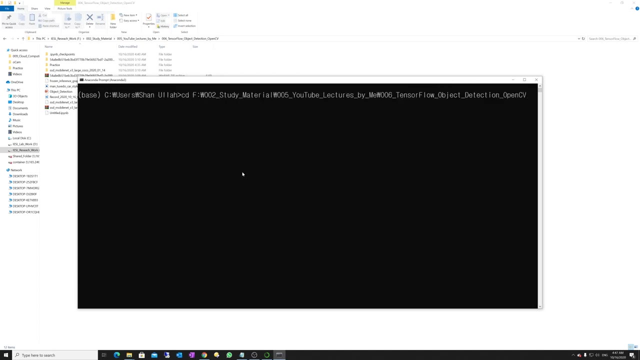 an empty folder for your project. then then again, you should write an anaconda, and this time, rather than clicking an anaconda navigator, you should press the anaconda prompt right. so once you click this, let me zoom for you. all you need is your CD and paste the path, and then change the. 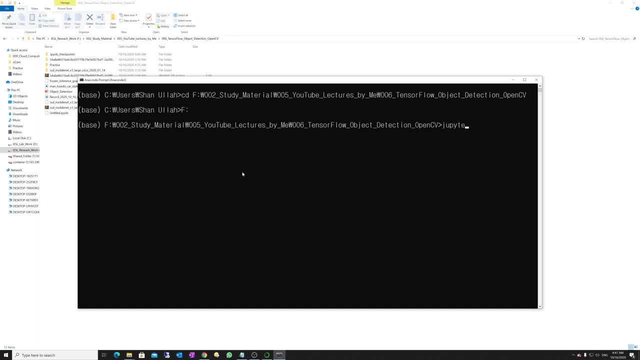 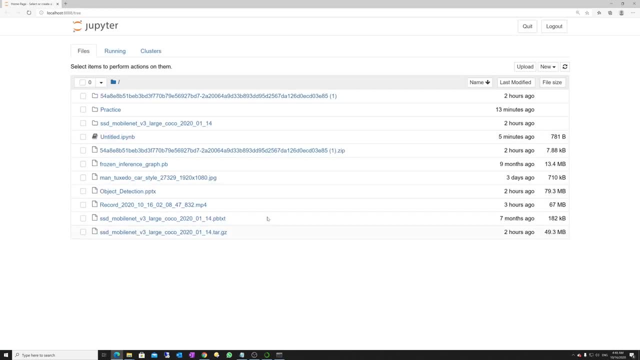 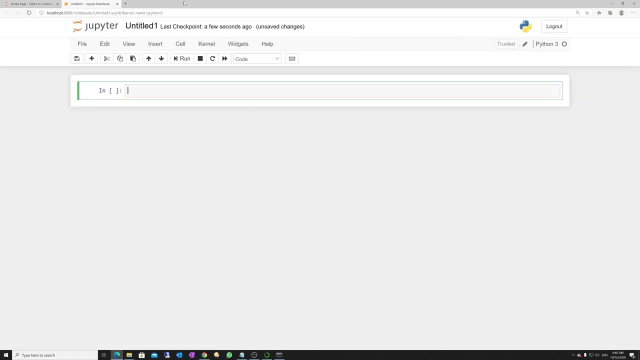 drive and just write jupyter notebook. once you write a jupyter notebook, okay, so a window will be appear like this: right, so all you need is you just create a new Python jupyter notebook and let me separate for you guys. okay, you don't need to do this to install an anaconda navigator, but you don't need to. 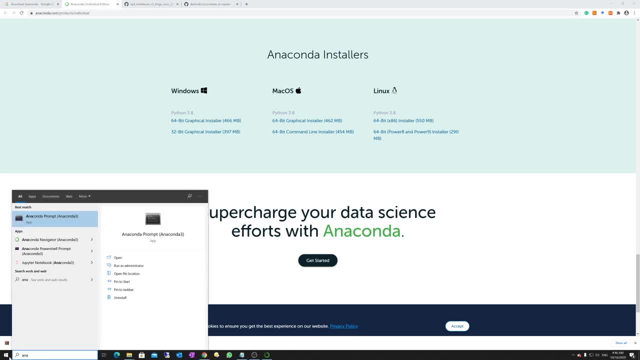 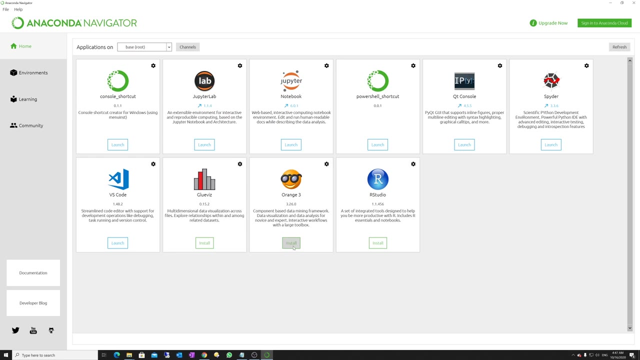 super simple to install. now I assume that you have already installed the anaconda. so in the Windows search bar if you write the anaconda like this, so you will reach here like anaconda navigator. if you press the anaconda navigator you will reach to this page. over here you can observe that we have green buttons. 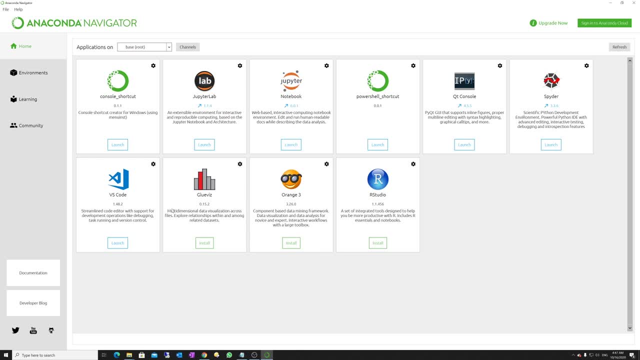 and blue buttons to launch right. so in your case, as you install the navigator, so all of them will be green and you can just click the install button of the Jupyter notebook. now I assume that you have installed anaconda navigator and Jupyter notebook. once you installed the both of them, it's better. 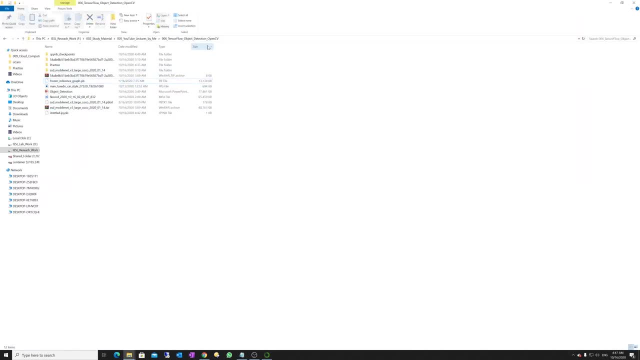 to create a new folder, right? so in my case it's full, but in your case the folder will be empty, right? so create an empty folder for your project. then. then again, you should write anaconda, and this time, rather than clicking anaconda navigator, you should press the anaconda prompt. 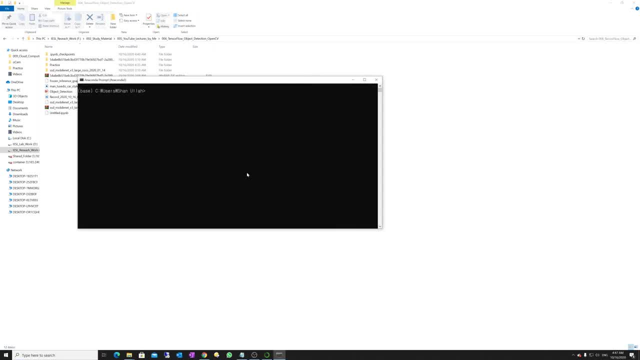 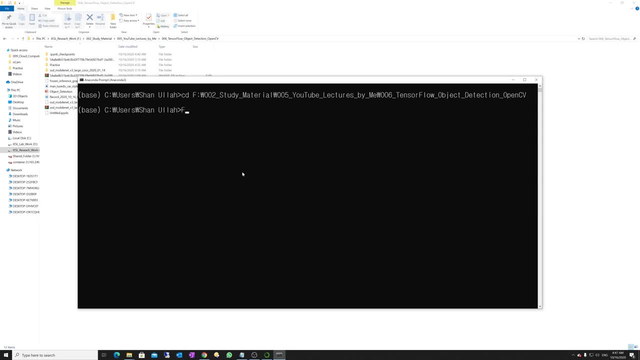 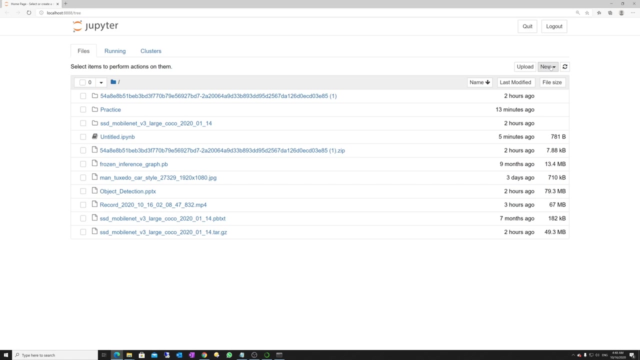 right. so once you click this- let me zoom for you- all you need is just cd and uh, paste the path and then change the drive and just write Jupyter notebook. once you write a Jupyter notebook, okay, uh, a window will be appear like this, right? so all you need is you just create. 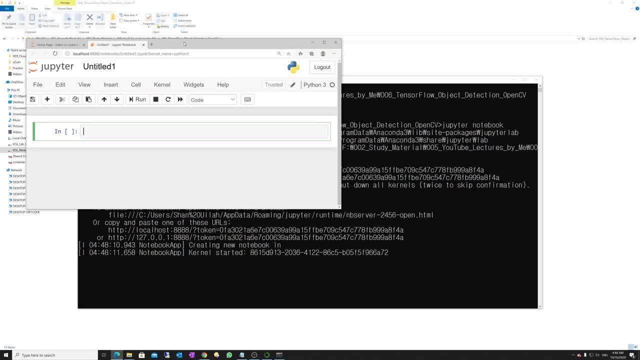 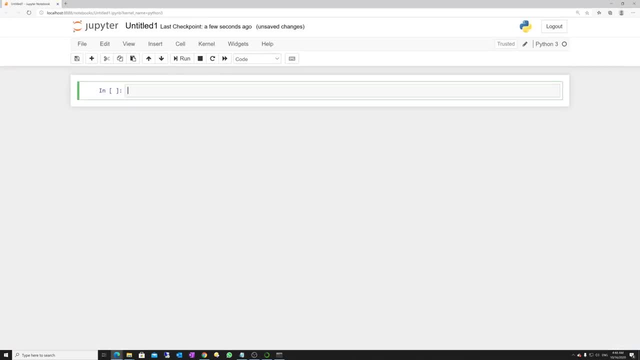 a new python, uh, Jupyter notebook, and let me separate for you guys, okay, okay, the first thing we need to do is to import opencv, right? so import, or cv2, is the command in order to install opencv. definitely, uh, at this moment you have installed the anaconda navigator. 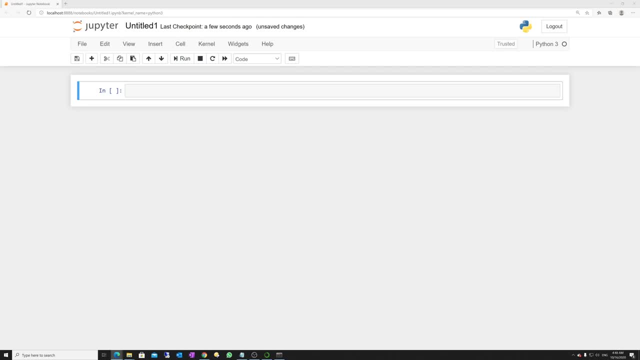 do this. so we need to do the following thing. okay, the first thing we need to do is to import open CV. right? so import CV 2 is the command in order to install open CV. definitely, at this moment you have an installed, the anaconda navigator and the open an jupyter notebook. so far, so. 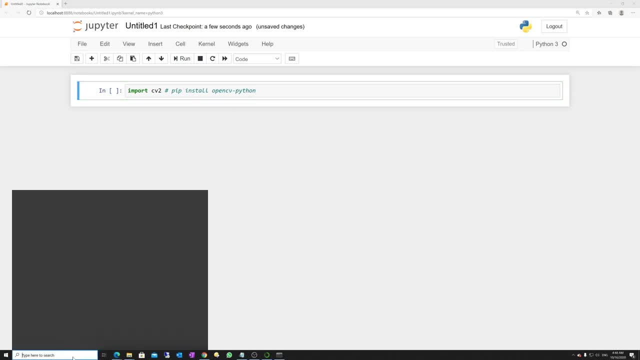 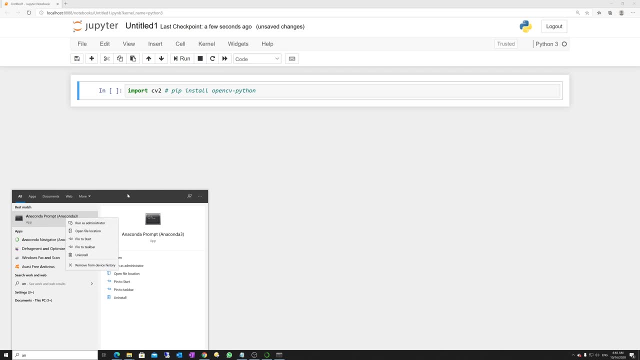 open c right. so all you need is to just visit anaconda prompt again and this time make sure that you run it as an run as administrator. once you run it, uh, you, all you need is to just copy this command and just run it, right. so open c will be installed, okay. the second tool we need is to 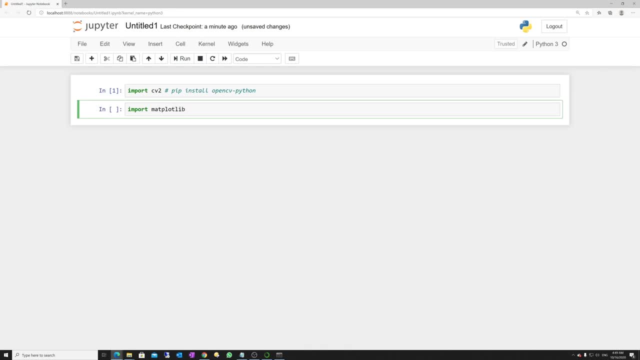 import matplotlibpyplot as plt, right. so in order to install this, you need into pip install matplotlib, right. so again, like run as an administrator, then anaconda prompt, and just write this, this command, and you will be uh good to go, right. so now i assume that, uh, you have. 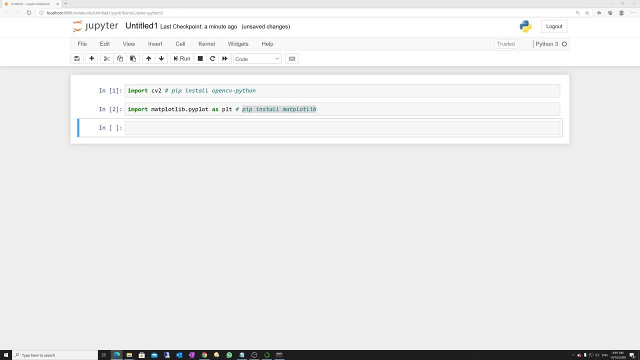 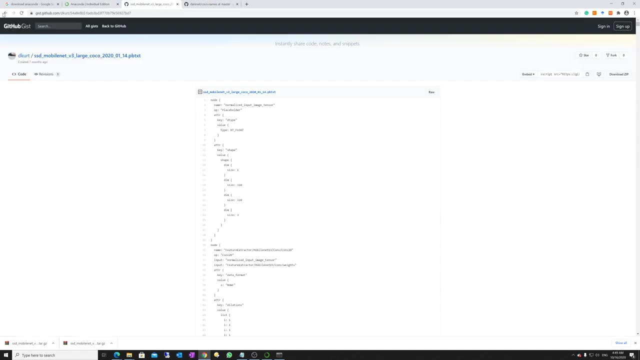 installed these four candidates. you have installed these four candidates, such as, for example, the open cv and matplotlib. okay, so let me tell you how to start. where to start the for the object detection, right? okay? so this is the open cv page. official github link i will provide in the videos, just 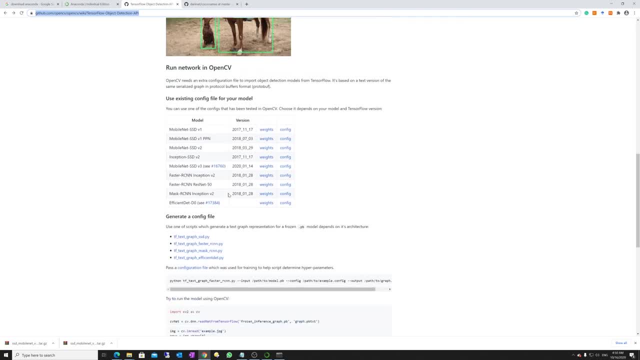 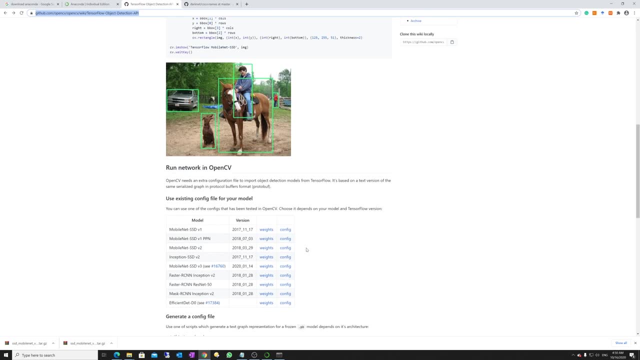 description. so once you visit over here, you will find many deep learning architectures- already pre-trained models- available to you and you will be able to use them in your project. you will be able to use them in your project and they are based on tensorflow right, so they are. 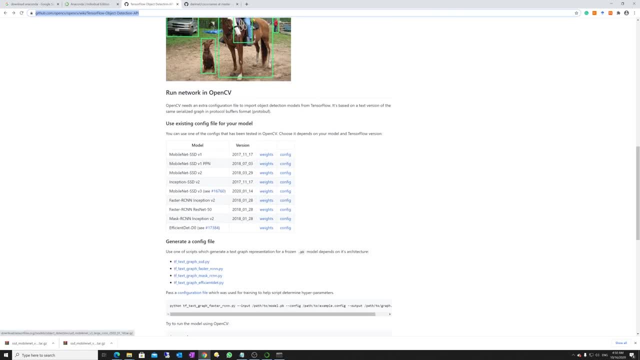 although they are based on tensorflow, but you can just download and you can use open cv to load them. that's what we are doing, going to do right now. so the most uh recent one is mobilenet ssd version 3. that is discussed in the beginning of the video. so all you need is to just 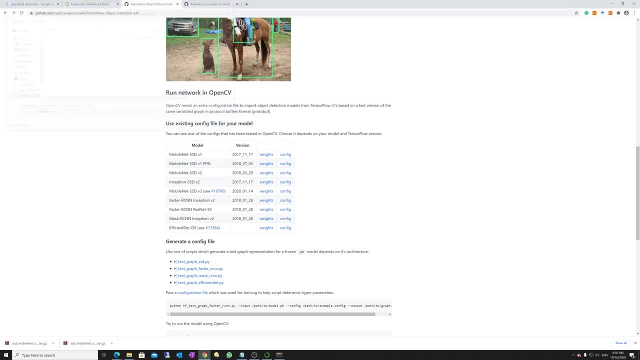 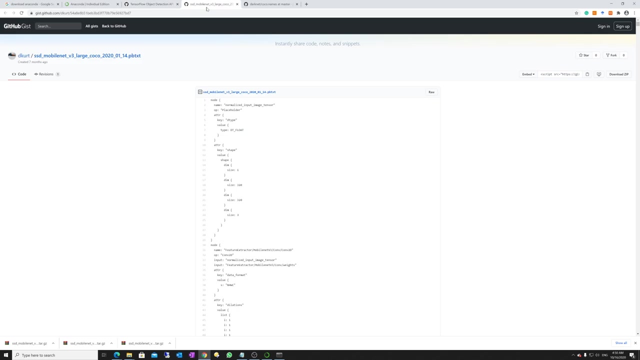 write and save link. okay, or you just click the. click it so it will be downloaded right. and another important thing is: one are the weights like the, your deep learning architecture. and the second thing is your configuration. if you click to the configuration, you will be here right. 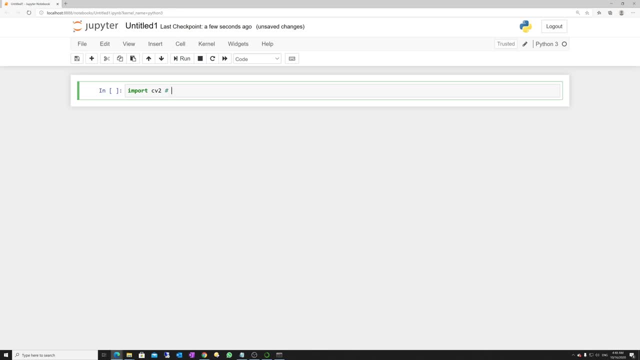 the open notebook so far. so pip install opencv. dash python is the command to install the openc, right. so all you need is to just visit anaconda prompt again and this time make sure that you run it as an run as administrator. once you run it, uh, you, all you need is to just copy this command and just run it. right, so opencv will be installed and Id through the command like this in a minute. I hope you've found this good and I'm sure y'all do not need one, so if you do have any questions, enlist the work in the comments here below. really appreciate your interest, either video or on your own req, comments or cellåbank. is there this and I will see you in the next video. but I will see you on the next video bye-bye. so, pinky, thanks guys, see you, ericg ord. 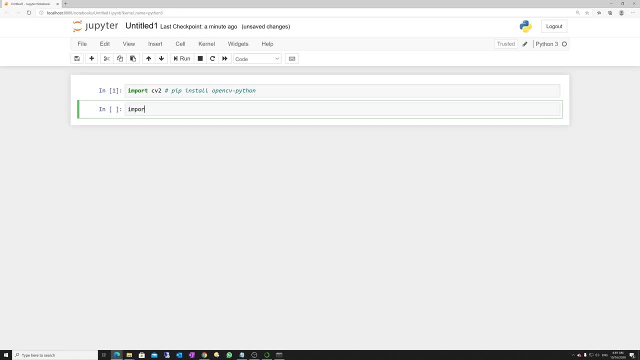 okay, the second tool we need is to import matplotlib dot pyplot as plt, right. so in order to install this, you need into pip, install matplotlib, right. so again, like run as administrator, then a conda prompt and just write this, this command, and you will be, uh, good to go right. 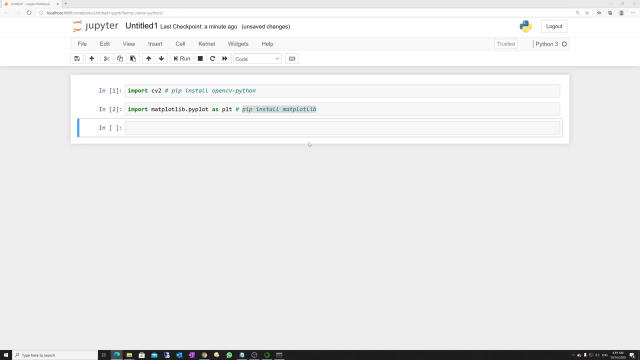 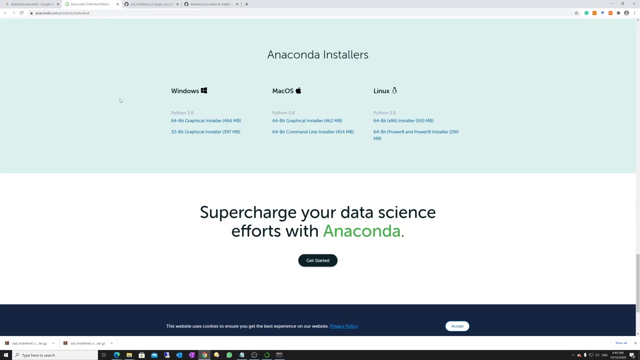 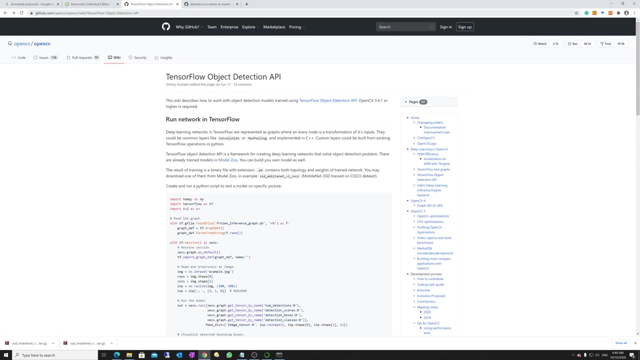 so now i assume that you have installed these four candidates, such as, for example, the opencv and matplotlib. okay, so let me tell you how to start, where to start the for the object detection, right? okay? so this is the opencv page official github link i will provide in the videos, just 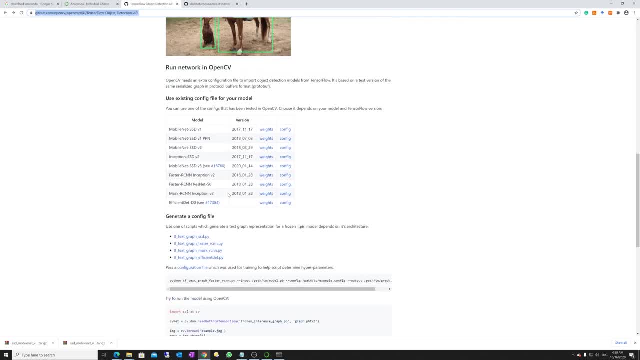 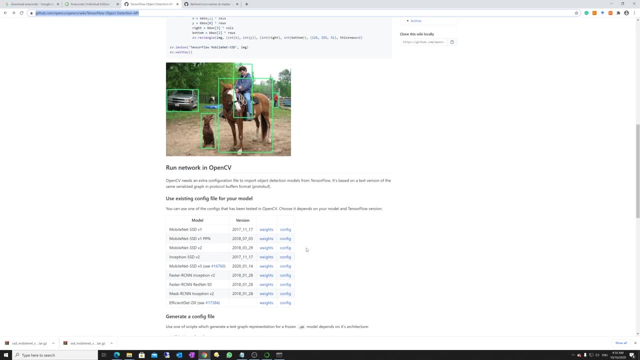 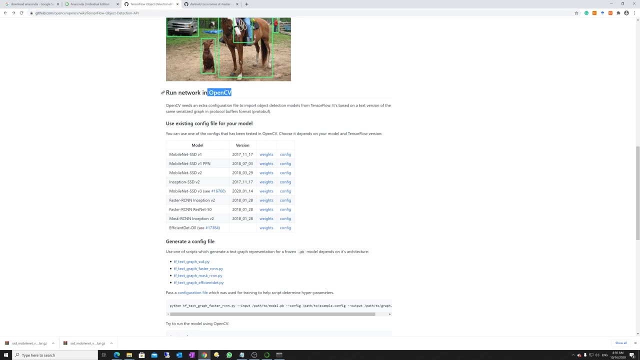 description. so once you visit over here, you will find many deep learning architectures, already pre-trained uh models available and they are based on tensorflow, right. so they are based- although they are based on tensorflow, but you can just download and you can use opencv to load them. 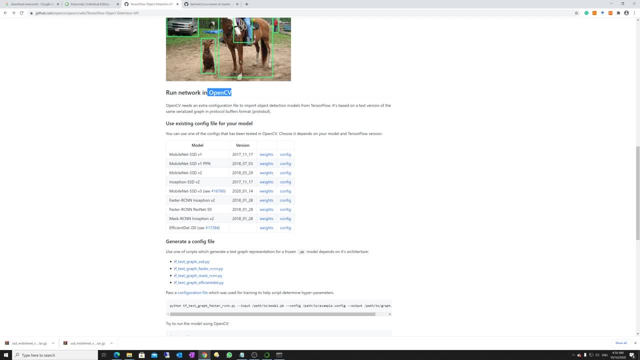 that's what we are doing, going to do right now. so the most uh recent one is mobile net ssd version 3 that is discussed in the beginning of the video. so all you need is to just write and save link, okay, or you just click the. click it so it will be downloaded right. and another important thing: 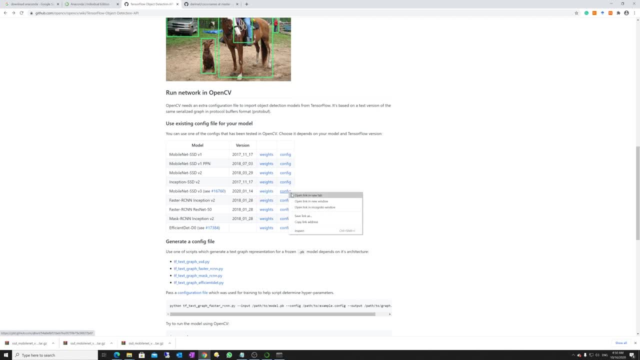 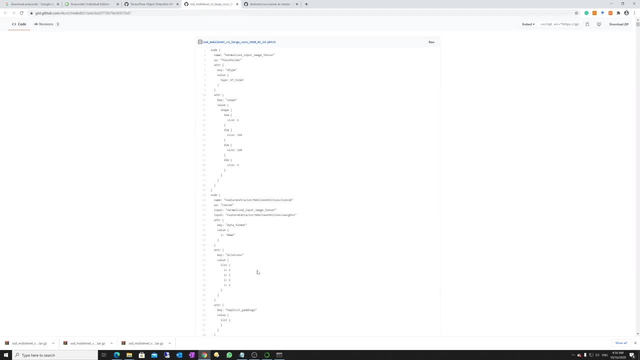 is one are the weights, like the, your deep learning architecture, and the second thing is your configuration. if you click to the configuration, you will be here right. so, as you can see over here what is the com, the configuration like, what is the input size and a lot of other information is available, so you need to load it as well, so just download. 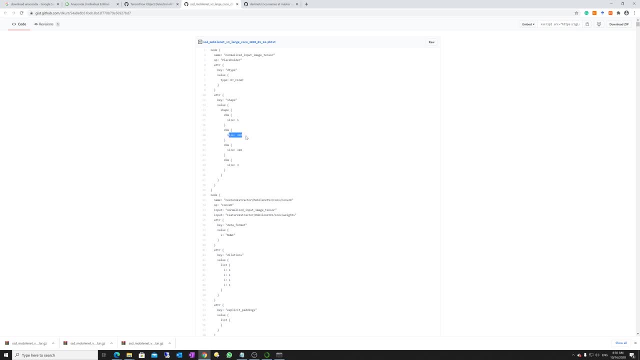 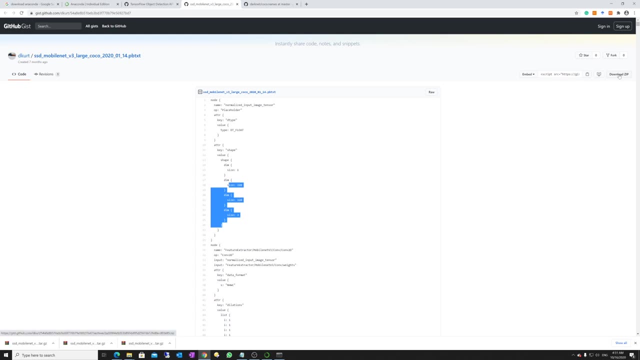 so, as you can see over here, what is the com, the configuration like, what is the input size and a lot of other information is available, so you need to load it as well. so just download zip, right you? once you download zip, for example, let me download for you guys. so once i press download, it will be. 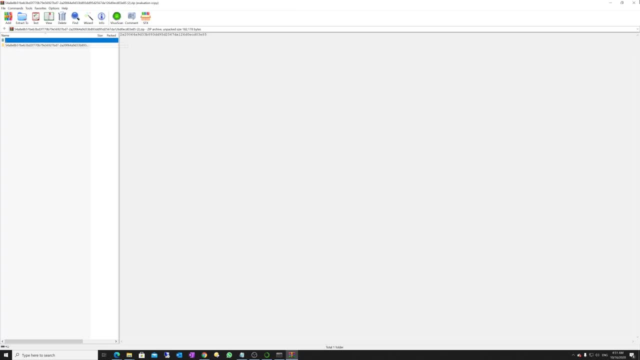 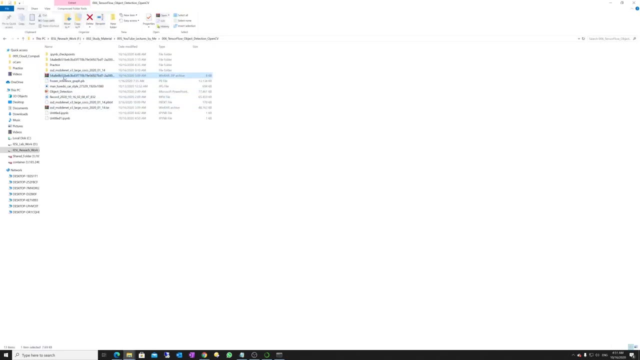 download with that, with some, you will be able to download it and you will be able to download it with the name like this: so, in my case, i have already downloaded and copied in my folder like: this is my graph and this is my, okay, so this is the version. uh, this is the graph of the deep learning architecture which i recently. 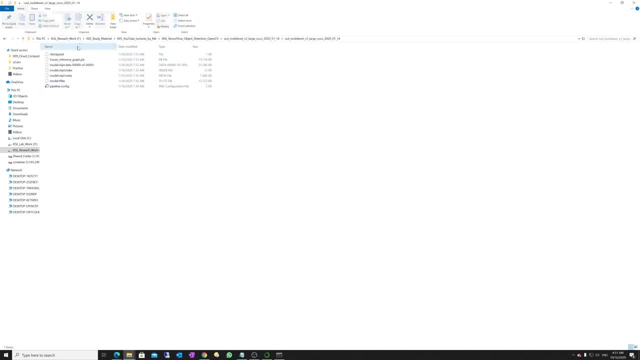 downloaded. so when you, once you extract the folder, you will find a lot of them. so the most important one is frozen inference graph. all you need to do is just copy and paste it wherever you are going to use. so this is my project folder. i just created this uh untitled new, uh python notebook, so i have just placed over here. 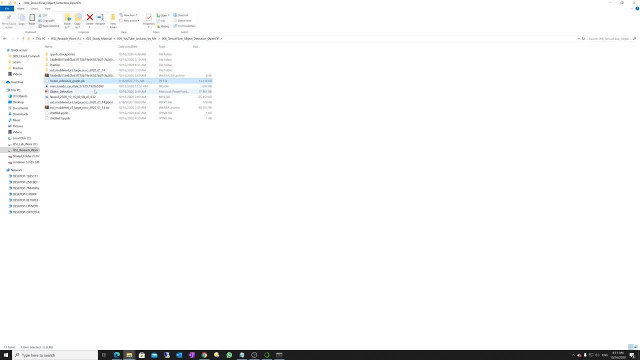 right. so in any folder you can place wherever you are working right in the project folder. similarly, if you visit this, if you extract this the to the graph configuration, you just need to copy this configuration and just paste it wherever you are working right. so now, as i have these two candidates, 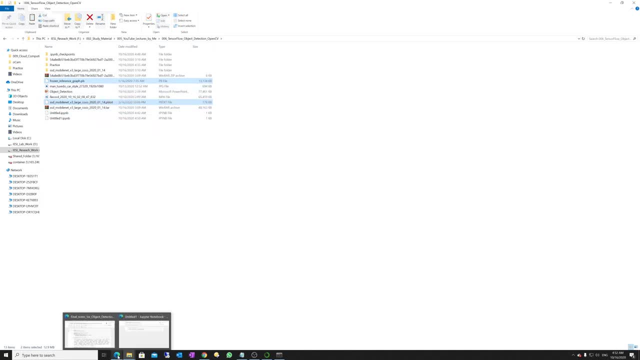 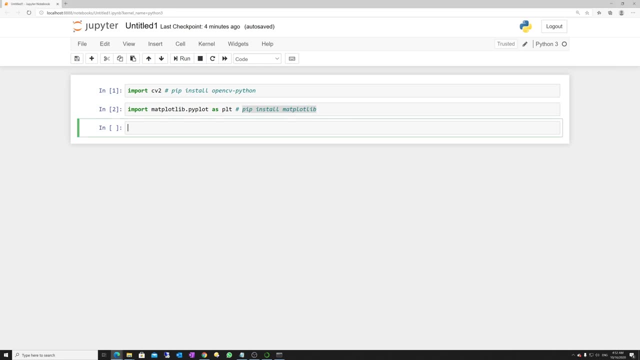 inside my folder where i'm working, okay, so i can just load it, right, okay, so let me load them, so let me give them names. for example, my configuration file is this: and: and. secondly, if you have in any other folder, you don't need to copy, so you can just. 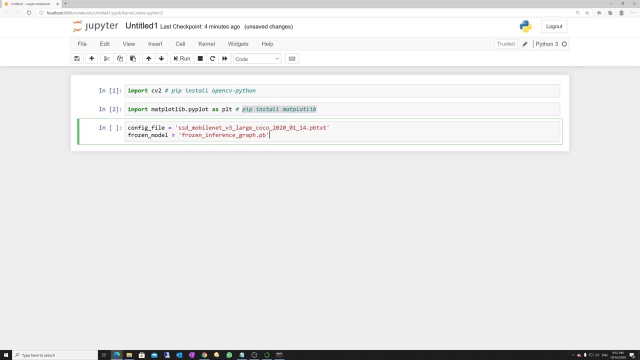 provide the path right over here. so in my case i have copied in my main folder so i need to execute. so before diving it, uh, it's better. for example: okay, let me load the model. so the model is equal to sorry, cv2 dot dnn. if i press the tab, i will have multiple options right, so the most important one is the. 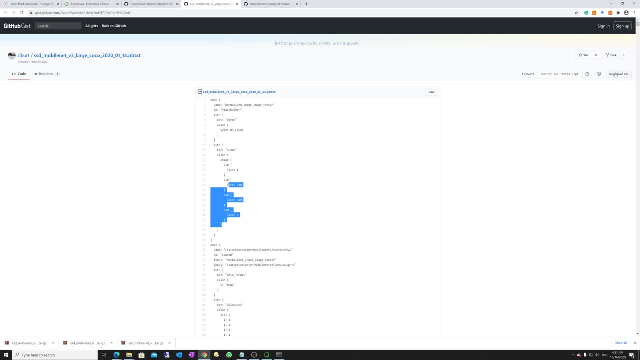 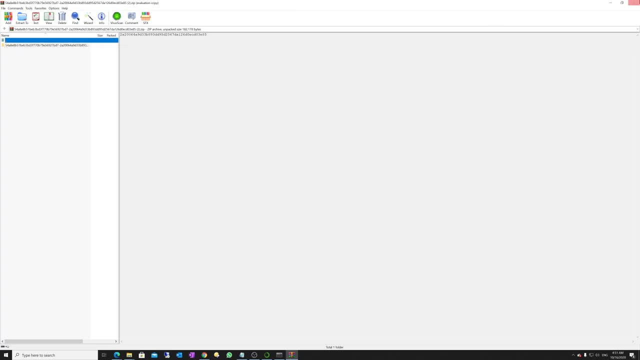 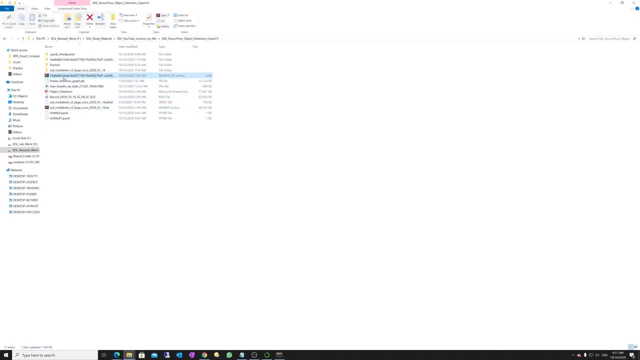 zip, right, you, once you download, zip it. for example, let me download for you guys. so once i press download, it will be downloaded with the some name like this: so in my case, i have already downloaded and copied in my folder like this is my graph and this is my. 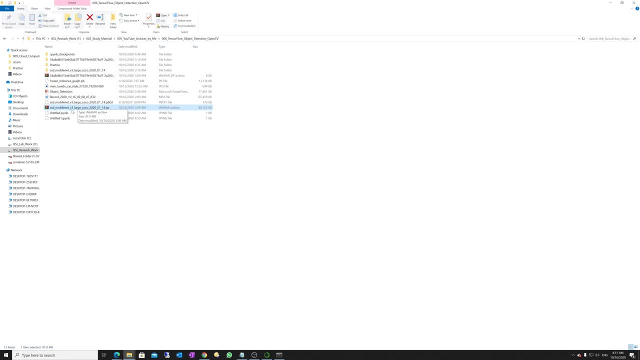 okay, so this is the version. uh, this is the graph of the deep learning architecture which i recently downloaded. so when, once you extract the folder, you will find a lot of them, so the most important one is frozen githubcom, which is the the most common organization which is going to help you in your deep learning architecture. so once you extract the folder, 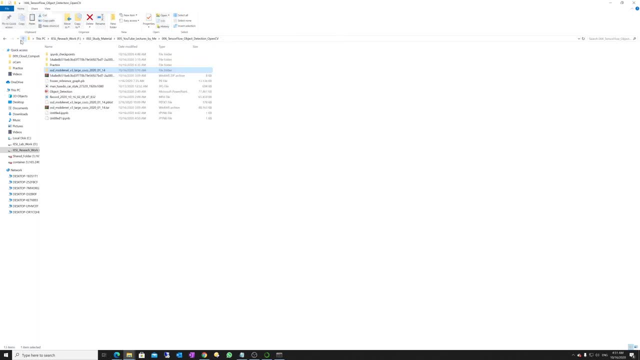 inference graph. all you need is just copy and paste it wherever you are going to use. so this is my project folder. i just created this uh untitled new, uh python notebook, so i have just placed over here right, so in any folder you can place wherever you are working, right in the project. 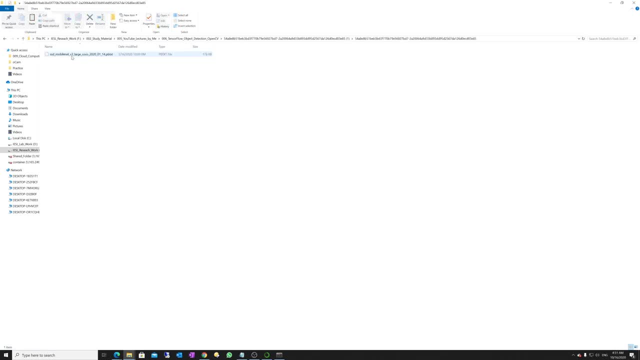 folder. similarly, if you visit this, if you extract this, the to the graph configuration, you just need to copy this configuration and just paste it wherever you are working. right, so now, as i have these two candidates inside my folder where i'm working, okay, so i can just load it, right, okay, so? 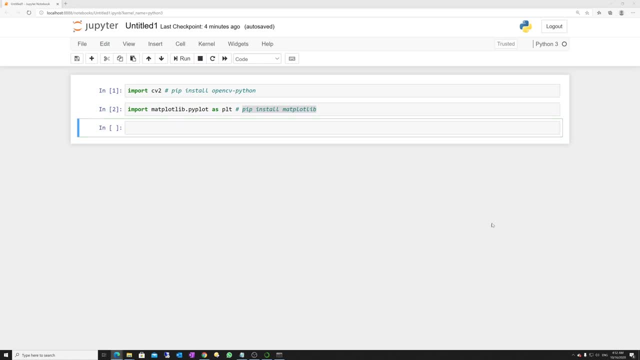 let me load them. so let me give them names. for example, my configuration file is this: and: and. secondly, if you have in any other folder, you don't need to copy, so you can just provide the path right over here. so in my case, i have copied in my main folder, so i need to execute so before diving. 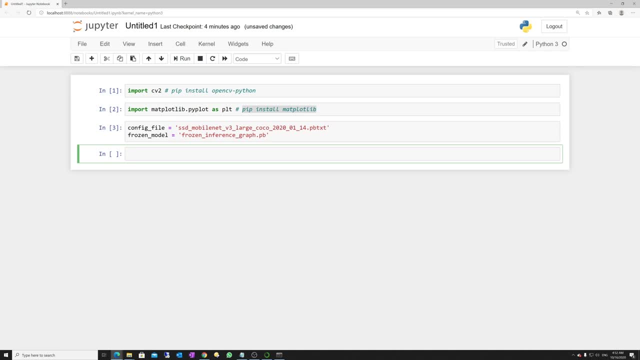 it. uh, it's better. for example: okay, let me load the model, so the model is equal to sorry, cv2, dot, dnn. if i press the tab, i will have multiple options, right, so the most important one is the dnn detection model, right? so there is. 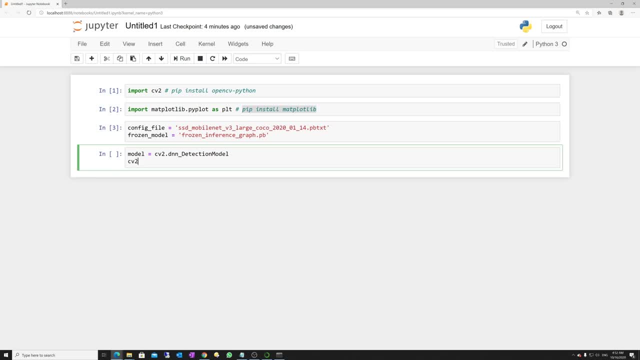 one method and the second method is, for example, if you write cv2, dot, dnn- sorry, dnn, dot, for example, and then you can just read from the tensorflow as well. but i will follow the like this method, right, not the run from tensorflow, but we do have another method as well. 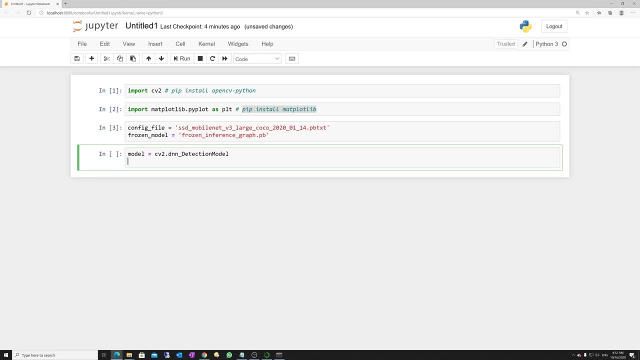 dnn detection model. right. so there is one method, and the second method is, for example, if you write cv2, dot uh, dnn, sorry, dnn, dot, uh. for example if you press a tab and then you can just uh read from the tensorflow as well. but i will follow the 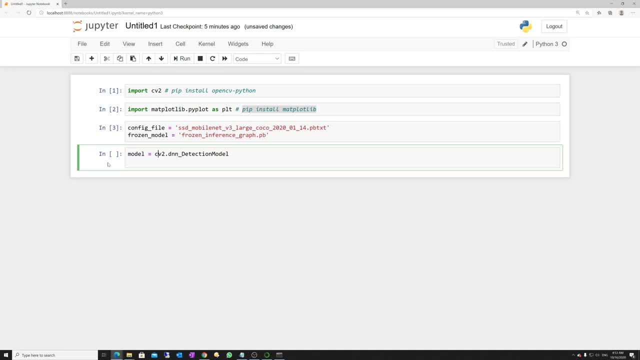 like this method, right, not the run from tensorflow, but we do have another method as well. so in this case i can give: the frozen model is the first candidate and the second candidate is config file. right, so now? okay. so now in my memory i have loaded the tensorflow pre-trained model, right? 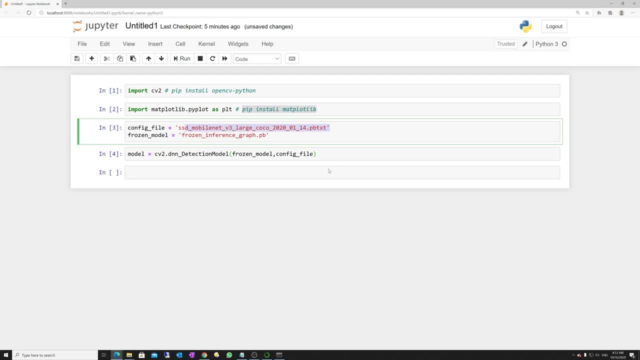 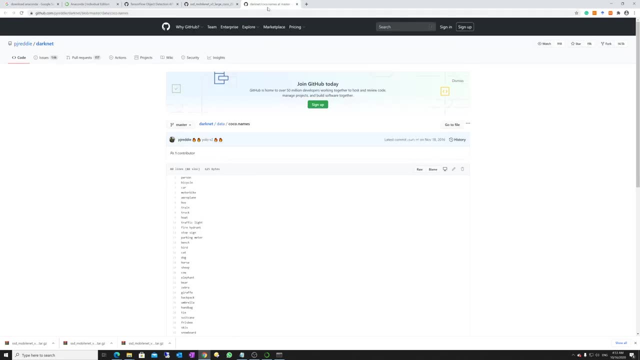 so this is my model and this is my configuration file, right? so once i have loaded my model- so i mean uh, single function- right now i can save it for any other example. data set: right, so that i have already saved and i can save in my memory again. um, i can also do the same with on. 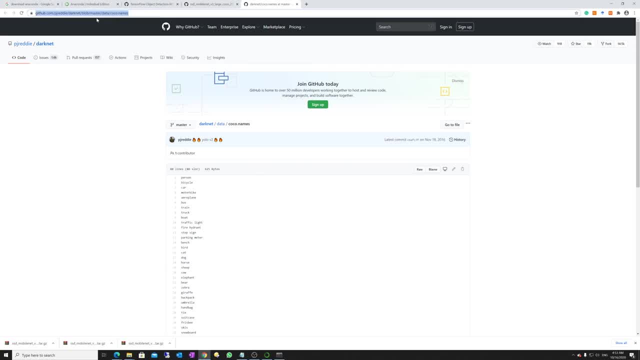 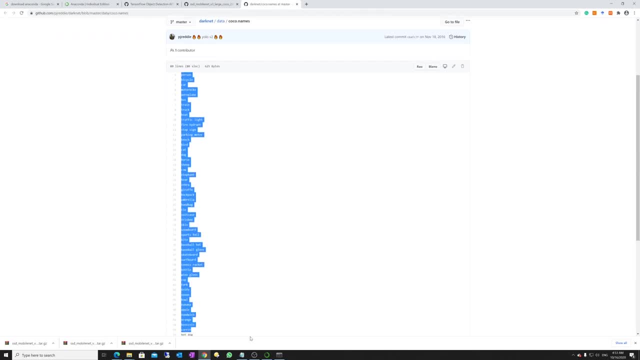 my own macbook pro, so i will just keep adding this to my macbook pro and uh, this is the only point i need to do in my macbook pro. uh, the other important thing we need to have is this darknet right uh labels. so in this case, all you need is to just uh, for example. i will also provide the link. 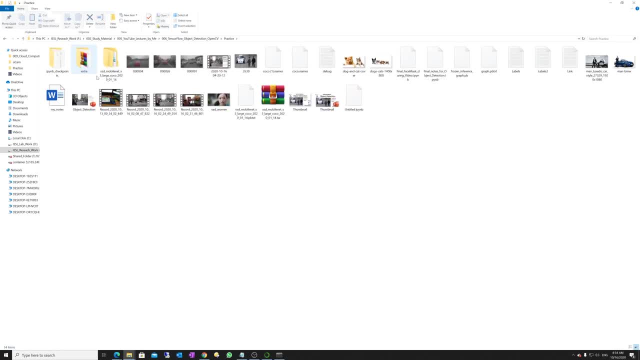 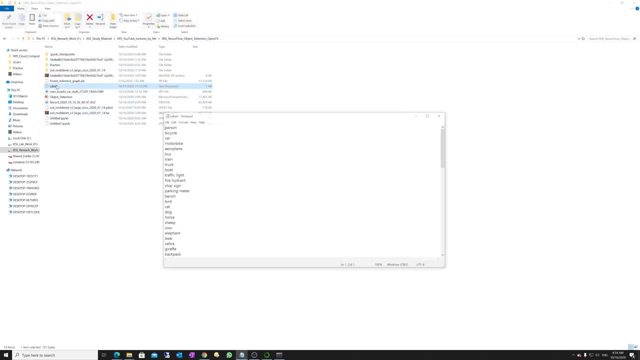 so once you have- for example, i have already the labels. okay, these are my labels. so let me show you what are my labels. okay, so i have just copied in a text file. so all you need is just create a text file like this. okay, and create a text file and just copy all of the 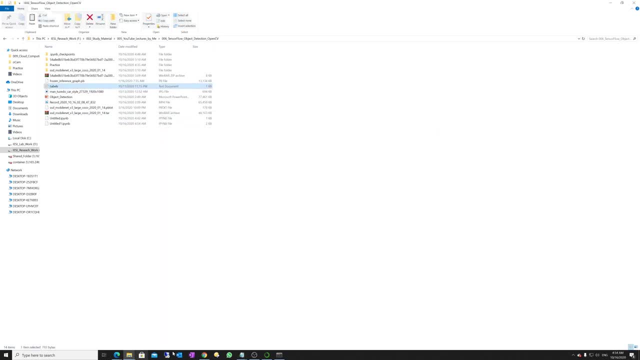 labels right. so now the third thing: i assume that you have already copied the labels right and just download it, okay? so once you download the labels, why we need labels, right? so in order to check our answer is correct or not right. so that is why we need labels, okay, so um, 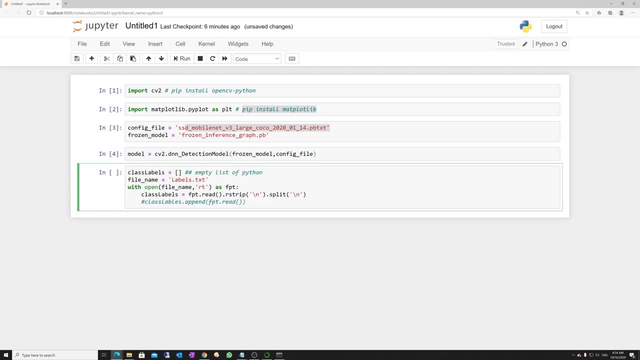 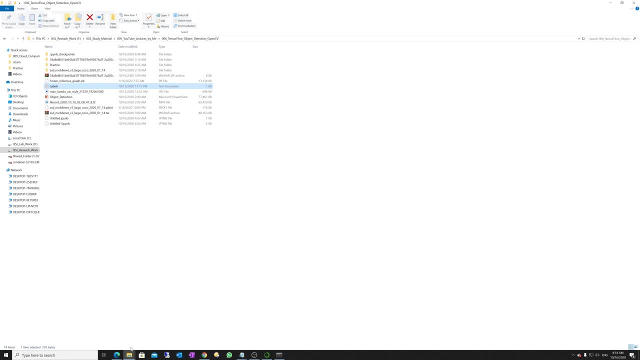 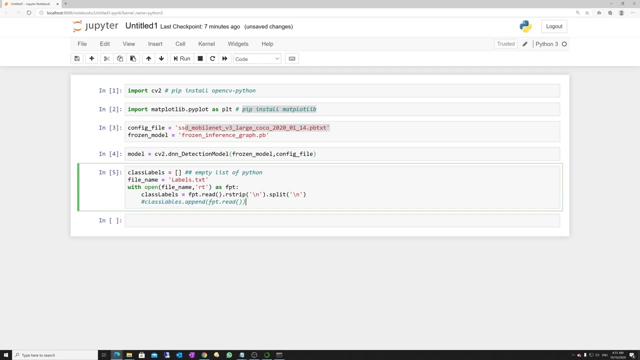 let me write a code for you for loading. so labeltxt. i have just copied in my folder, right? this is my labeltxt containing all 80 classes. okay, so i can just execute like this. i can also do using a pen, but i'm over here, i'm not using. 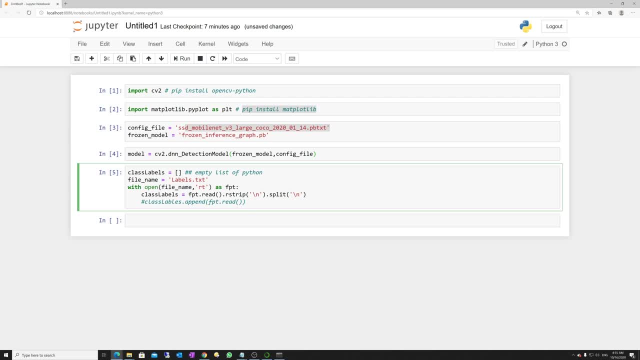 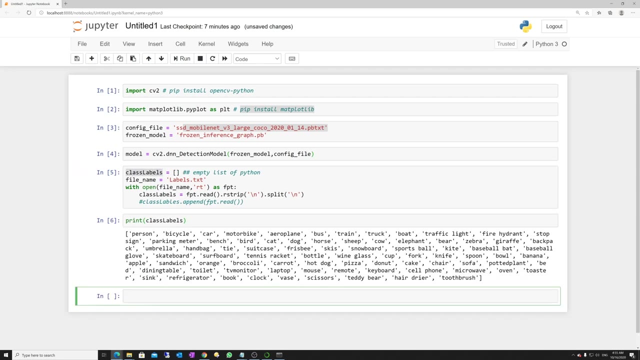 doing it using a pen, but i'm just doing it like i'm reading the label and creating the list of python, and just doing it like this. so let me print for you, if i print the class labels that have already been appended. so you see we have a list of this, all 80 classes, right? if i check the 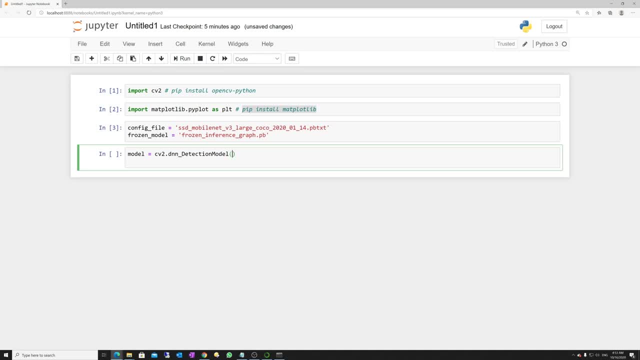 so in this case i can give the frozen model as the first candidate and the second candidate is config file, right, so now? okay. so now in my memory i have loaded the tensorflow pre-trained model, right? so this is my model and this is my configuration file, right? 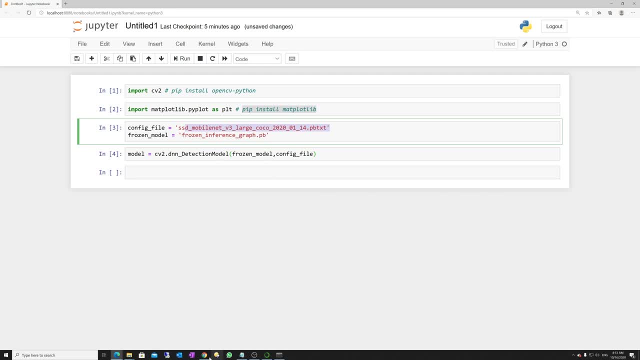 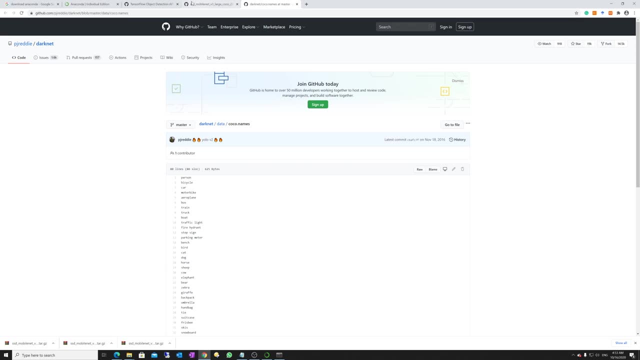 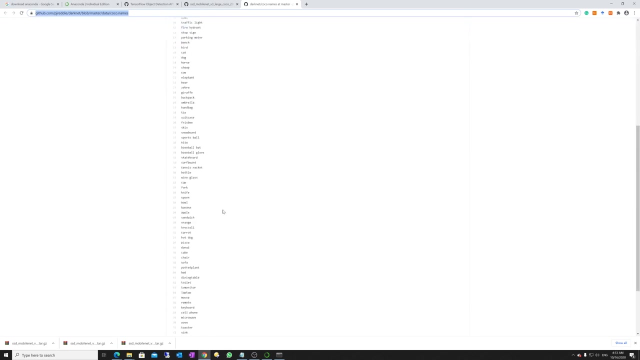 so, once i have loaded my model. so another important thing we need to have is, uh, this darknet right uh labels. so in this case, all you need is to just uh. for example, i will also provide the link of this darknet coco names, okay, so all you need is to just copy all of them, right? so 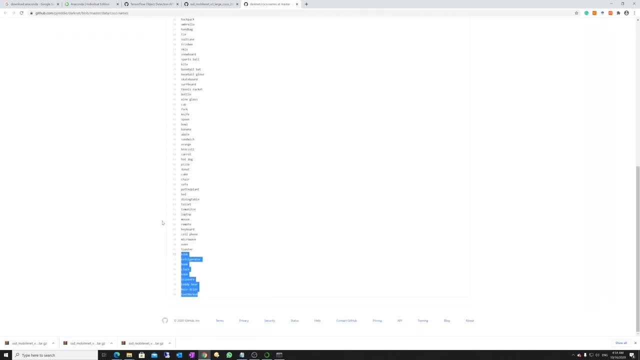 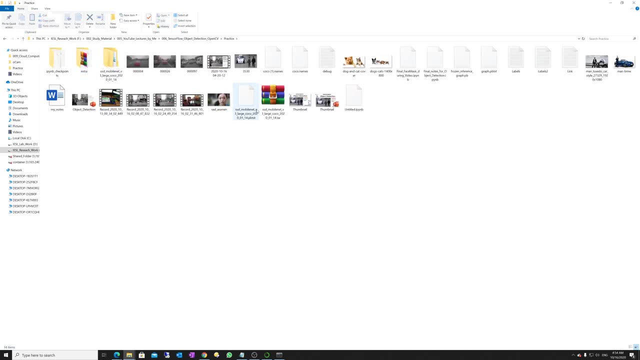 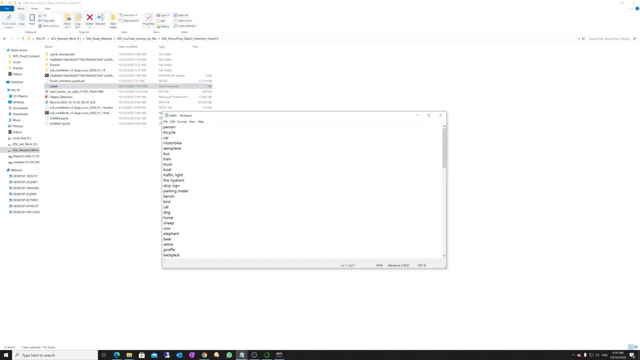 there are 80 classes. as i told you before, in the coco dataset. there are 80 classes, right? so these are the labels. so once you have, for example, i have already the labels. okay, these are my labels. so let me show you what are my labels. okay, so i have just copied in a text. 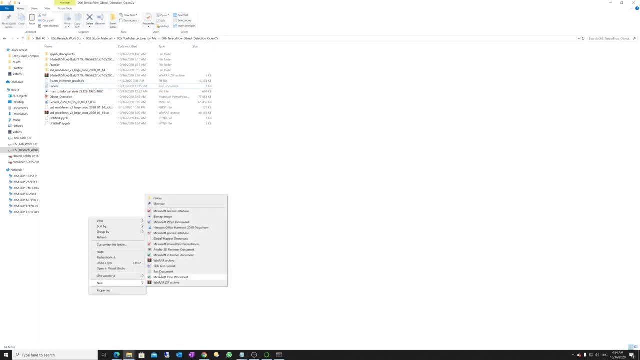 file. so all you need is just create a text file like this. okay, and create a text file and just copy all of the labels, right? so now the third thing. i assume that you have already copied the labels, right, and just download it, okay? so once you download the labels, why we need labels? 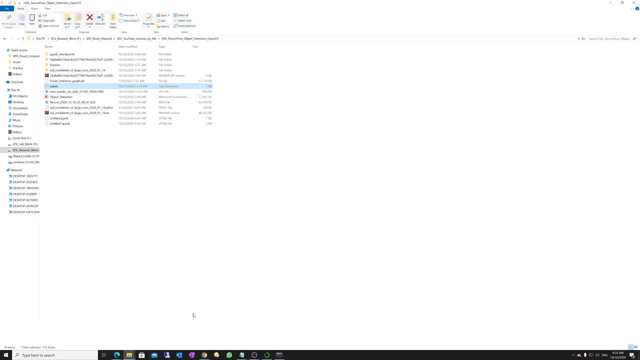 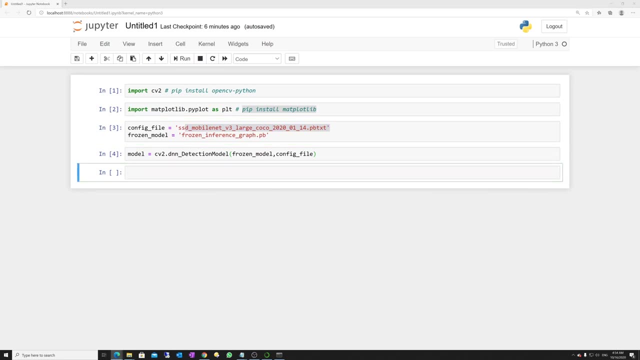 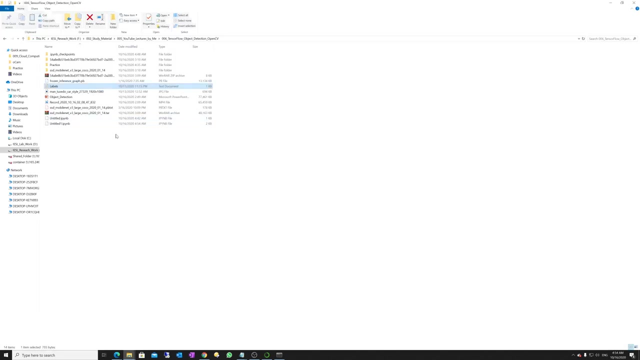 right? so in order to check our answer is correct or not right? so that is why we need labels. okay, so let me write a code for you for loading. so labeltxt i have just copied in my folder, right? this is my labeltxt containing all 80 classes. 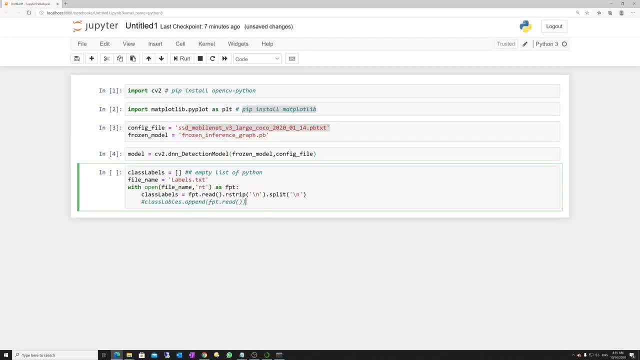 okay, so i can just execute like this. i can also do using a pen, but i'm over here, i'm not using doing it using a pen, but i'm just doing it like i'm reading the label and creating the list of python and just doing it like this. so let me print for you. 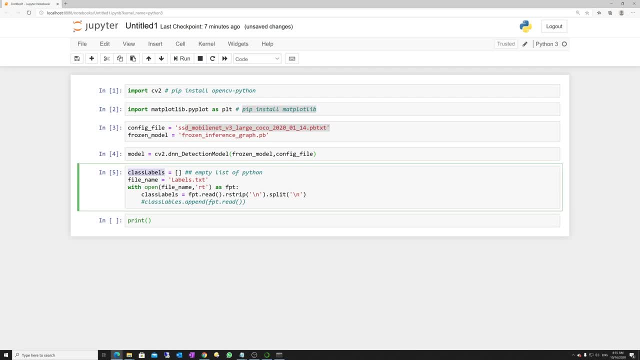 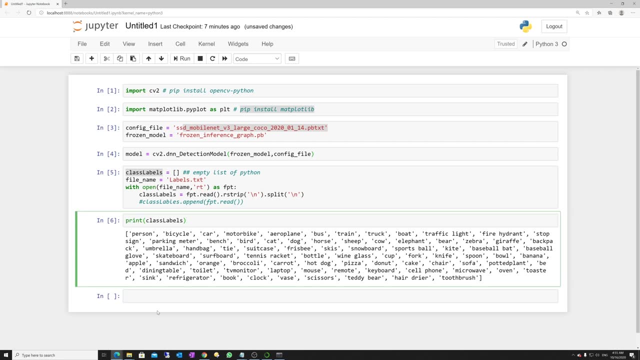 if i print the class labels that have already been appended, so you see we have a list of this, all 80 classes, right? if i check the label, i can see that i have already copied all 80 classes, right? so i can just execute like this. so let me type the length. 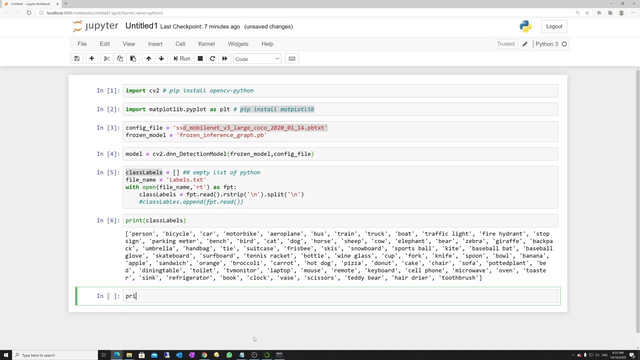 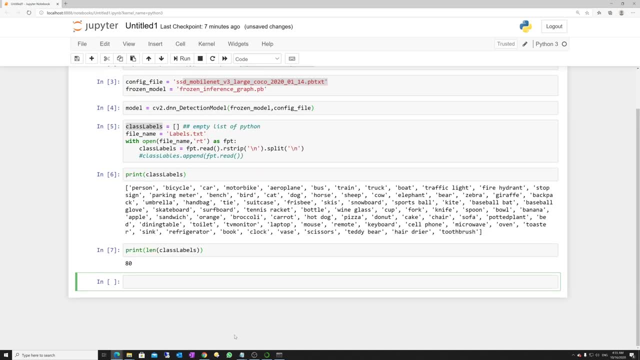 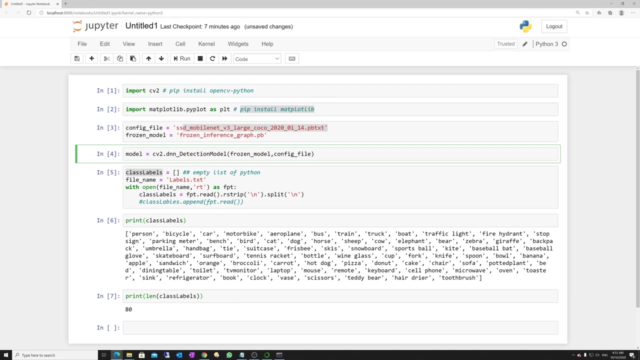 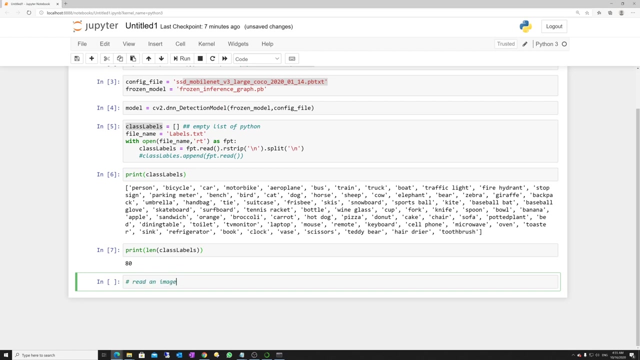 length like this: if i print the length, there are 80, right, so we have 80 uh classes and we now we have loaded, successfully loaded the model and now we are good to go. right, so for doing it, let's read an image, right, okay, so, in order to read an image, uh, what we need, okay, so the good thing is to solve. 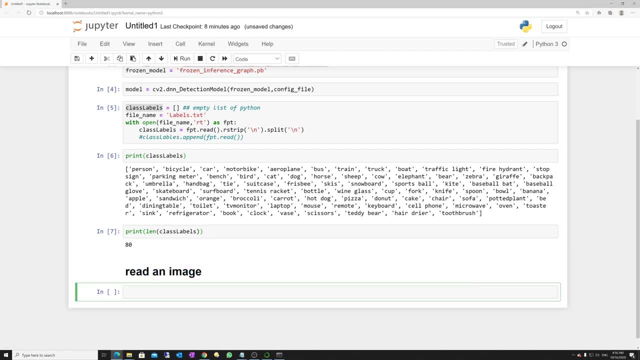 we can just convert all right into notes, right. so in order to read an image, okay, we can just uh read any image, right so this is the command cv2.im read, okay. so, before reading, uh, the image is the one very important thing we need to consider if we check the google uh over. 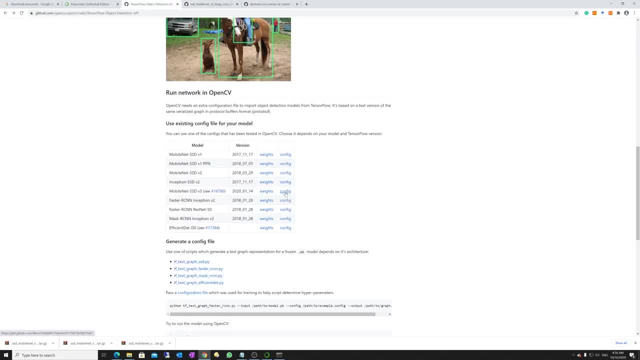 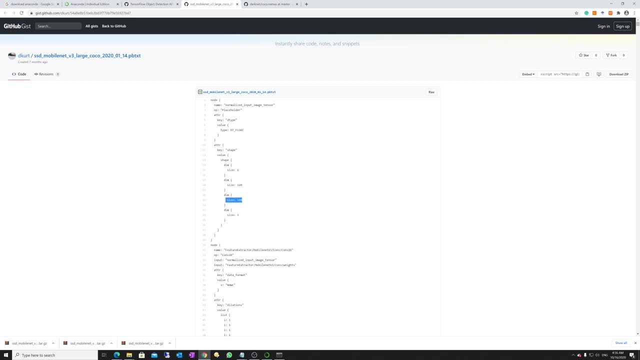 here, as i showed you that in the configuration file. if you visit the configuration file in the configuration file, you can see that the configuration file, you can see that the size is 320 by 320. right, and there are many other uh changes as well. so what we need to do is: 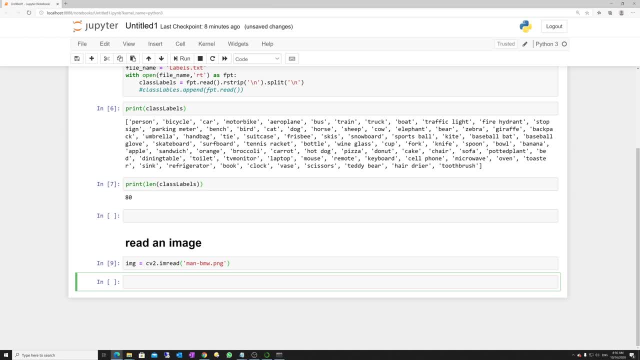 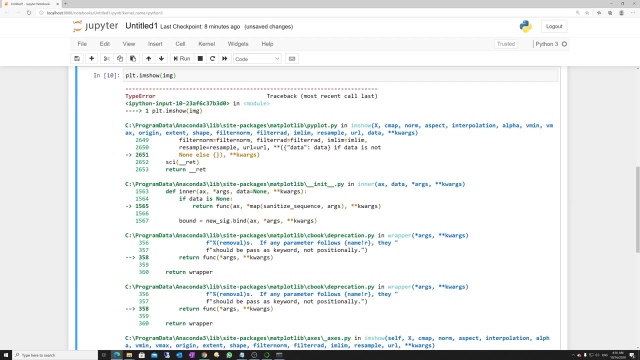 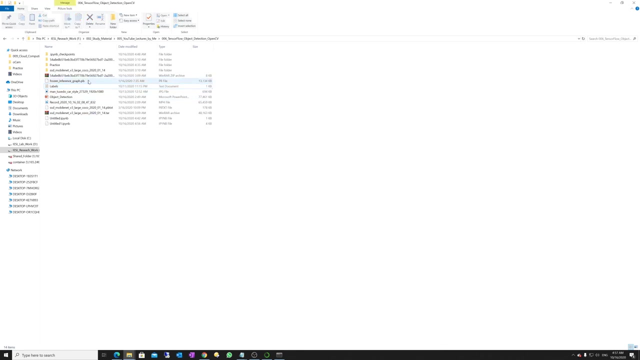 over here. if i load, for example, this image and let me show you plt dot, i am show image. so, oh, sorry, i i think i haven't copied this image. okay, let me check either this image exists or not. okay, this image do not exist, so let me load this image. make sure to have the image inside your 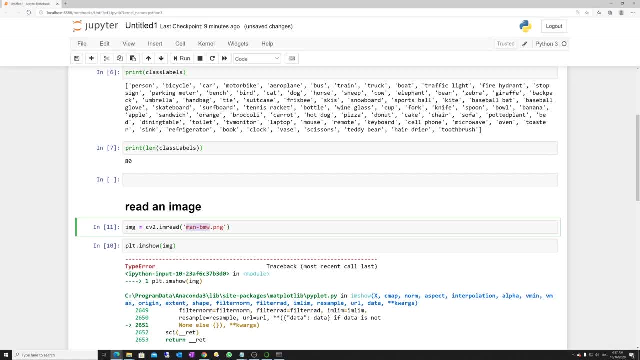 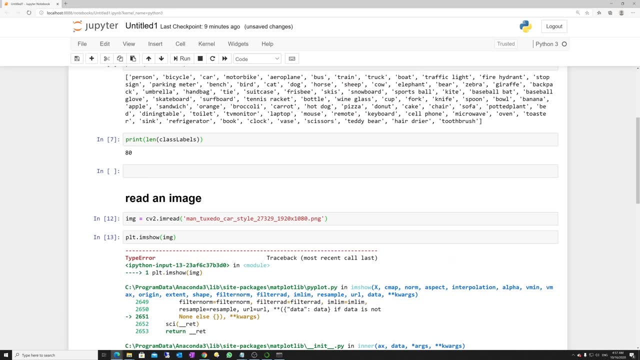 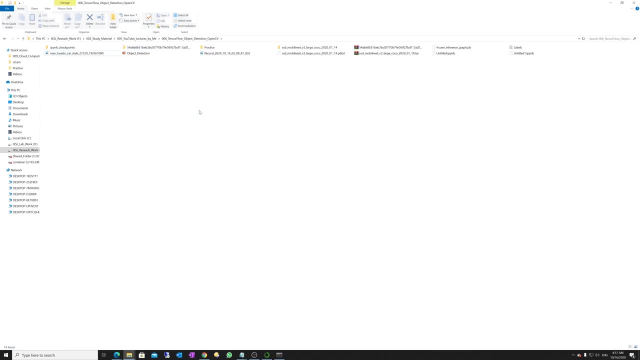 folder. actually i was okay, okay, collaboration, what is happening? uh, it may be not png, so let me check. either it's png or jpg. so you see, over here it's a jpg format. right, let me view it for you guys, large. i'll leave it in the case of the jpg and 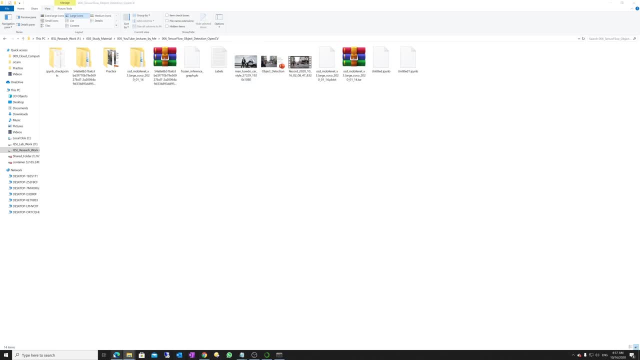 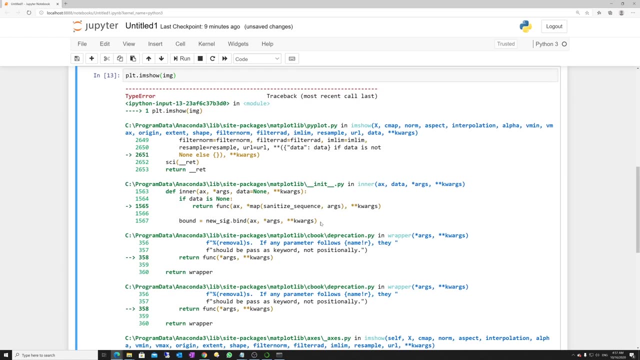 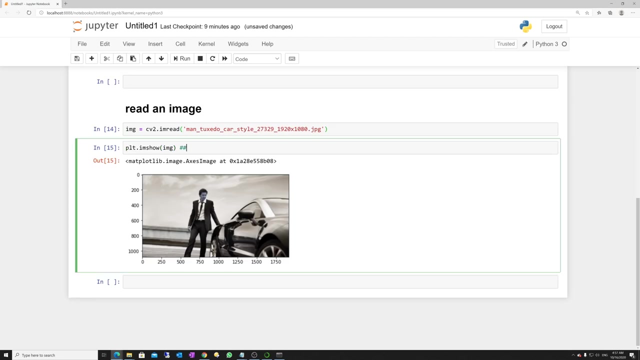 icons. so it's a jpg file, right? so make sure that to put the right format specified as well, the format should be same, right? if I write like this, then you see over here. so now it's a BGR actually. so we have BGR, right. so blue, green, red. 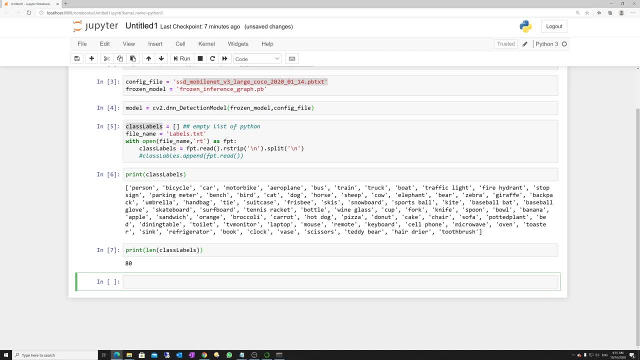 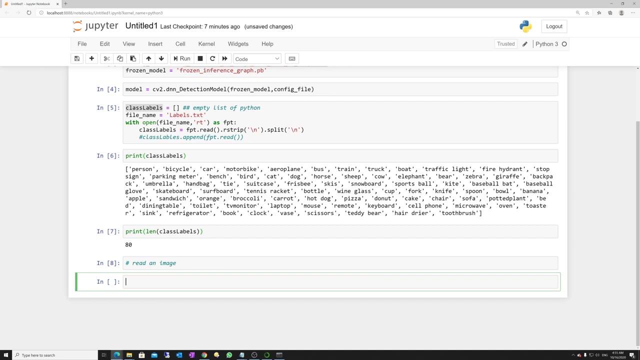 like this: if i print the length, there are 80, right, so we have 80 classes and we now we have loaded, successfully loaded the model and now we are good to go. right, so for doing it, let's read an image, right? okay, so, in order to read an image, what we need, okay, so the 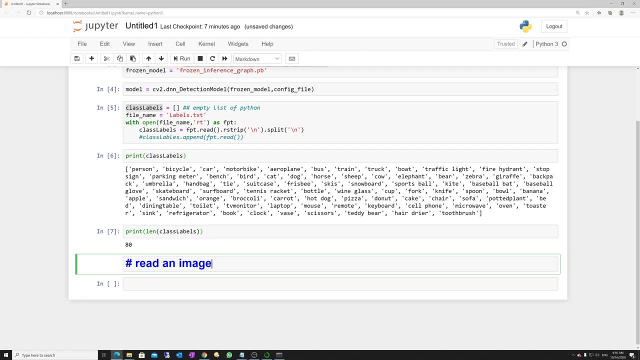 good thing is to start the model. we are going to want to have a lot of classes. okay, so i'm going to cell. we can just convert all right into notes, right? so in order to read an image: okay, we can just read any image, right? so this is the command: cv2.im read. okay, so before reading the image is: 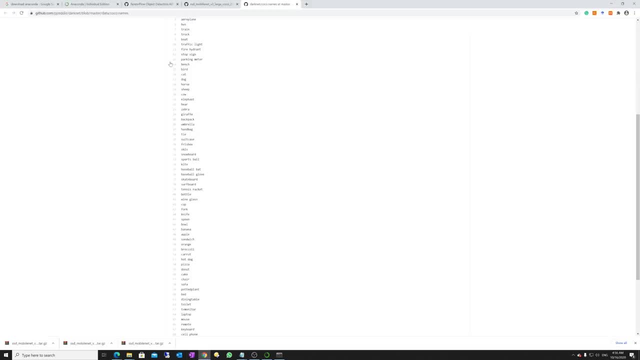 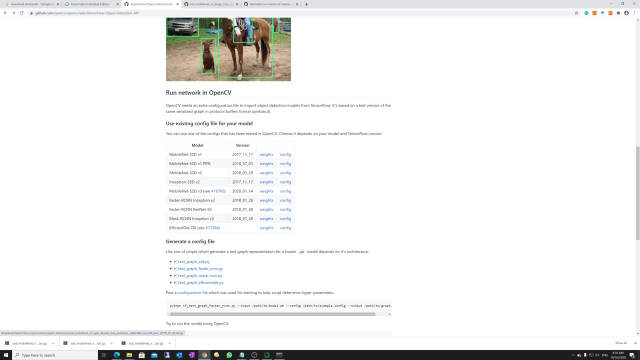 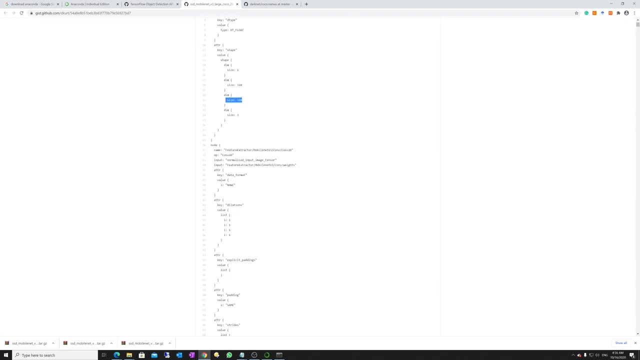 the one very important thing we need to consider. if you check the google uh over here- as i showed you that in the configuration file, if you visit the configuration file in the configuration file, you can see that the size is 320 by 320. right, and there are many other uh changes as well. so what we? 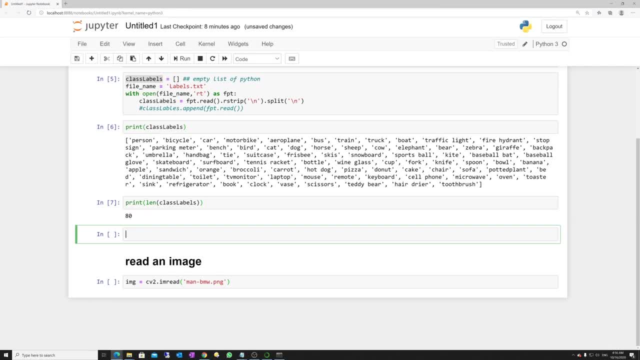 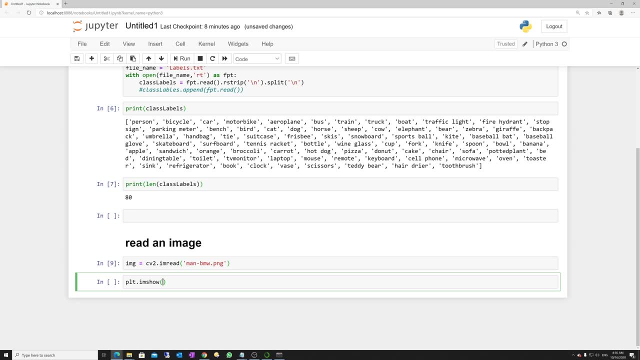 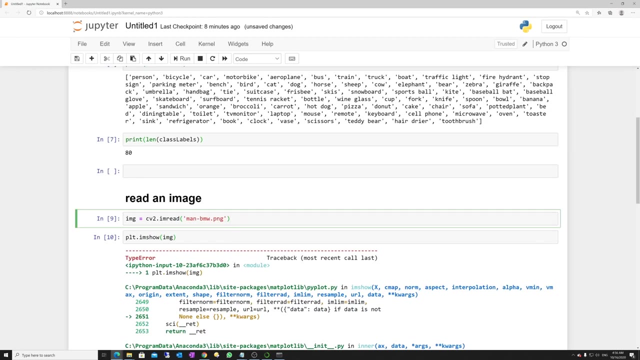 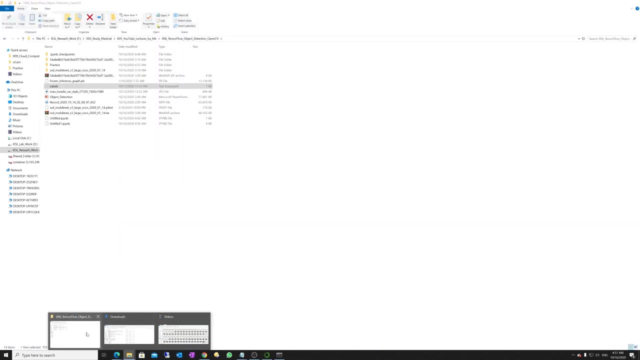 need to do is over here, if i load, for example, this image and let me show you pltim show image. so, oh, sorry, i i think i haven't copied this image. okay, let me check either this image exists or not. ah, okay, this image do not exist, so let me load this image. 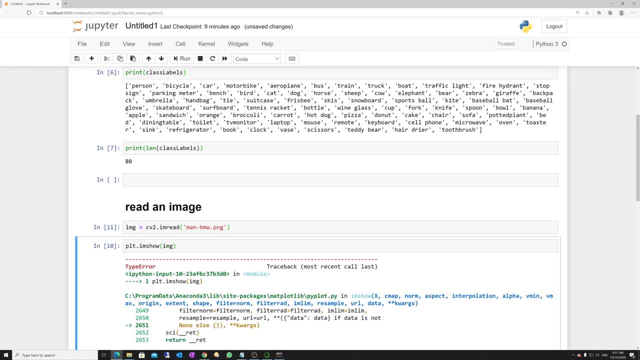 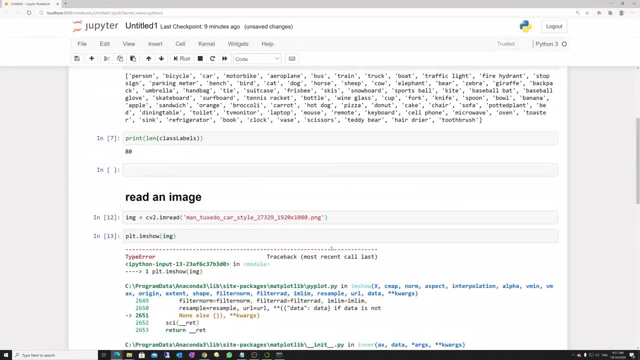 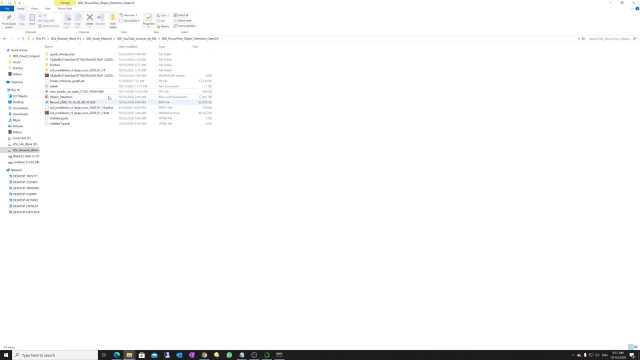 make sure to have the image inside your folder. actually, it was okay. okay, what is happening? uh, it may be not png, so let me check either it's png or jpg. so you see over here it's a jpg format, right? let me view it for you guys- large icons. so it's a jpg file, right. so make sure that to put the right. 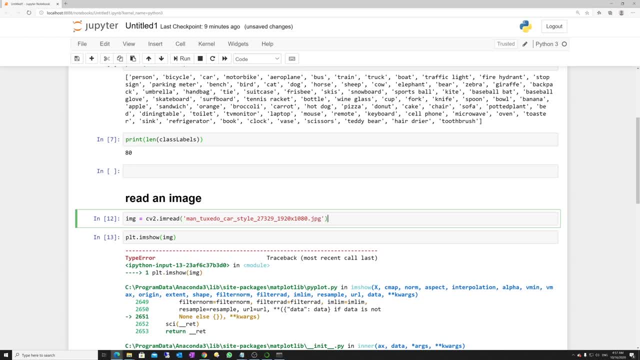 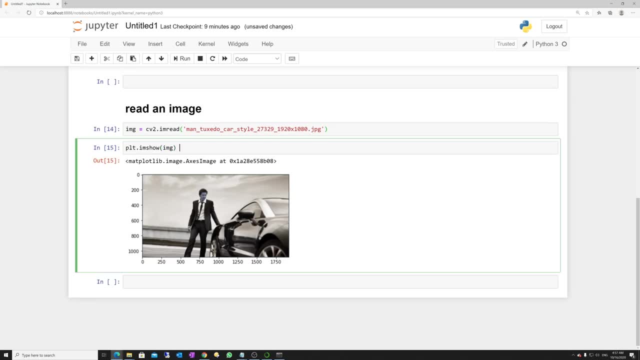 format specified as well. the format should be same, right? if i write like this, then you see over here. so now it's a bgr actually, so we have bgr right. so blue, green, red is the uh by default using c, open cv right. so if i convert into dbgb, right, and see that you do. 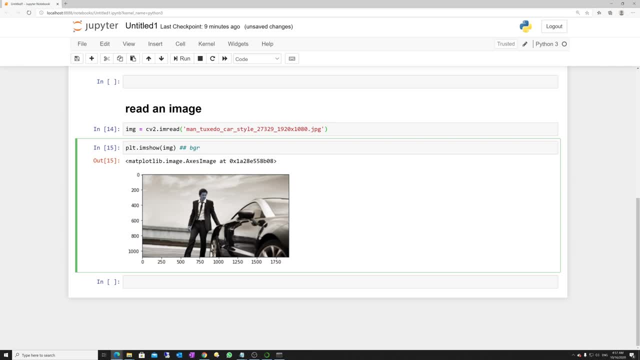 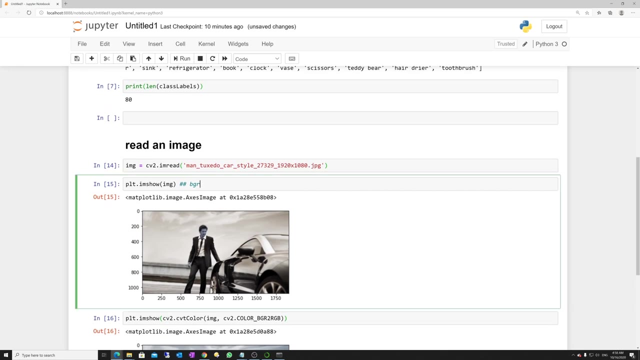 is the by default using C open-cv, right? so if I can word into like this, so you see over here, if I convert into RGB, this is the actual image, right? so these are the thing. like we need to convert BGR to RGB and many other settings we need to. 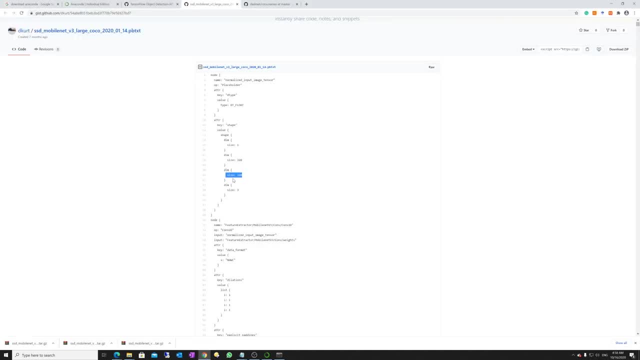 do right and as I showed you that we have a 3, 20, 3- 20 size, right, so this is the configuration we have. we have just loaded. you can see we have a 3, 20, 3- 20 size, right? so this is the configuration we have. we have just loaded. 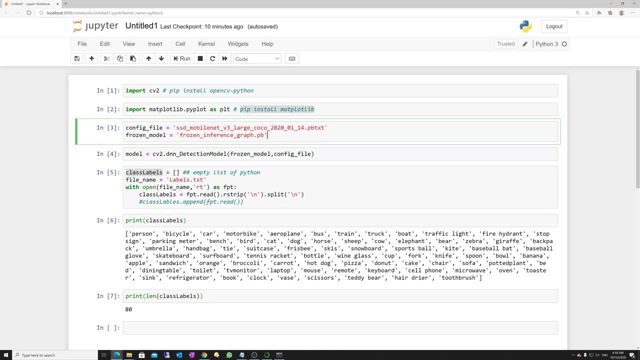 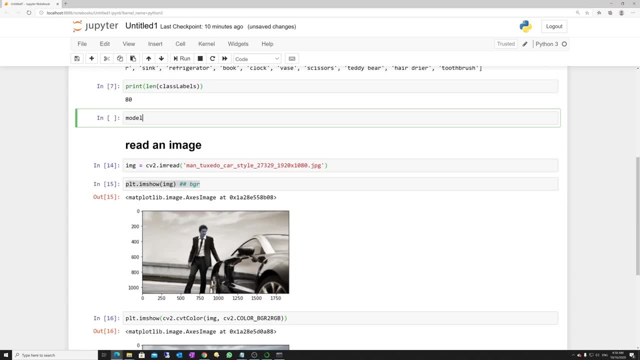 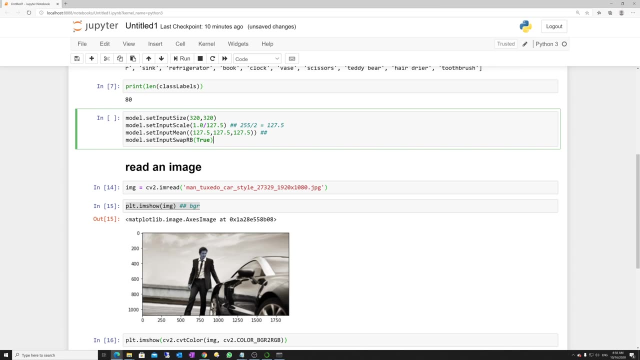 it, right? so this is the configuration we have loaded, you see. so you, this is the configuration. so now the the total configuration. right, if i press model? okay, let me to save my time. okay, so model dot. you need to do like this once you loaded the model, like this, using this command: 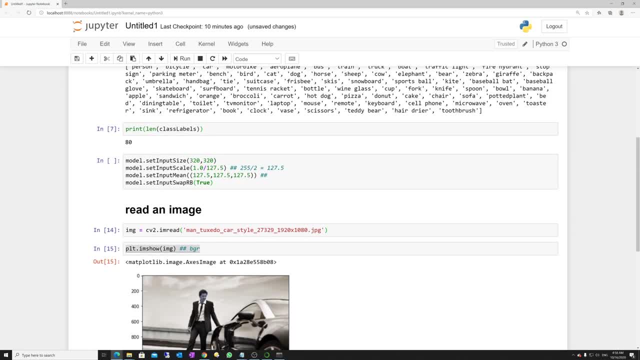 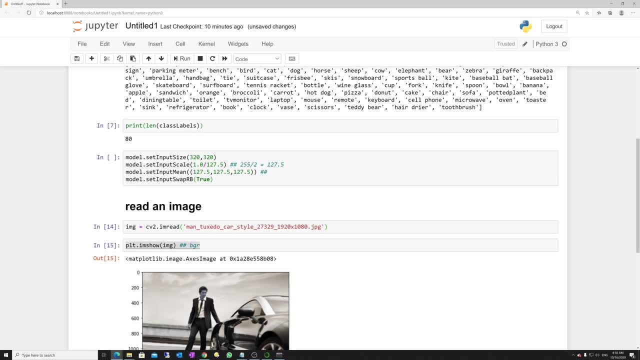 so another thing important: you need to set up the configuration. so input size is 320 by 320 y, because in this configuration file we have defined it's 320 by 320, right. and another thing is that 255 divided by 2, 255 is the gray level for white right. so 0 to 255 is the mostly gray level. so 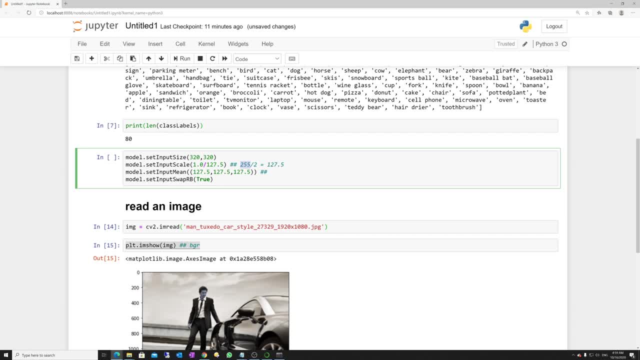 it's, we are converting it to the for scaling. we are doing it right. so another thing is: that is 127.5. we are taking the mean the. why is so? because mobile net, this, this mobile net, uh, takes the input as a minus one into one right. 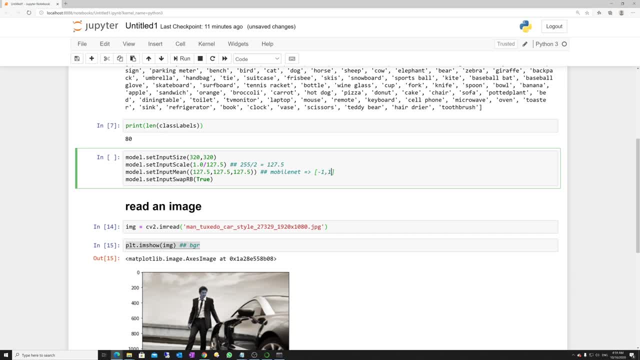 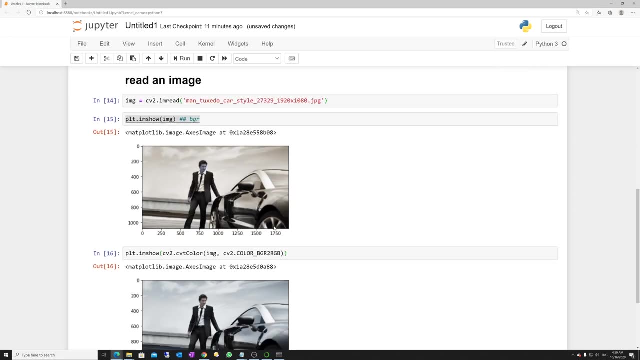 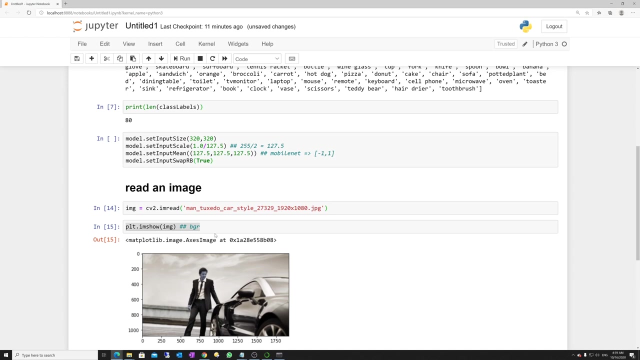 okay, so this is the reason why we are. we are doing it like this, right? so it takes minus one into minus one, right? so you have to take care of the configuration of your architecture. similarly, we have set input swap rb. so, as you see over here, we did like this, like bgr to rgb, so we don't. 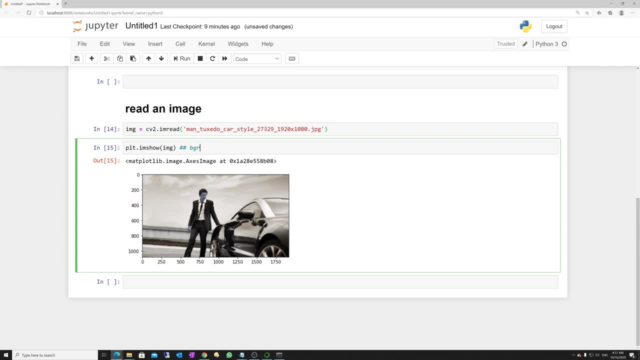 it. so we have gb directory, right, so you can see the gbd directory. it's the gbver ax痛 here, actually. so it's the exist. so i will ender form and i also wanna wait a moment into like this, so you see over here, if i convert it to rgb, this is the actual image, right so? 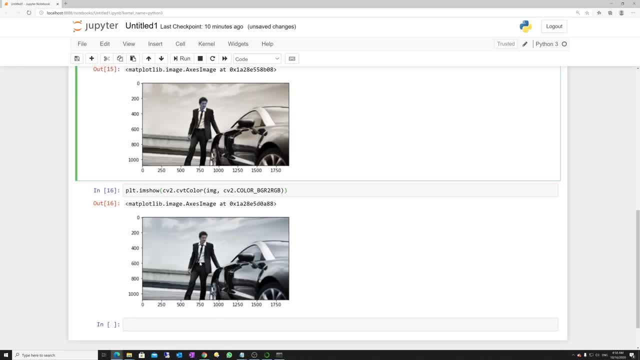 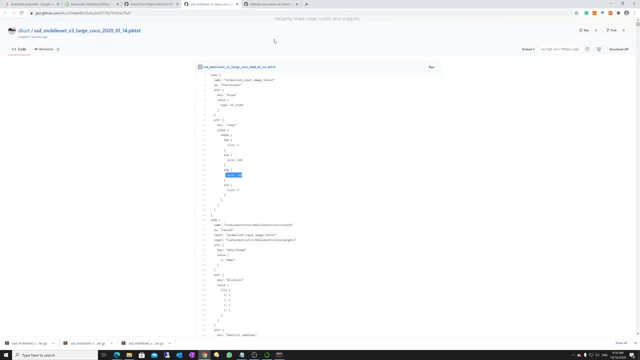 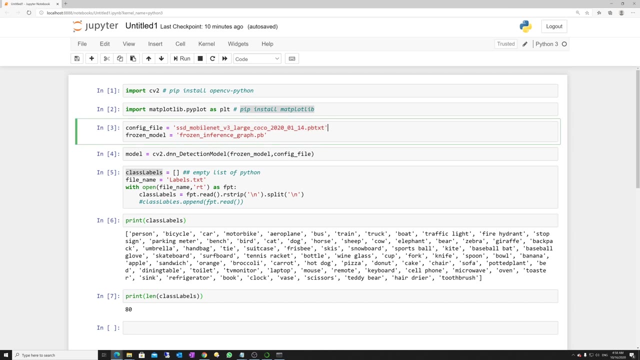 these are the thing, like we need to convert bgr to rgb and many other settings we need to do right and, as i showed you that we have a 320, 320 size, right? so this is the configuration we have, we have just loaded, right? so this is the configuration we have loaded, you see. so you, this is the 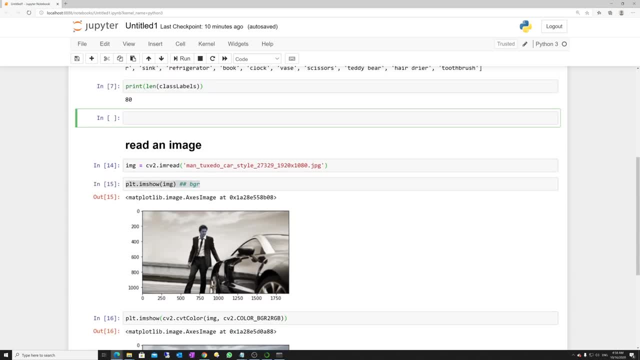 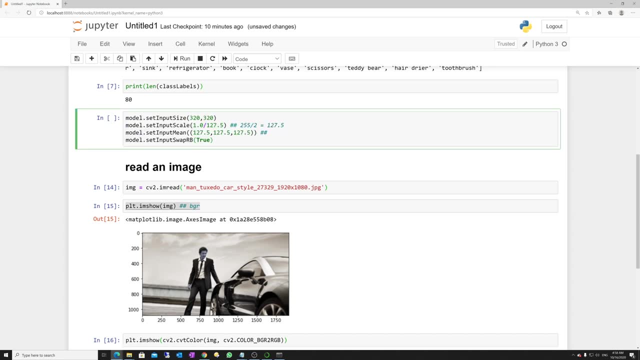 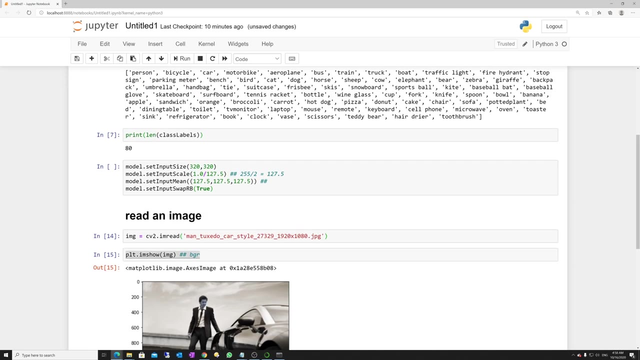 configuration. so now the the total configuration. right, if i press model. okay, let me to save my time. okay. so model dot, you need to do like this, once you loaded the model, like this, using this command. so another thing important: you need to set up the configuration. so input size is 320 by 320 y. 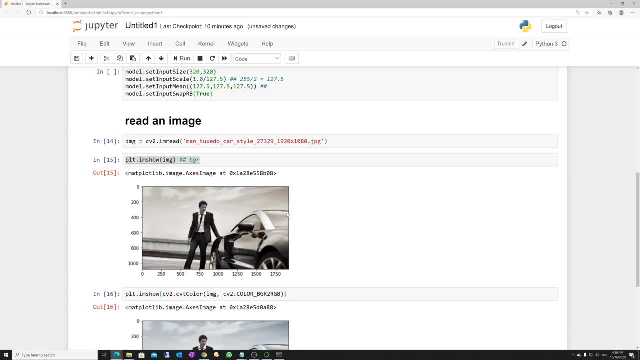 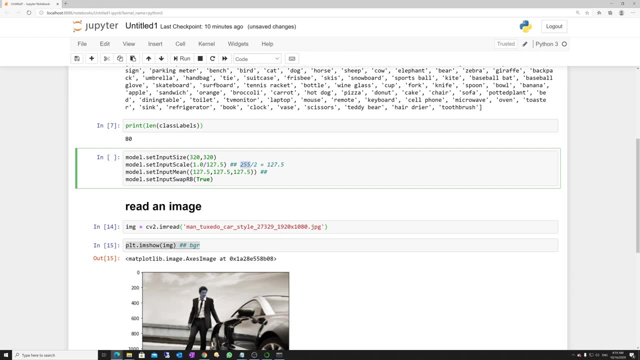 because in this configuration file we have defined it's 320 by 320 right, and another thing is that 255 divided by 2, 255 is the gray level for white right. so 0 to 255 is the mostly gray level. so it's we are converting it to the for scaling, we are doing it right. so another thing is that 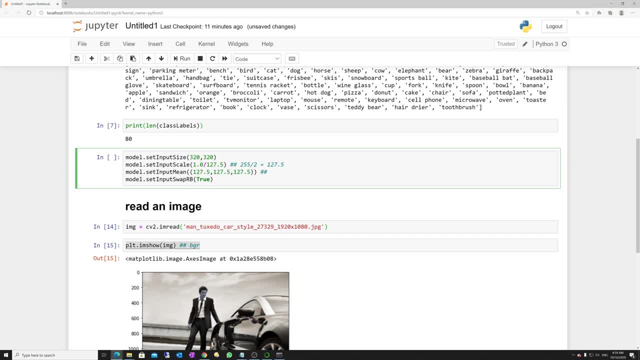 is 127.5. we are taking the mean the. why is so? because mobile net this, this mobile net takes the input as a minus 0-1 x 1, right, okay? so this is the reason why we are doing it right, like this, right, so it takes. 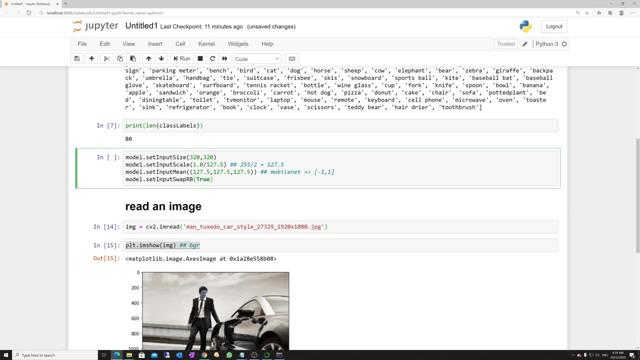 0-1 x 1, right, so you have to care, take care of the configuration of your architecture. similarly, we have set input swap RB. so, as you see over here, we did like this, like bgr to RGB, so we don't need to configure the nature or the. this is just used to. 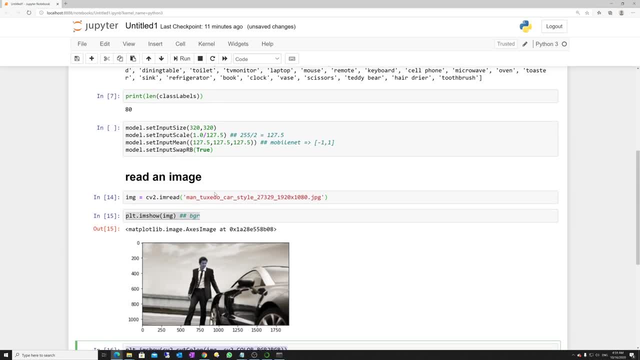 to create the color. then, next step, we are going to write the base for the solid attributes. burgundy, now the base comes under library. you are going to be Menoun ministre on. if you want, you can use the b so we don't need to convert it each time. right, so it should be automatic. so when we did, we did. 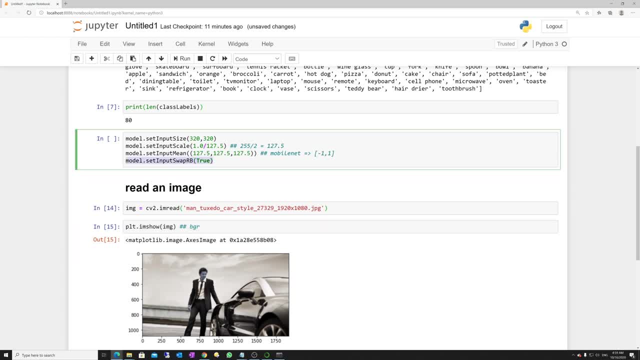 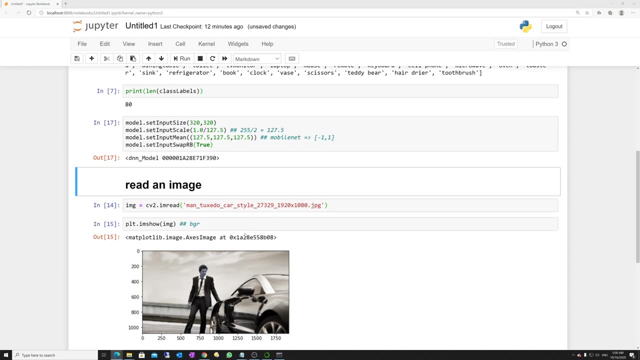 need to convert it each time, right, so it should be automatic. so when we did, we did: uh, swap rb. true, so it will be automatically did by itself. right, it will perform automatically. so now, once we do it- okay, so the most easy thing is okay. so once i have model so i can just 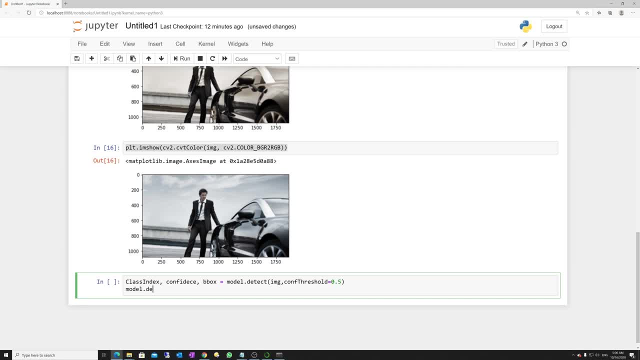 you see, i can just write model dot detect. you see, so if i press the tab it will be automatic, automatically. done right, because i have already loaded the model. so class index conference b box. so this is the three uh output of this and this is the threshold based on your accuracy, you want. 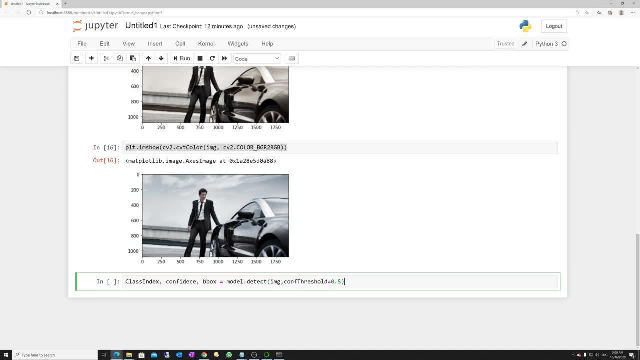 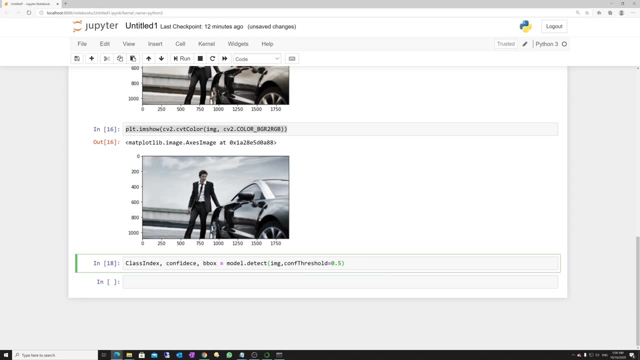 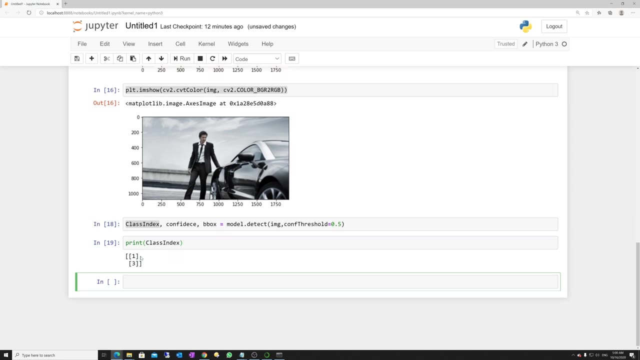 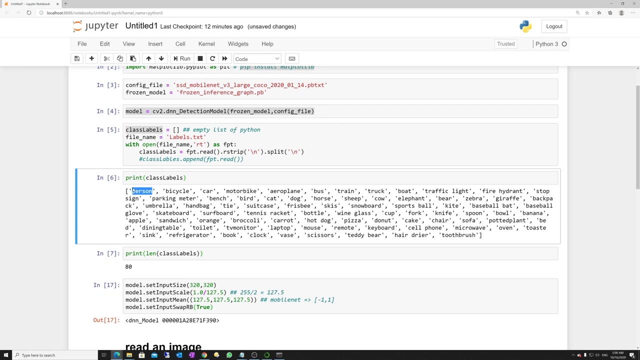 if you want to have more accurate, then you can reduce and you can change it. we have just fixed it for 50 percent confidence, you see. so if i print my class index, so if there are two things like one and three, so what is one and three? so if you see over here, one is actually. if i start from zero, 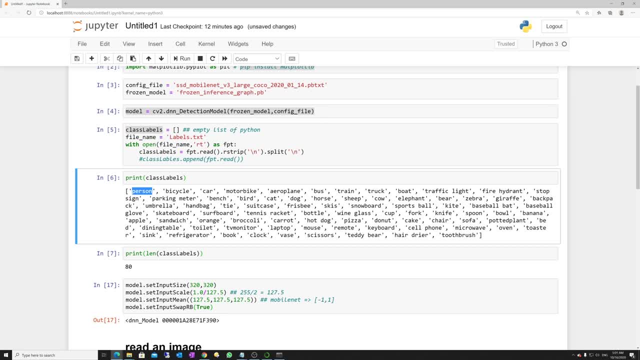 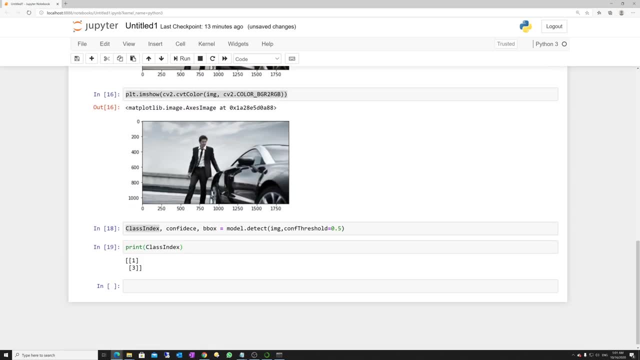 it is one. so i will reduce minus one. i will show you. but this is one and this is three, right, so one is person and one is car. so you see we have two labels: one is person, one is car, right, so it's successfully detect. so if i check, uh, you see over here it is not flattened. so in order to do it so, 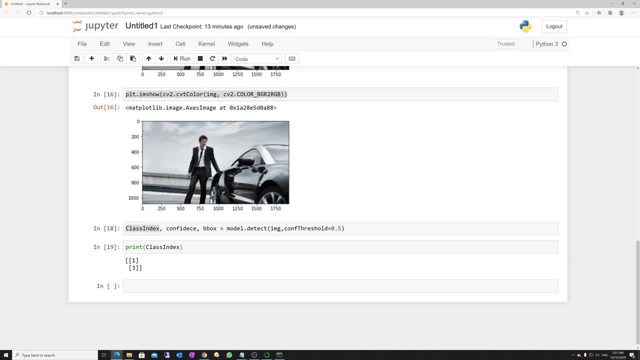 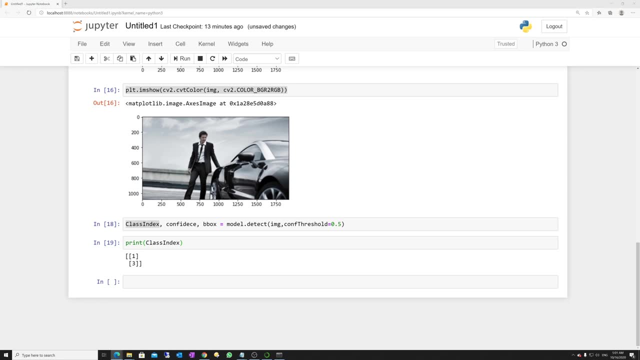 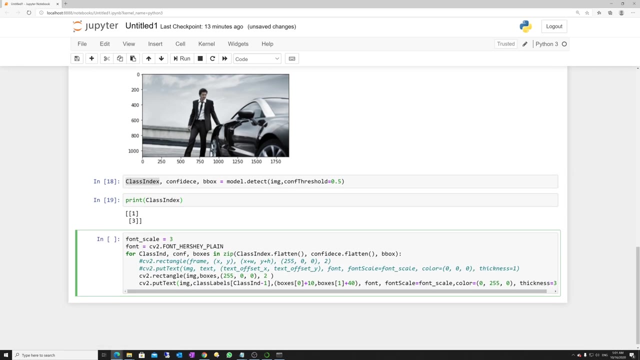 we can, just we need to flatten everything right, so we, you can see over here, we have two lists right, so we have to flatten before doing it. so okay, so this is the code for like, for example, i'm setting my font uh, like, uh, what is my font size? 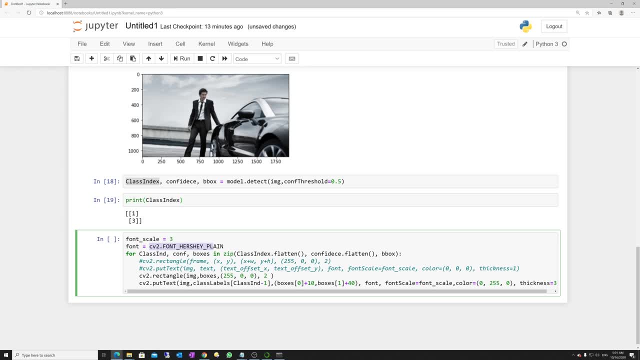 and what is my font type. and then i need to have a loop like class index, confer, conference boxes in zip. so, uh, if we have three different uh folders- sorry, three different variables- we need to do zip and everything. i'm flattening my because there are double braces, right, so that is why i'm 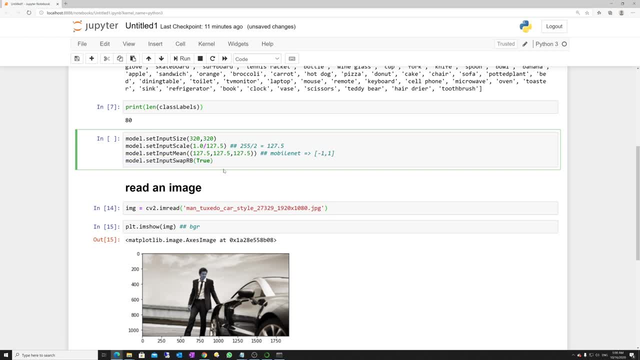 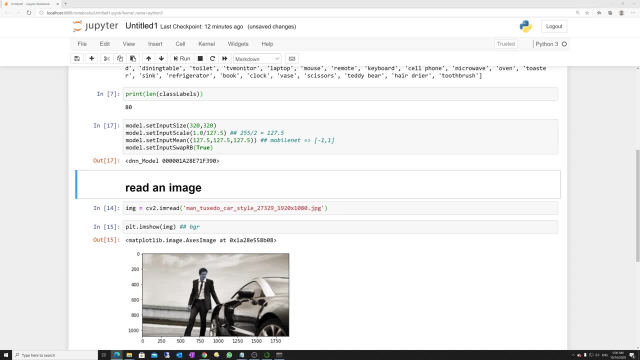 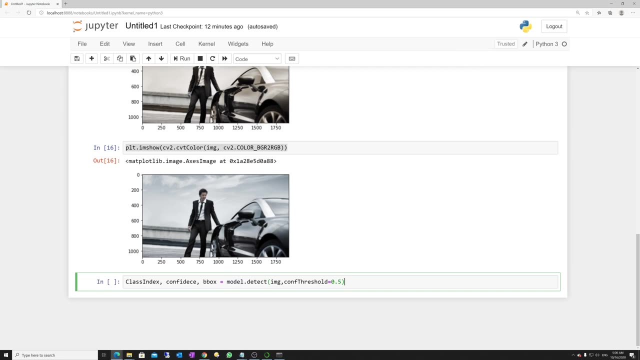 swap rb. true, so it will be automatically did by itself. right, it will perform automatically. so now, once we do it, okay, so the most easy thing is okay. so, once i have model, so i can just, you see, i can just write model dot detect. you see, so if i press the tab it will be automatically done. 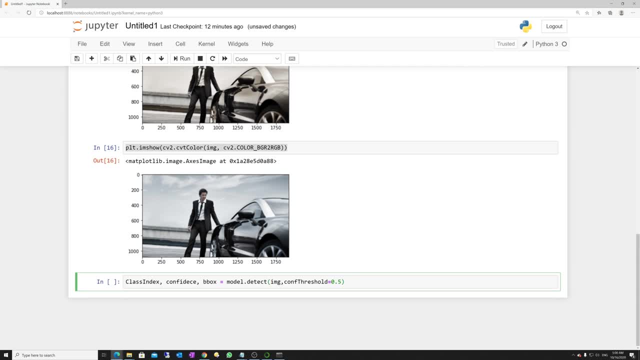 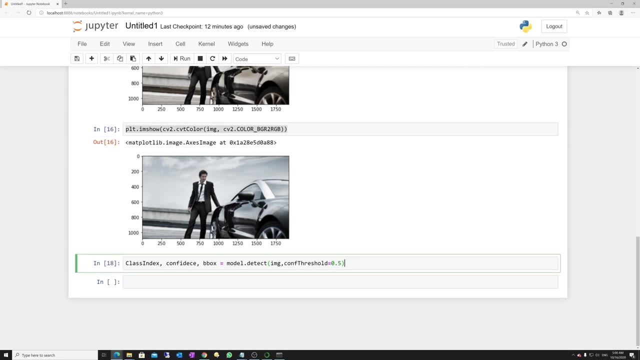 right because i have already loaded the model. so class index conference b box. so this is the three output of this and this is the threshold based on your accuracy you want. if you want to have more accurate, then you can reduce and you can change it. we have just fixed it for 50 confidence, you see. 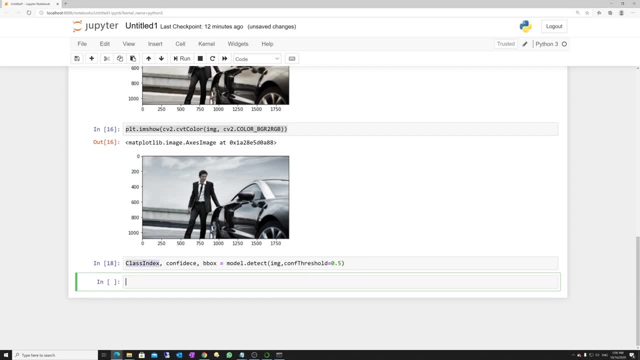 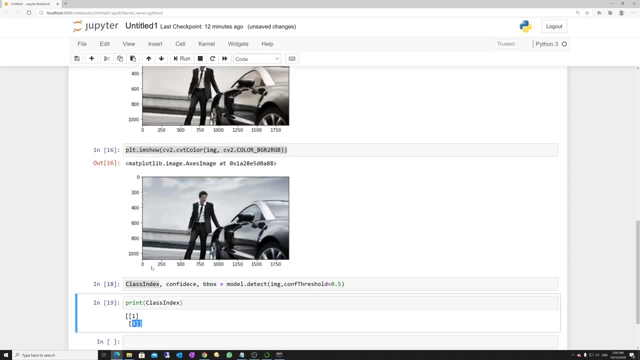 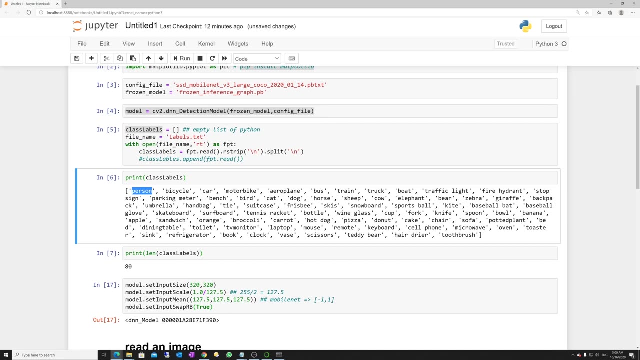 so if i print my class index after you text your class index, so there are two things like 1 and 3. so what is 1 and 3? so if you see over here, one is actually: if i start from 0, uh, it is 1, so i will reduce minus 1, i will show you. but this is 1 and this. 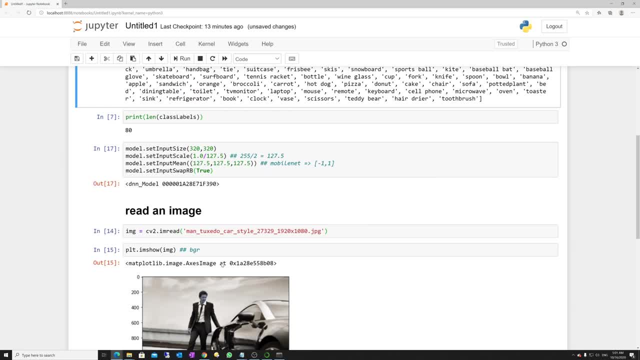 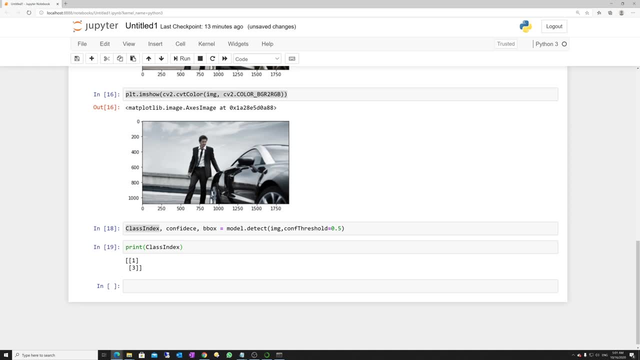 is 3, right, so one is person and one is car. so you see we have two labels: one is person, one is car, right, so it successfully did that. so i check. uh, you see, over here it is not flattened. so, in order to do it, so we can, just we need to. 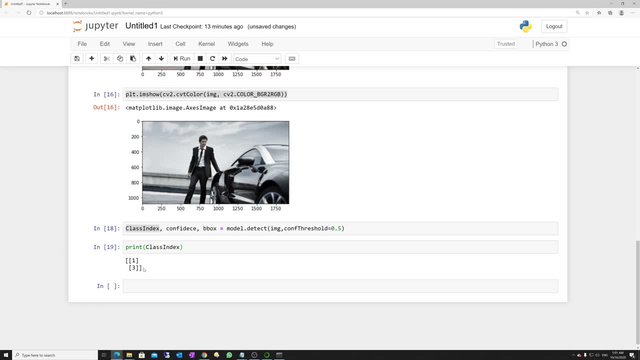 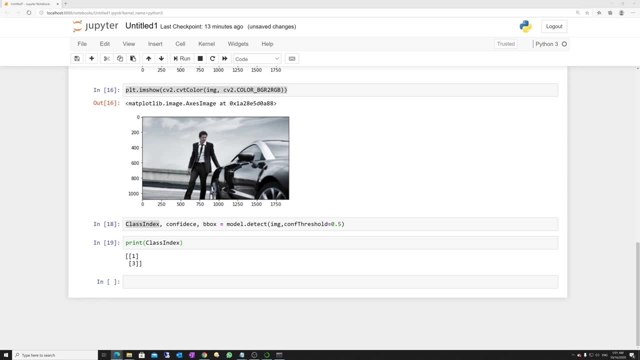 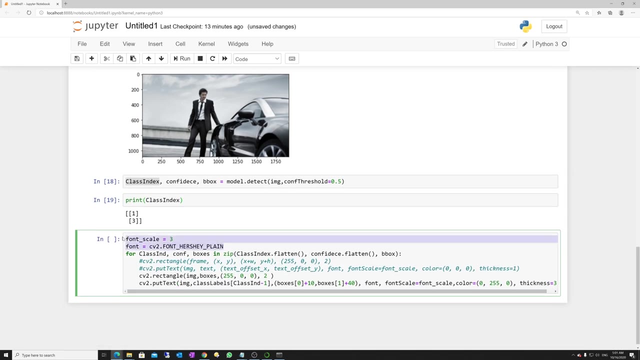 flatten, right, so we- you can see over here, we have two lists, right, so we have to flatten before doing it. so okay, so this is the code for like: for example, i'm setting my font like what is my font size and what is my font type, and then i need to have a loop like class index config. 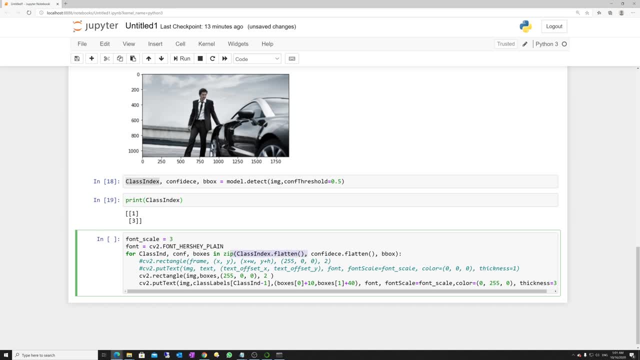 conference boxes in zip. so, uh, if we have three different uh folders, sorry, three different variables, we need to do zip and everything i'm flatting. why? because they are com double braces, right. so that is why i'm doing it for flatten for b box. it's not, that is for people. 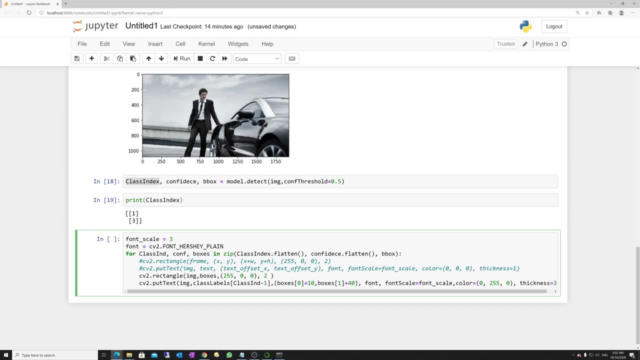 doing it for flatter, for b box. it's not, that is for for the box. we are not doing it and we can have different. uh, like cv2.rectangle means that plot this box having our bgr right blue, so the blue and this is the scale. and similarly we have put text like: this is my text, whatever i write. 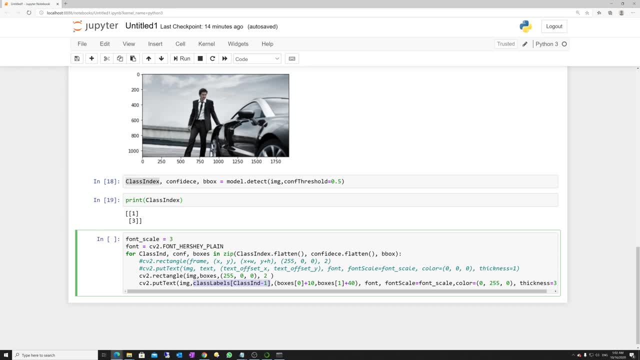 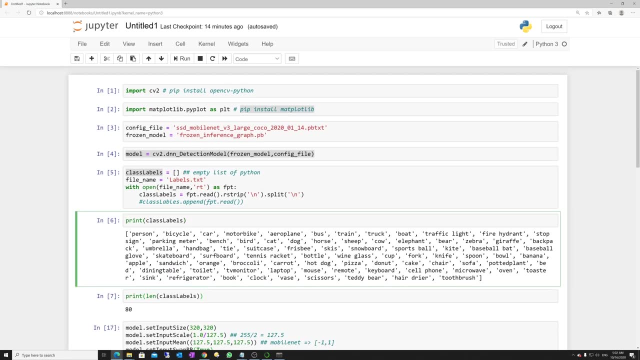 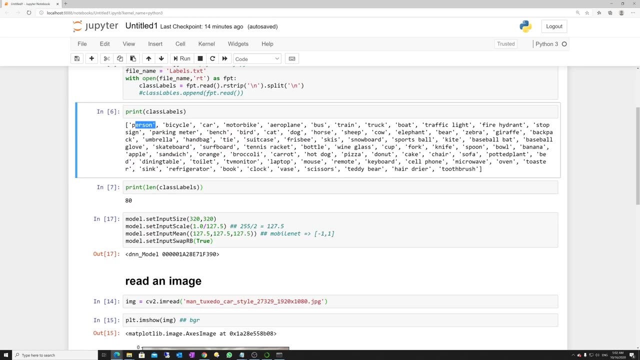 over here. it will be displayed over here. so the class index, the class label: we have class labels, right? we have 80 class labels. you see, in the class labels we have this. so we want to display this one right, but it is at zeroth index, as you can see over here. there is a offset of one over here to. 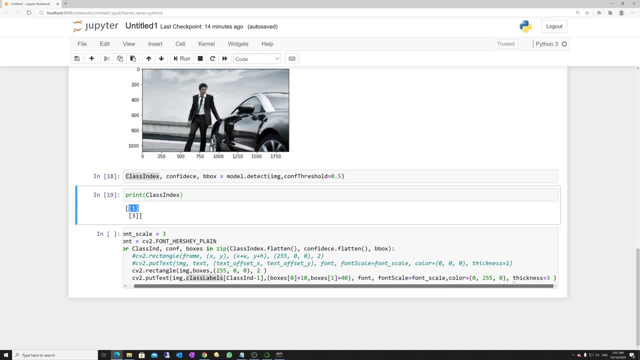 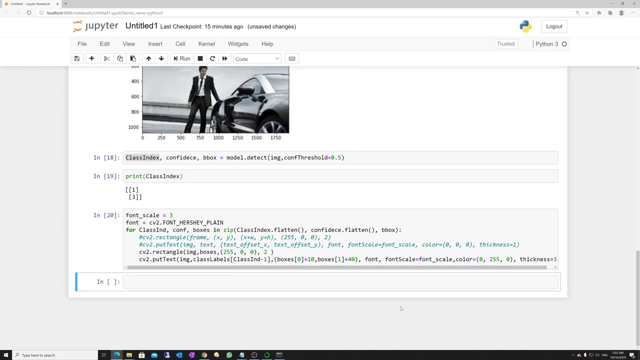 see. so i need to reduce minus one wire. so once i execute this command and similarly, the font color is 055, so bgr. so font color is green and bgr and the rectangle color is blue. so if i shift, enter and execute it and then i need to plot again. 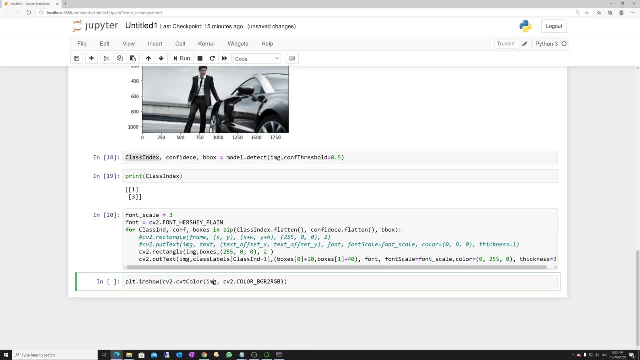 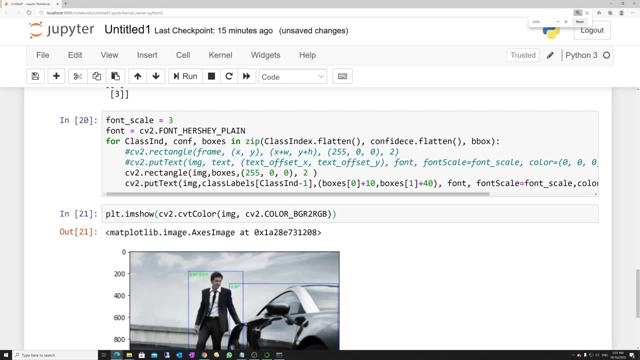 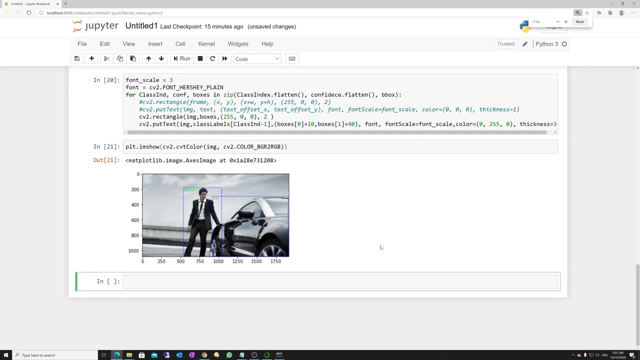 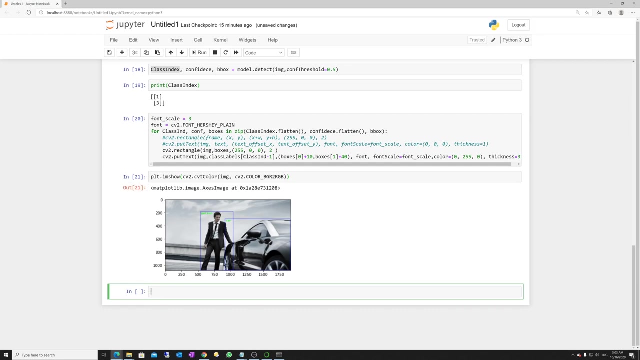 let me plot again my image right. so i have modified my image, you see. now you can see over here that it has detected the person and the car right, so very efficiently. it detected the person and car. now, as we can process one image at a time, now it's time to go for the video demo, right, in order to 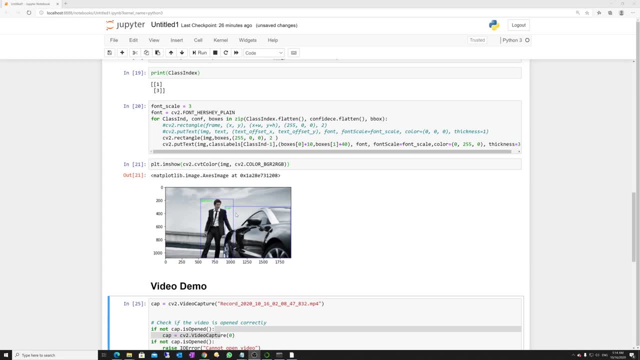 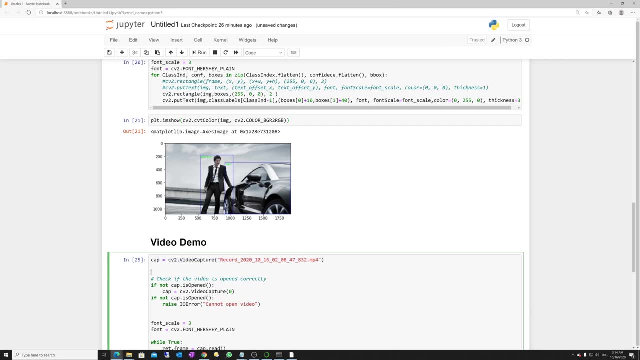 deploy this code for the object detection. in case of the video, all you need is to just write this code, like cv2.video capture, so it will just load this mp4 video file, so it mostly support mp4 and other formats. you need to check and once you do it, you need to write. 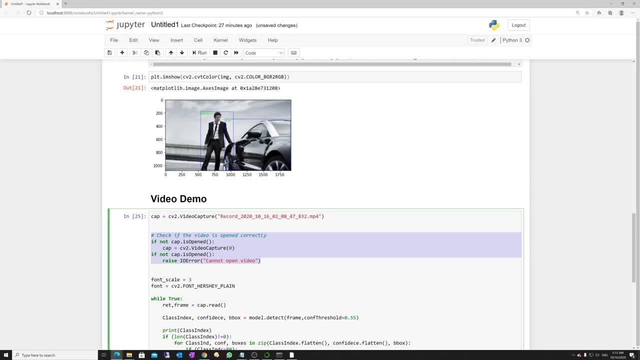 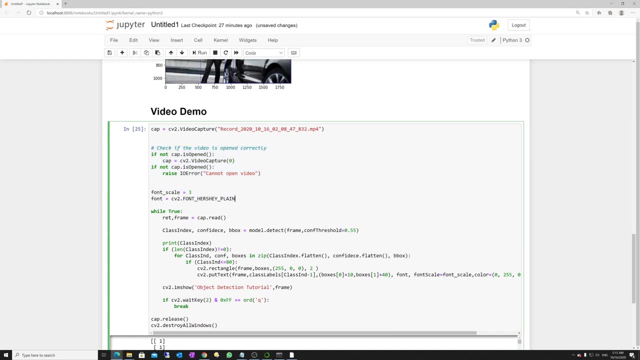 this code, for example, if it is corrupted or you cannot open the video. so these are the commands. and, similarly, this is the same like for scaling my font, and this is the type of my font, and you can do it while true, like one, but you can do it until end of that as well. but right now for the simplicity. 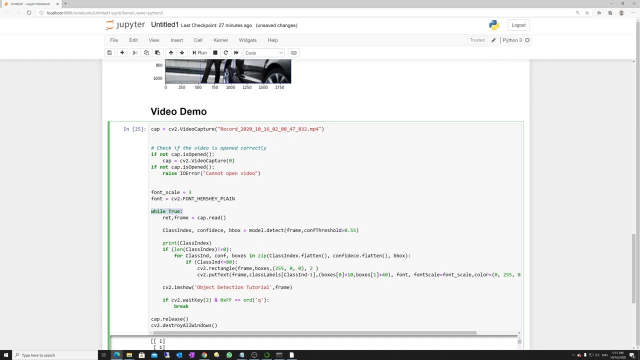 i'm having infinite loop. so what is this? like cap, uh, cv2.video capture is a file pointer to this video, like it will be pointing the foot to the first image of this video. so the video video is nothing, but it's the combination of the images, right? so usually we have, on average, 25 frames per second. 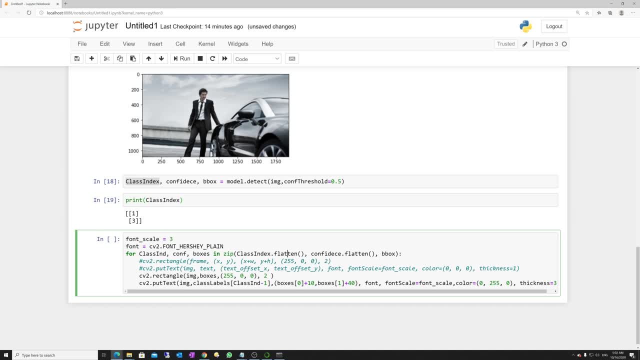 for the box. we are not doing it and we can have different. uh, like, cv2.rectangle means that plot this box having r, g, bgr, right, blue. so the rectangle color will be blue and this is the scale. and similarly, we have put text like: this is my text. whatever i write over here, it will be displayed over here. so the class index, the class. 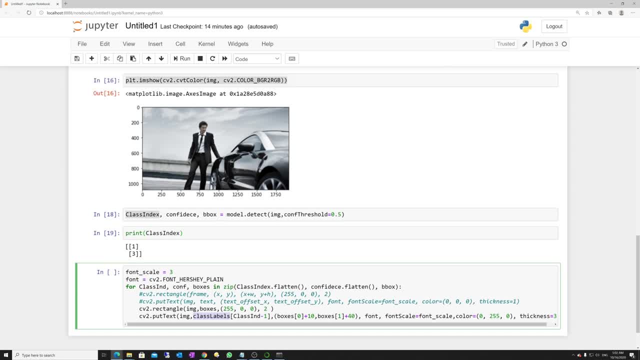 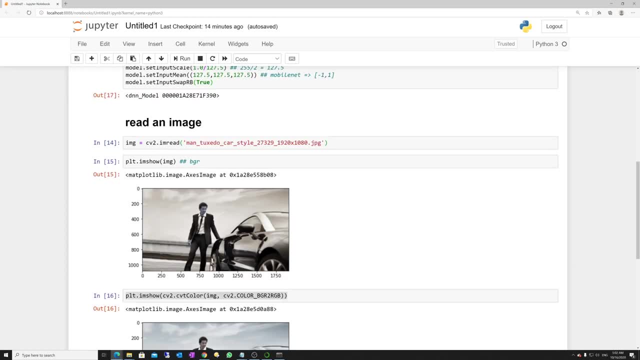 label. we have class labels, right, we have 80 class labels. you see, in the class levels we have this, so we want to display this one right, but it is at zeroth index, as you can see over here. there is a offset of one over here to see. 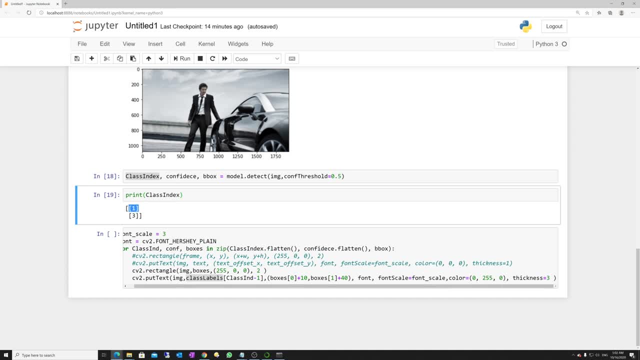 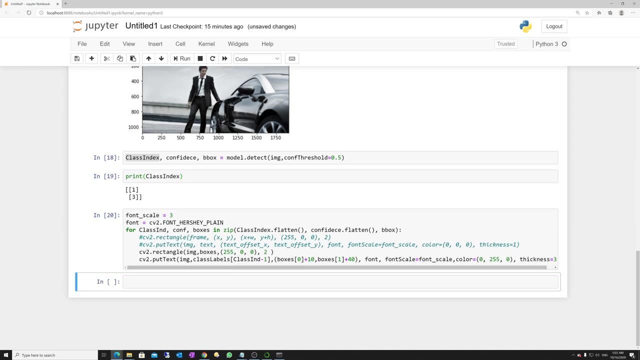 so i need to reduce minus one wire. so once i execute this command and similarly, the font color is 055, so bgr. so font color is green and bgr and the rectangle color is blue. so if i shift, enter and execute it and then i need to plot again, 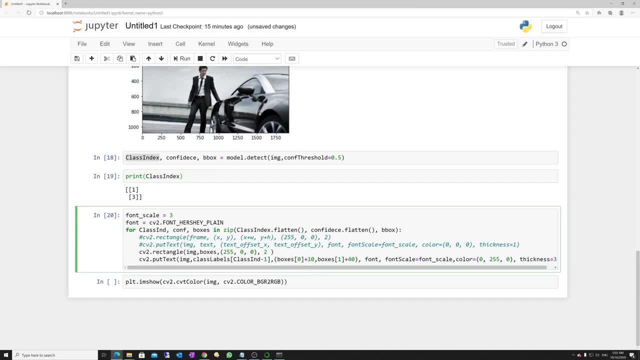 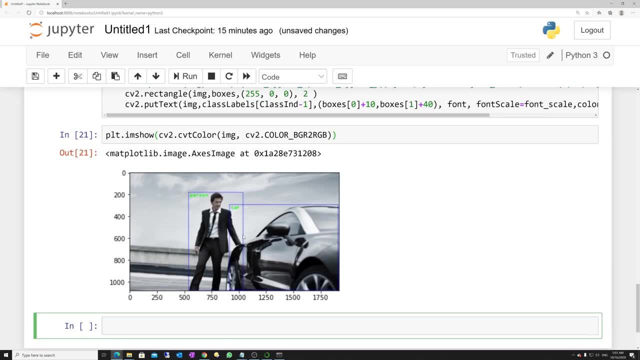 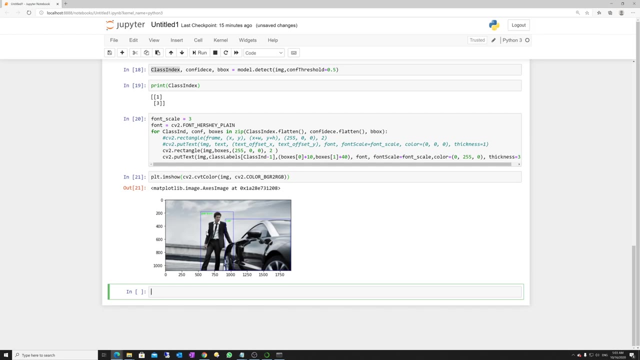 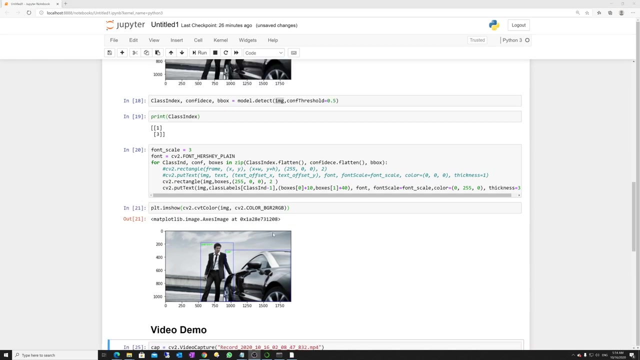 let me plot again my image right. so i have modified my image, you see. now you can see over here that it has detected the person and the car right, so very efficiently. it detected the person and car. now, as we can process one image at a time, now it's time to go for the uh video demo right, in order to deploy. 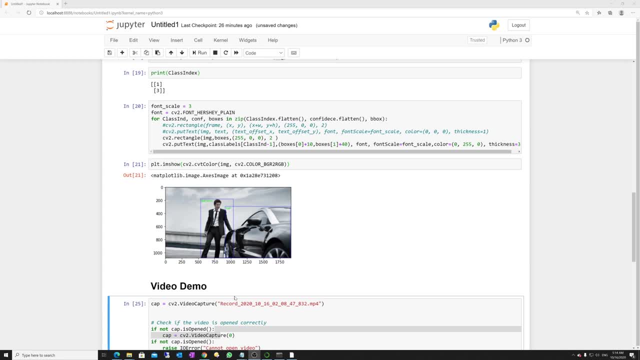 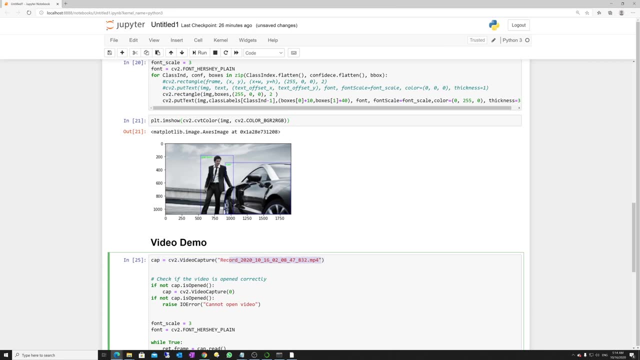 this code, uh for the object detection. in case of the video, all you need is to just write this code like cv2.video capture, so it will just load this uh mp4 video file, so it mostly support mp4 and other formats. you need to check and once you do it, you need to write this code. for example, if it 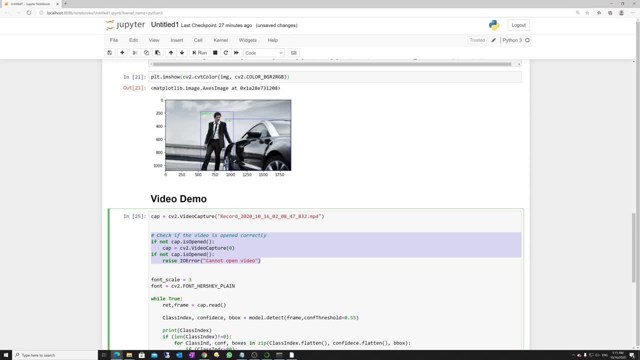 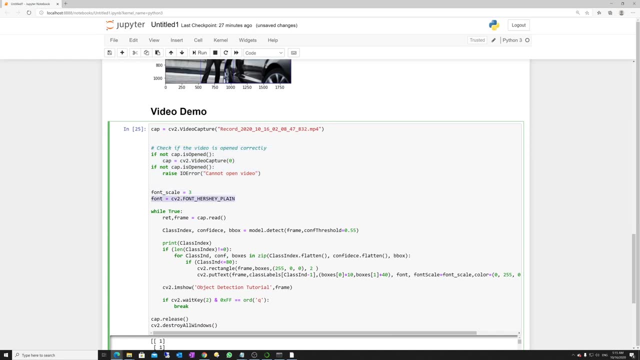 is corrupted or you cannot open the video. so these are the commands and, similarly, this is the same like for scaling my font, and this is the type of my font, and you can do it while, true, like uh one, but you can do it until end of that as well. but right now, for the simplicity i'm having, 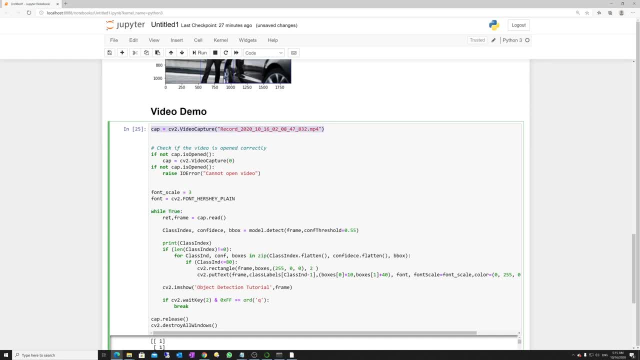 infinite loop. so what is this? like cap, uh, cv2.video capture is a file pointer to this video, like it will be pointing the fo to the first image of this video. so the video video is nothing, but it's the combination of the images, right, so usually. 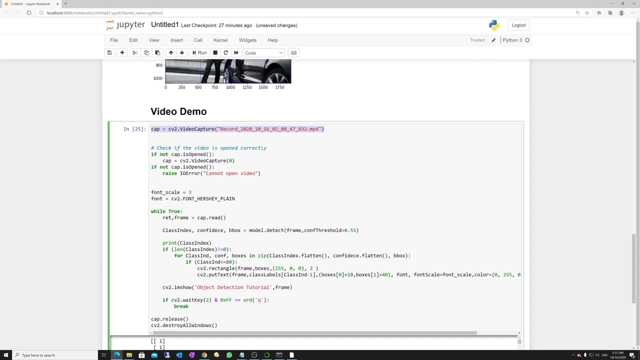 we have on average 25 frames per second right, and for high resolution videos, like 4k and others, we have 60 frames per second right. so video is nothing but a combination of images. so we are reading capread, okay, so now, then we will have image in it, right? so, as you can see over here, 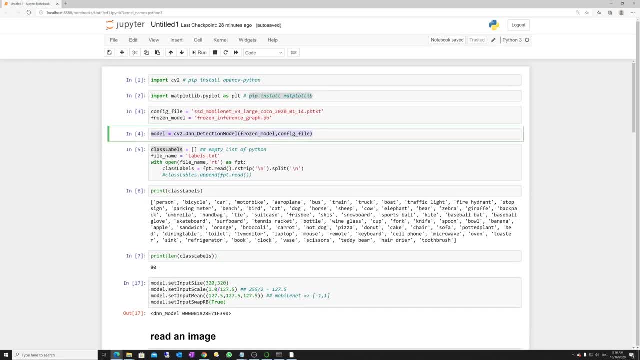 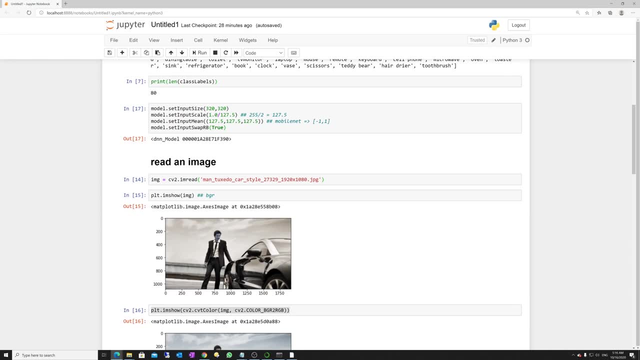 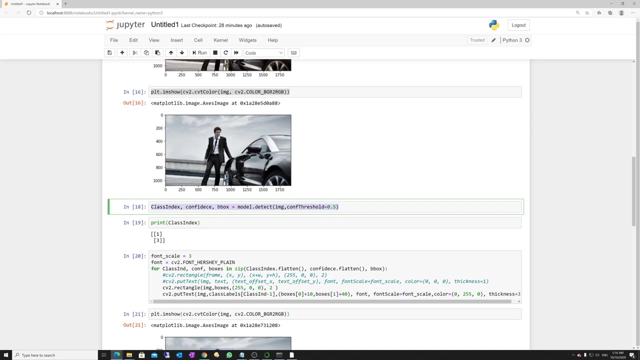 previously. we just have loaded the, our model based on our configurations, and the frozen graph right, and we do have all the labels as well. so all the settings we have put before that. and now, if we write this command right- modeldetect- so i have executed already these commands, so that is why i'm not doing it. 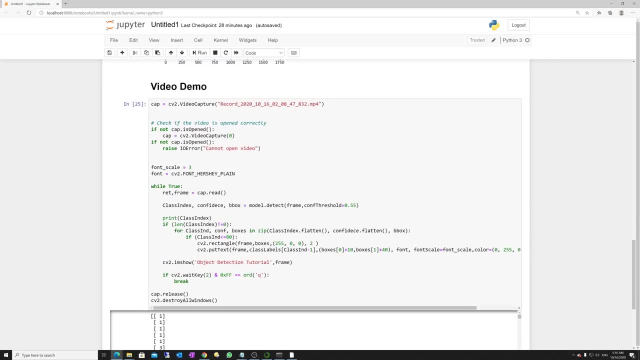 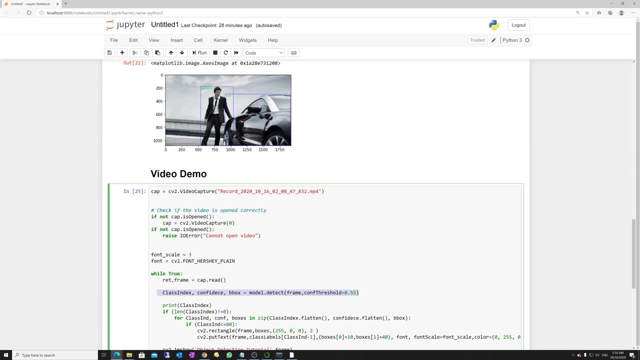 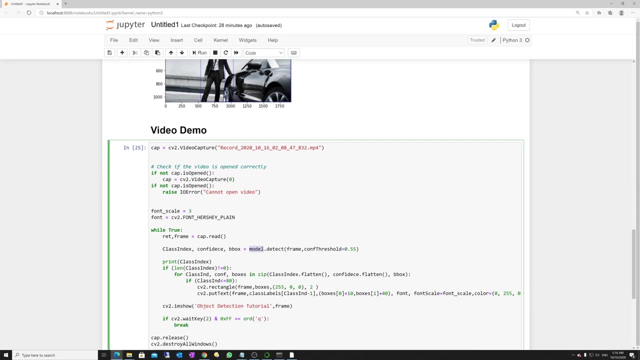 again. so all i need this command. okay, so i'm just doing it right. so in your case, if, for example, if you haven't executed previous commands, you need to do it right, because model will not be saved in your case, so you need to execute these commands. so i assume that you've already executed all previous. 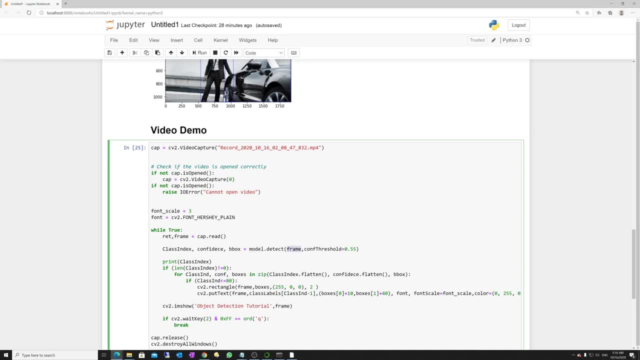 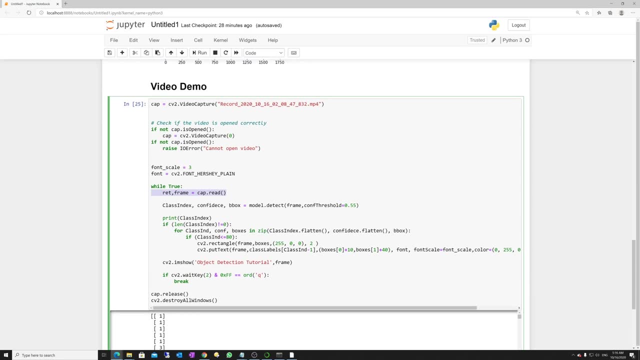 commands, so modeldetect. now, in this case, rather than image, i should have frame, so frame by frame, the video. and then, for example, in this case: uh, we need to make sure that it must not be uh zero, right, so there must be a frame in it, right? so we are double checking over here and over here. 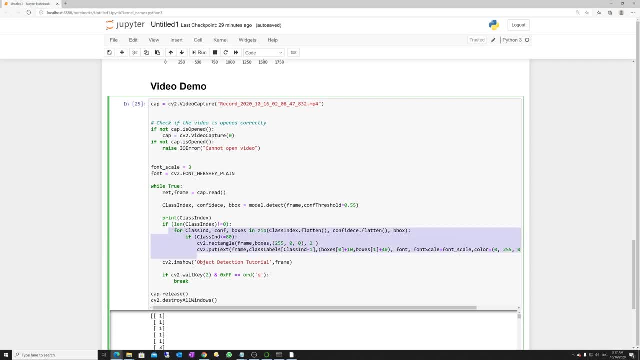 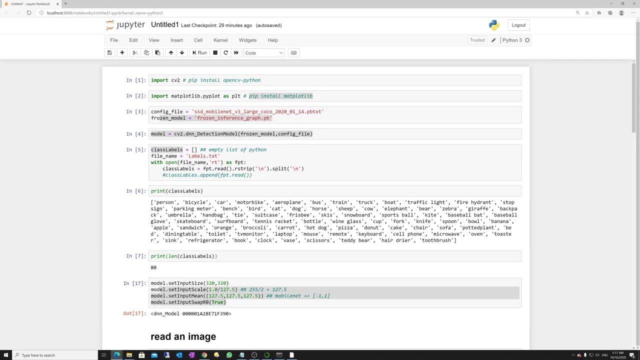 as well. so now this is the previous code. okay, but one more extra con condition i have just put, because sometimes it gives you an error or it more than 80 classes and other things. so make sure that class label must be 80, because we have only 80 classes, right? so we have only 80 classes. so i'm just, uh, in order to 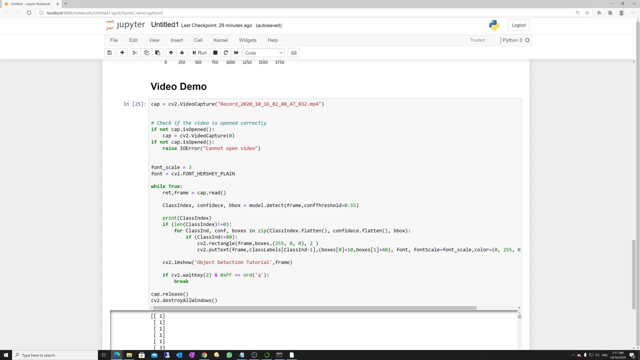 avoid crash the video. so that is why, and again, similarly, the color of my rectangles are blue and the color of my text, that is green. right so, bgr, bgr, right. so now, if i execute this, so this is the video, i'm just doing it. let me show you the video first. okay, so this is the video. 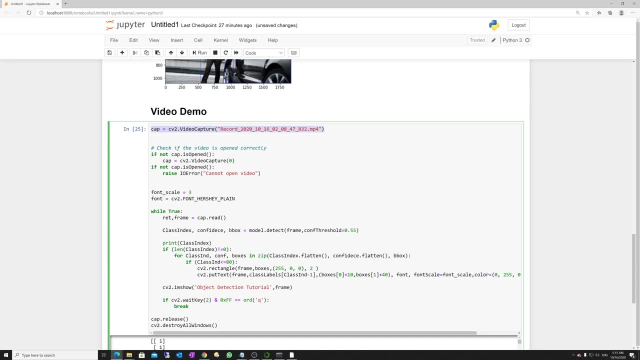 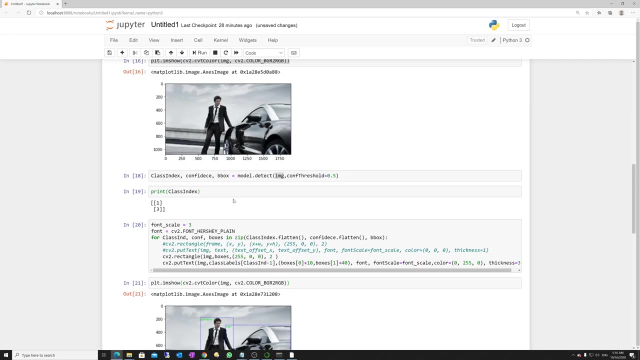 right, and for high resolution videos like 4k and others, we have 60 frames per second right. so video is nothing but a combination of images. so we are reading capread, okay, so now, then we will have image in it, right? so, as you can see over here, uh, previously. 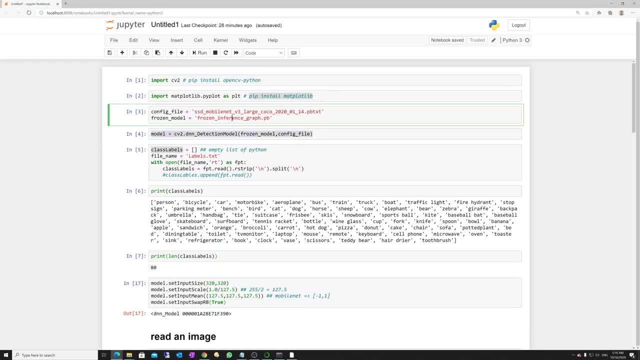 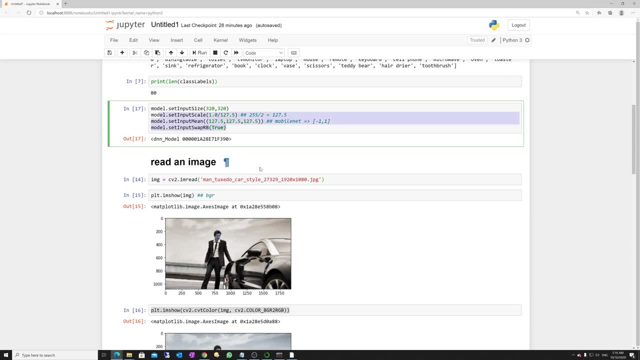 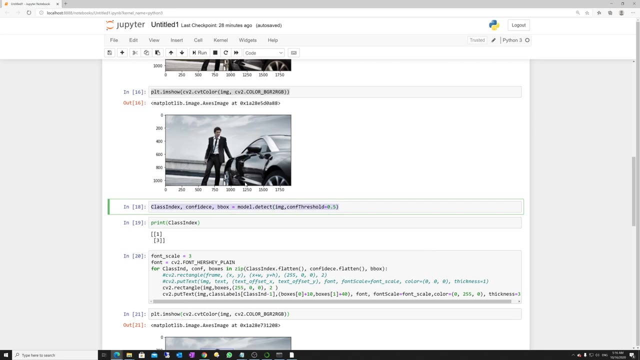 we just have loaded the, our model based on our configurations, and the frozen graph right, and we do have all the labels as well, so all the settings we have put before that. and now, if we write this command right, modeldetect. so i have executed already these commands, so that is why i'm not. 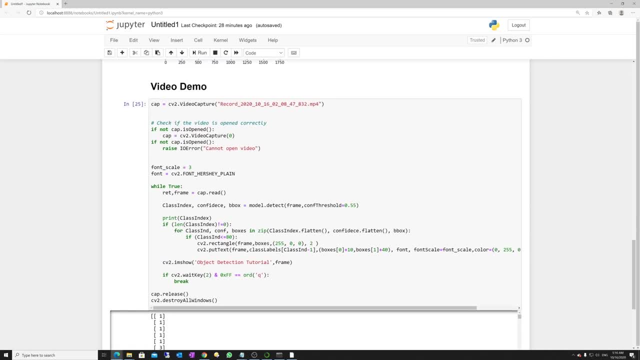 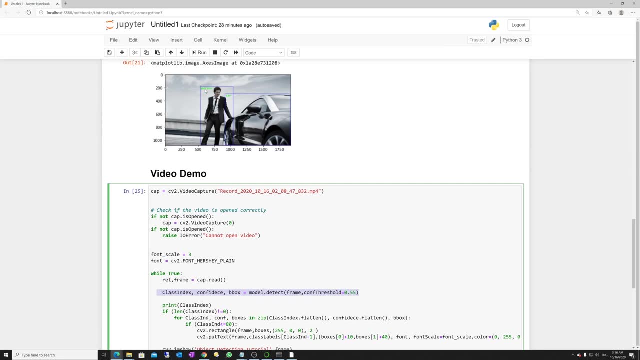 doing it again. so all i need this command. okay, so i'm just doing it right. so in your case, if, for example, if you haven't executed previous commands, you need to do it right, because model uh will not be saved in your case, so you need to execute these commands. so i assume that you have already. 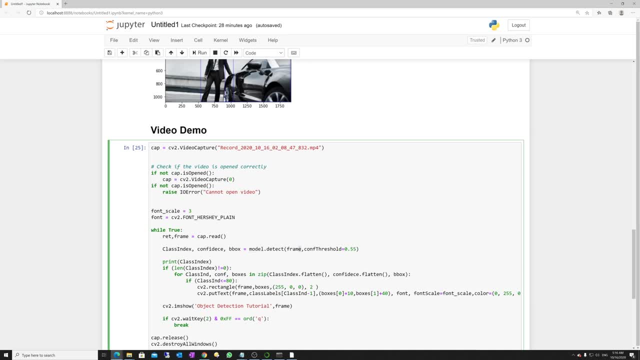 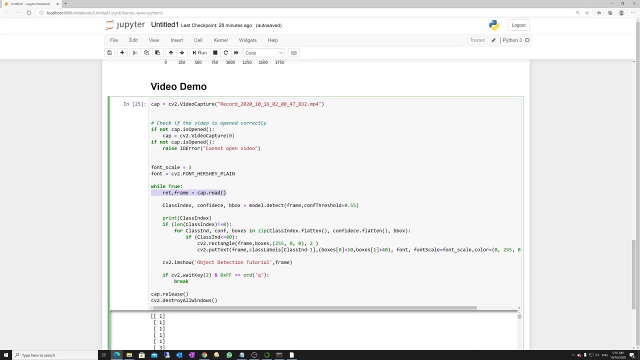 executed all previous commands. so modeldetect. now, in this case, rather than image, i should have frame. so, frame by frame, we are reading the video and then, for example, in this case, uh, we need to make sure that it must not be uh, zero, right, so there must be a frame in it, right? so we are double checking. 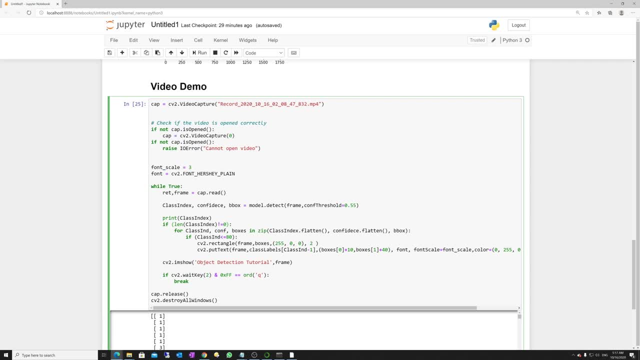 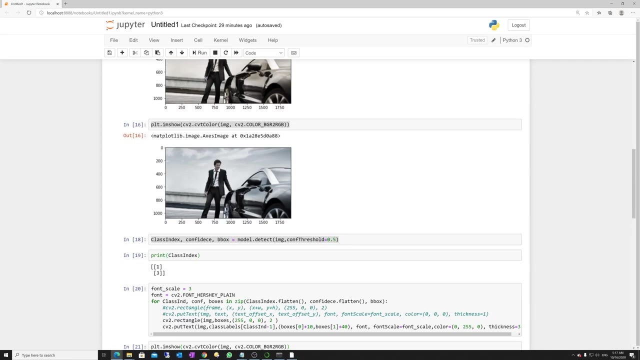 over here and over here as well. so now this is the previous code. okay, but one more extra con condition i have just put, because sometimes it gives you an error or it more than 80 classes and other things. so make sure that class label must be 80, because we have only 80 classes, right. 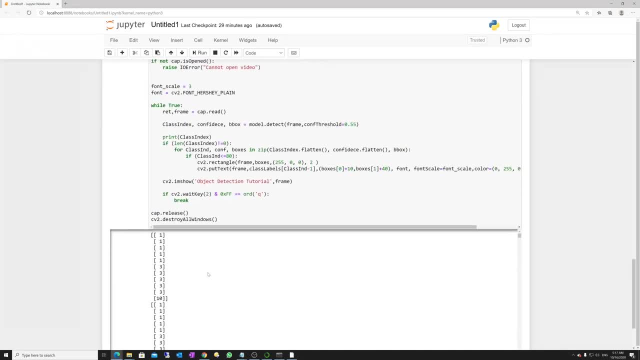 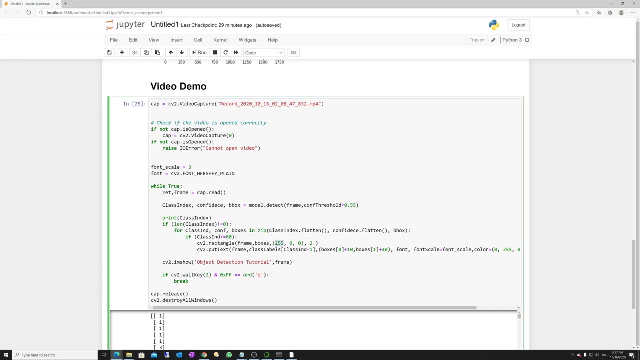 so we have only 80 classes. so i'm just, uh, in order to avoid crash the video, so that is why, and again, similarly, the color of my rectangles are blue and the color of my text, that is green, right, so bgr, bgr, right. so now, if i execute this, so this is the video, i'm just doing it. let me show you the video first. 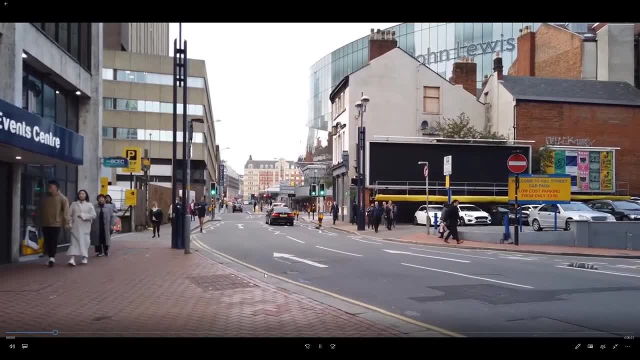 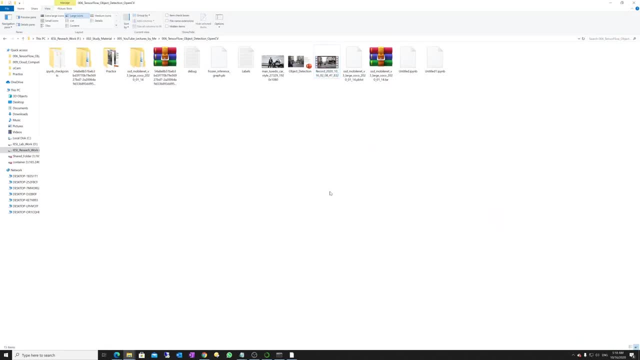 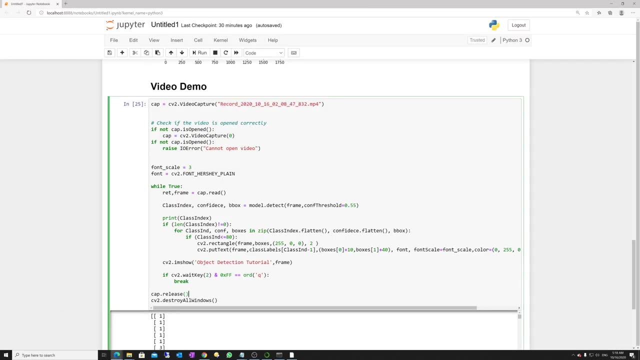 okay, so this is the video. right, as you can see, i have just uh recorded this video from youtube. okay, so you can just record your video as well from youtube or anywhere, and even if you do have your own video, you can just process it. so, if i execute this command, 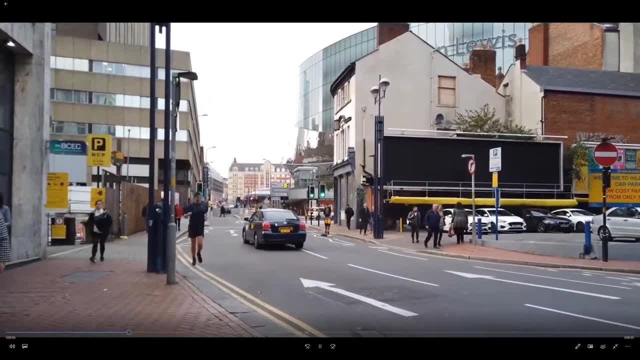 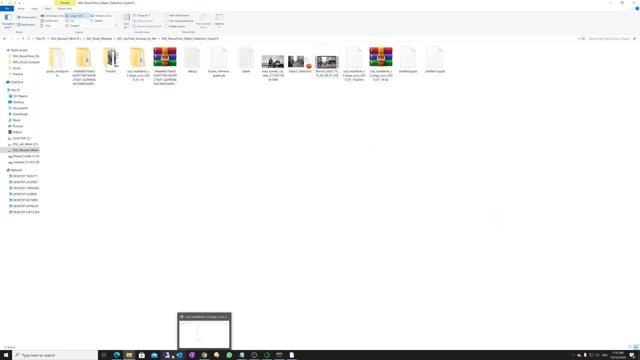 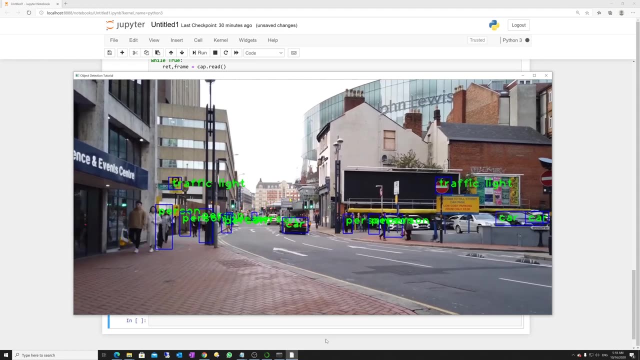 right, as you can see, i have just uh, recorded this video from youtube. okay, so you can just record your video as well from youtube or anywhere, and even if you do have your own video, you can just process it. so if i execute this command, you see over here, this is the same video, the same person, which was 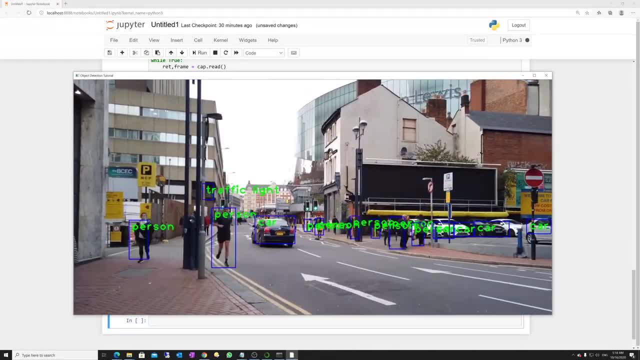 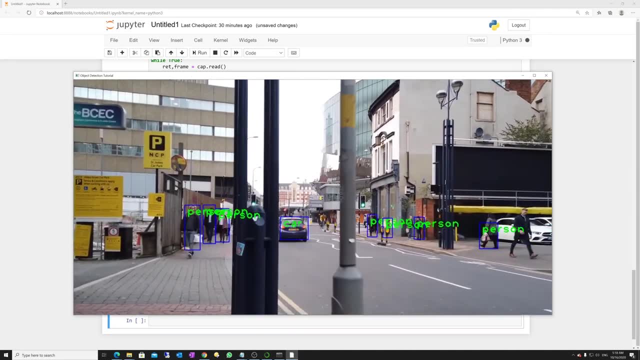 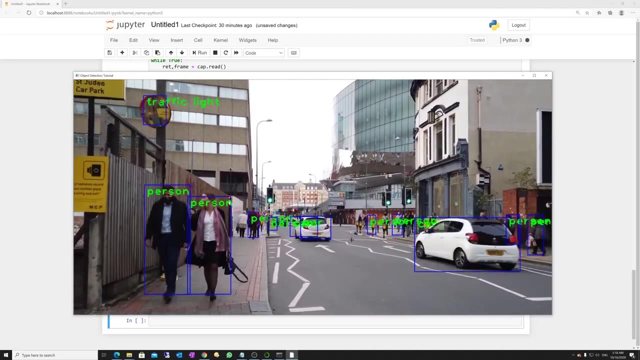 coming right now. so over here you can see that in the start i showed you this video, so uh as well. so you can see that in the first part this video was done by a person, and then we did this. the second part was all done by a person- a person, car and all others- and it is. 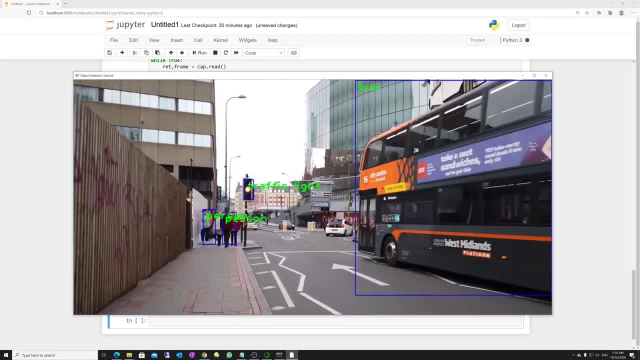 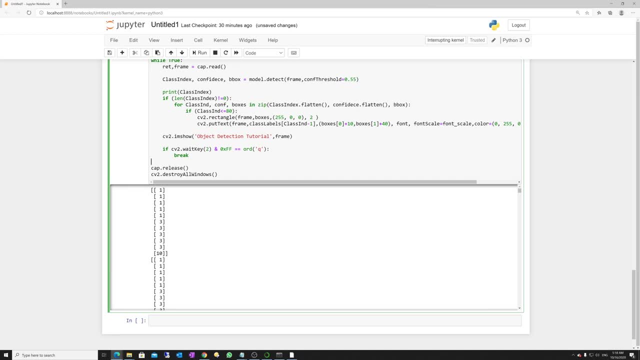 uh, doing it like. uh, right, so we have a wild one, so it should not be wild one, but anyways, it is perfectly working, right. so the same code we just run so you can download it. you see that when the bus comes, it is detecting the bus and the car comes, it just it is detecting the car. so now it's. 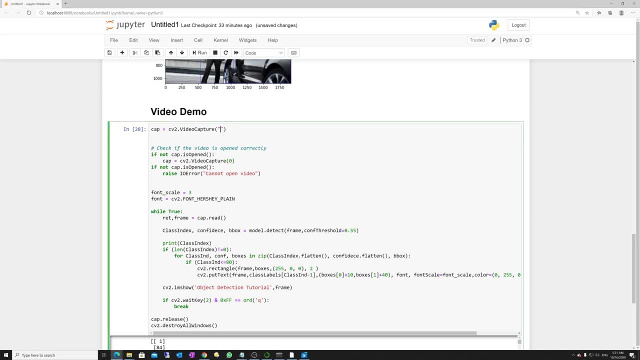 demo. it's better that you just, for example, you modify the previous code into one right. so in my case, i have only one webcam. so based on the number of the webcams you have, so you can change this code. but it's dynamic: one right, the code is very dynamic, so it is finding zero or one. uh, this is. 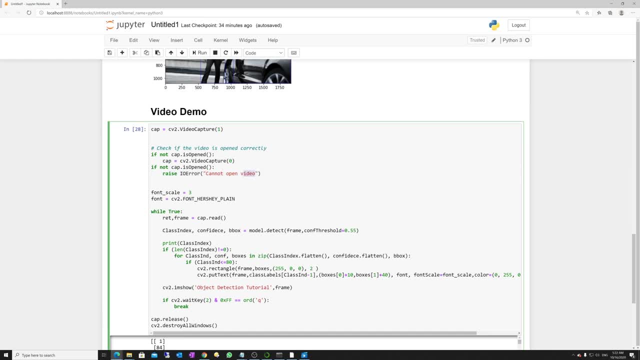 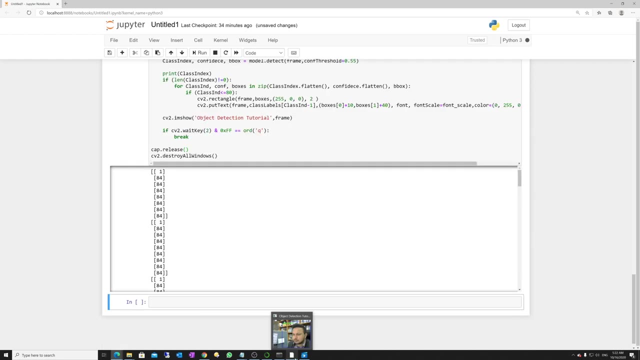 for example, this is webcam, so all you need is just change just. this is just my error instruction. so the most important one was that you need to change it to one right. so once you do do change it to one, the rest of the code is same. if you execute it, you see, it can successfully detect the person and 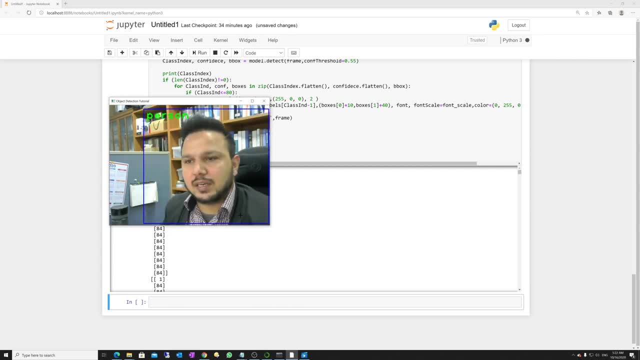 if i move, you see if i move, so it can detect it as well. so it's real-time demo. in your case, i assume that you might have other objects as well, so you can just try it using multiple objects in your using your webcam and you can just deploy. 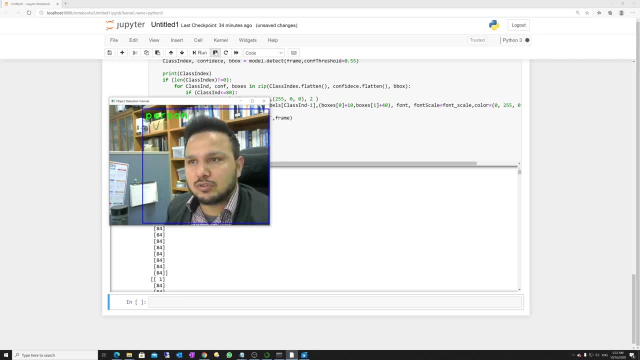 real-time. real-time webcam demo. thank you so much. thank you for watching this video. 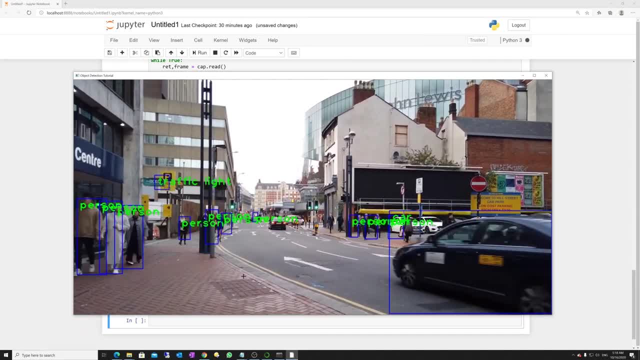 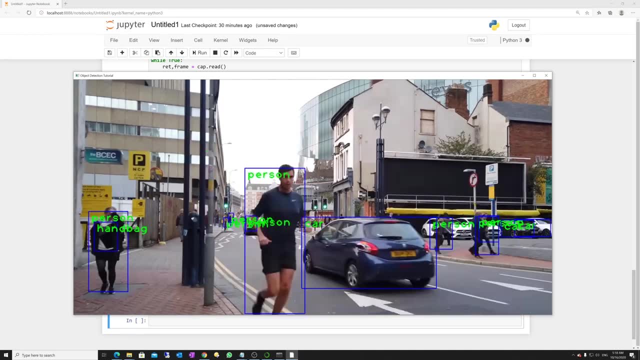 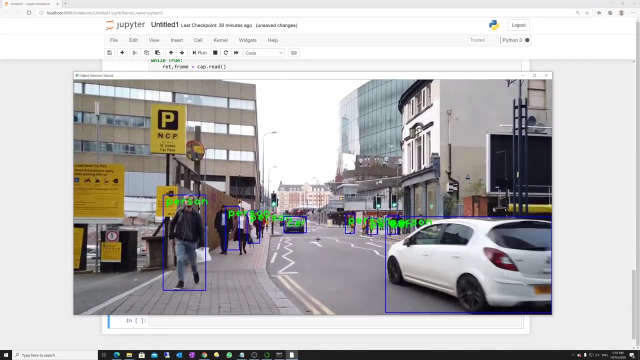 you see over here. this is the same video, this the same person, which who is coming right now. so over here you can see that in the start i showed you this video so as well. so it is detecting perfectly person, car and all others and it is uh, doing it like uh. 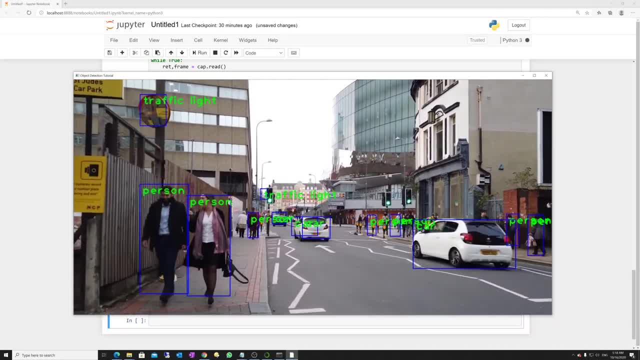 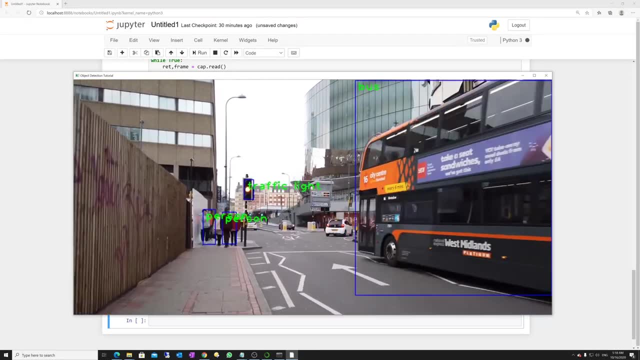 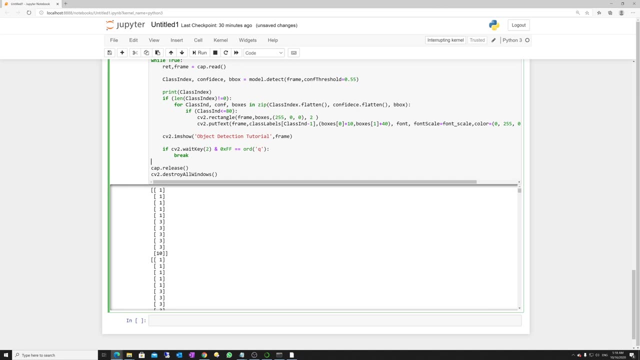 right. so we have a wild one, so it should not be wild one, but anyways, it is perfectly working, right. so the same code we just run so you can download it. you see that when the bus comes, it is detecting the bus and the car comes, it is it is detecting the car. so now it's time to have a webcam demo. 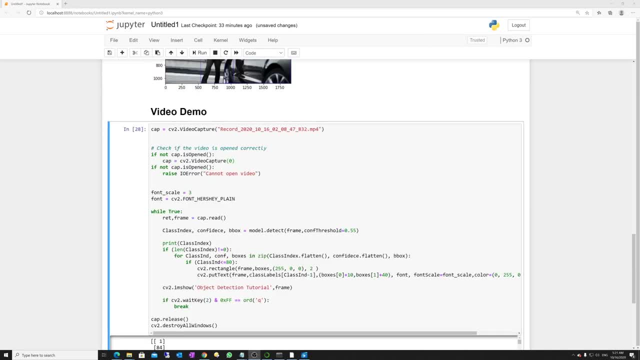 right in case to have a webcam demo, live webcam demo. it's better that you just, for example, you modify the previous code into one right. so in my case I have only one webcam. so based on the number of the webcams you have, so you can change this code. but it's dynamic: one right, the code is very. 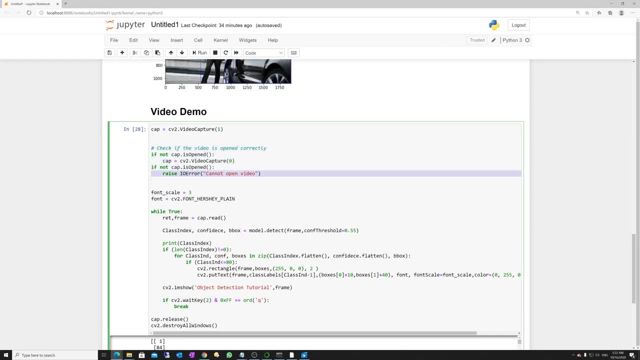 dynamic, so it is finding 0 or 1, and this is, for example. this is webcam, so all you need is just change it just. this is just my added instruction, so the most important one was that you need to change it to one right. so once you do. do. 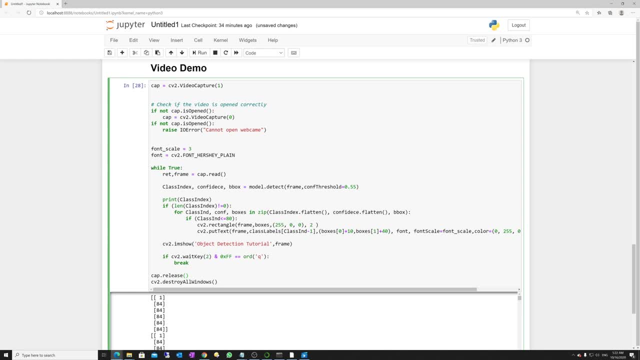 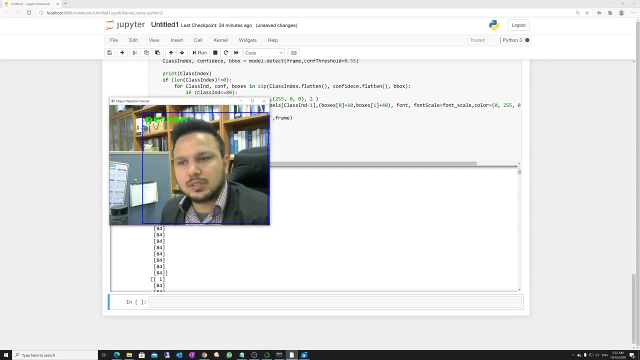 change to one. the rest of the code is same. if you execute it, you see it can successfully detect the person. and after move, you see if I move, so it can detect it as well. so it's real-time demo, in your case as you, that you might have. 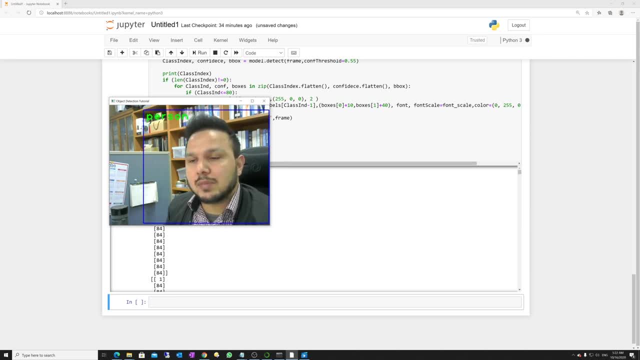 other objects as well. so you can just try it using multiple objects and you're using your webcam and you can just deploy real-time webcam demo. thank you so much. thank you for watching this video. 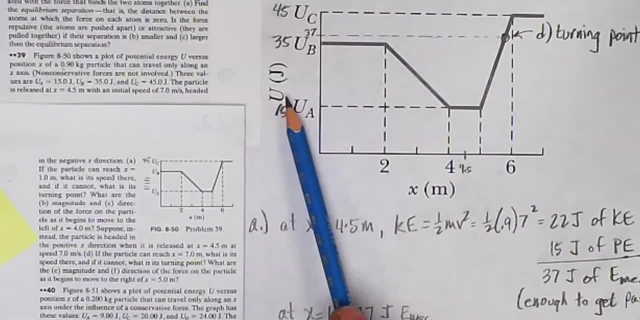 In this figure we have a plot of potential energy versus position, As a 0.9 kilogram particle that can only travel along an x-axis moves with no conservative forces involved. The values of UA are 15 joules, UB is 35 joules and UC is 45 joules. The particle is released.